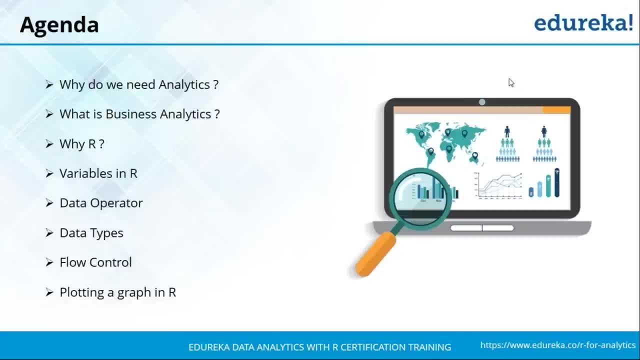 various types of graphs in R. So are we clear with today's agenda? Okay, so I've got a confirmation from Eric Shubham, Dave Roshni Gayathri, Reshma Pankaj. Okay, it's great to see that all of you guys are following. 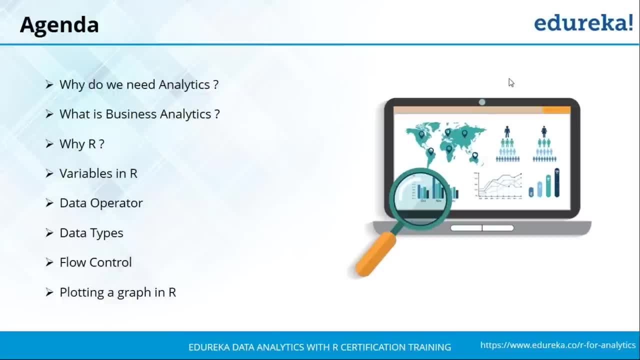 So I hope you guys are excited for the session as I am. So let's not waste any time and let's get started. So let's not waste any time and let's get started. So let's not waste any more time and let's move forward and look at the first topic for 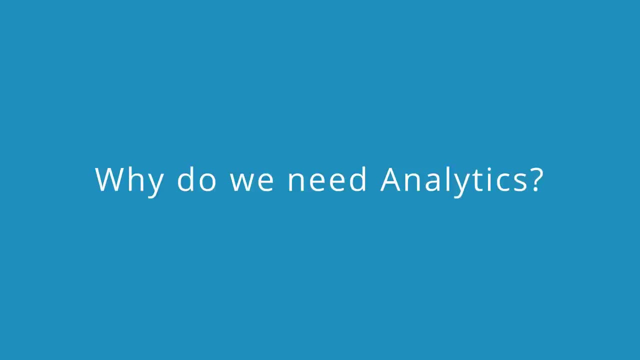 today's session. that is, why do we need analytics? Now, before we actually move into the content in the slides, I just want you to spend two minutes to have a thought and let me know why do you feel we need analytics? So the most common answer that I have got from you guys is that we use analytics to 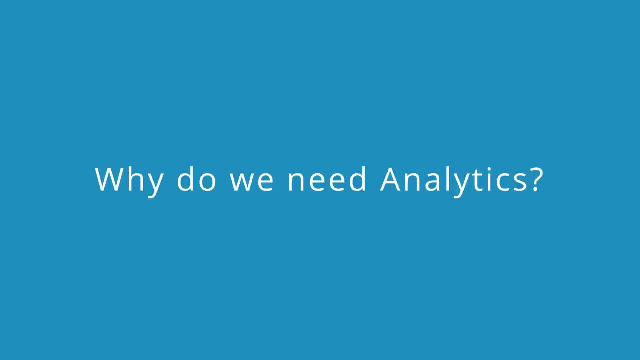 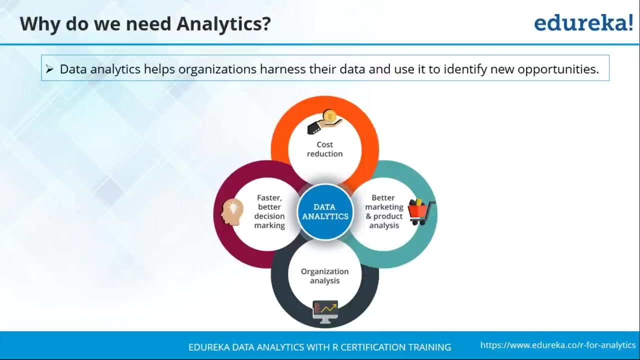 make better decisions. That's perfectly right, but analytics is not just used for making better decisions. There are many major things that analytics helps us achieve, So we'll mainly be discussing the need for analytics across four major points. Now, talking about the need for analytics in an organization, we can come across these. 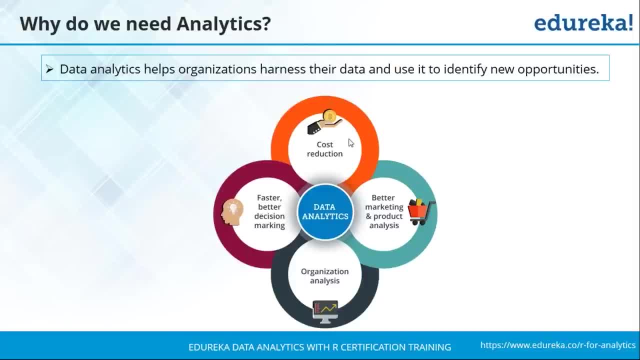 four points Now. the first point is cost reduction. Now every company invests a huge amount with respect to different resources that they take. It could be an investment on another company. it could be investment on the same company, across their employees. It could be with respect to certain marketing campaigns that they're running certain. 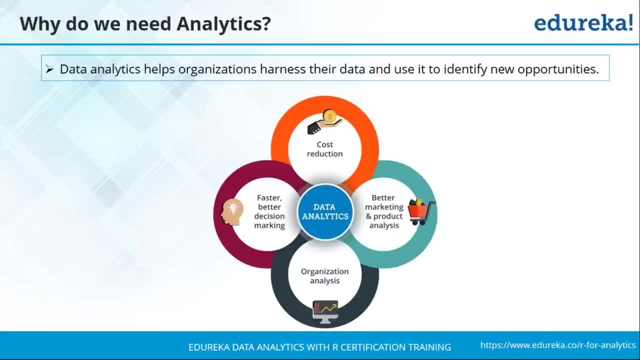 research they're putting into, but how do they know which is going to be successful and which needs more investment and where you need to cut short on? And that's exactly what analytics helps us achieve. Through analytics, we can identify which section is actually performing well. 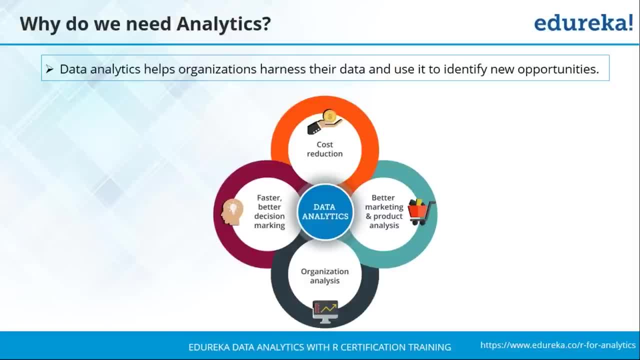 Now again, let's say you're investing maybe 50 million on three companies as such. So not all companies achieve the same level of performance and give you the same level of reward with respect to that, So you would definitely prefer to invest more in a company that is giving you more rewards. 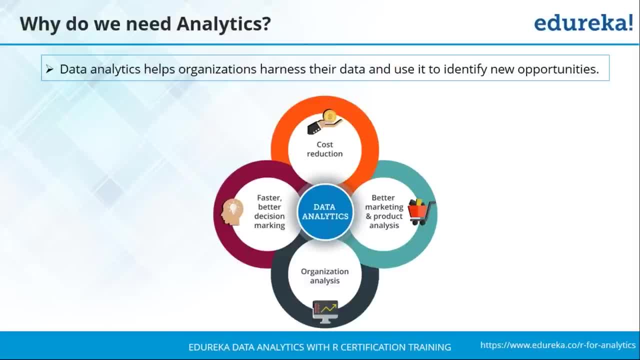 And to know that what you need to do is you need to analyze the performance of that company. Now, this is a big example. Let's take a smaller example. We end up spending money on a lot of unnecessary things over the month and at times we end. 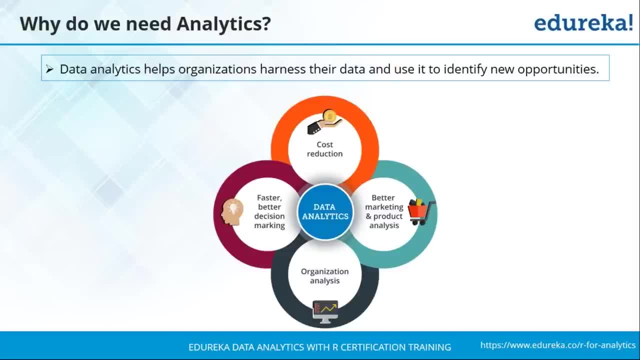 up short over the month. Now I personally have experienced this a lot of times, and here what we actually need is to analyze And reduce the cost expense that we take up on a regular basis. I personally had invested a lot of my money into fitness side. 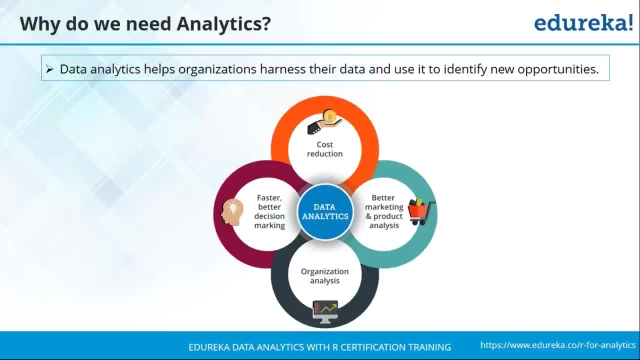 So finally, after some time, when I had checked how was I making the right decision investing there, I realized I was it. So, again, those are one of the key things that help you identify and make a better decisions with respect to that sale. No, Eric, I didn't stop going to the gym. 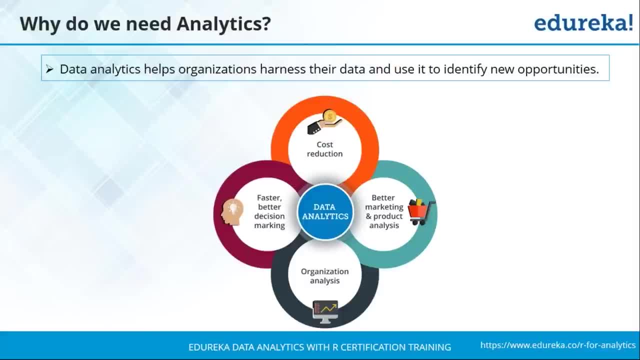 I just increased that and reduced a certain level of unnecessary investments. So, again, Those were decisions I had made after carefully analyzing my investments as well as my opportunities, Which in turn, also helped me reduce the cost that I was spending. So the next key part that I would be talking about is better marketing. 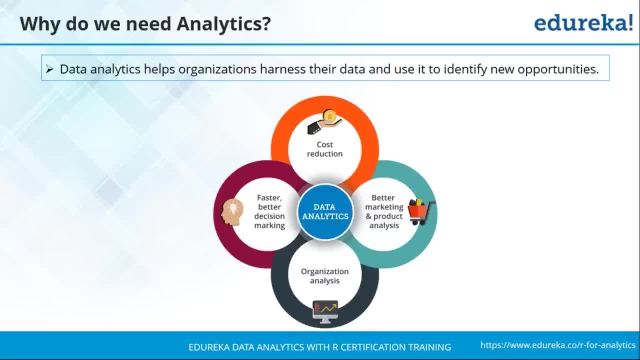 Okay, now again. it's always important to understand how the present market is and what is the public demand as well. Once you understand that, it becomes easier for you to market your product according to the requirements of the user, as well as create a better product that would meet the requirements. 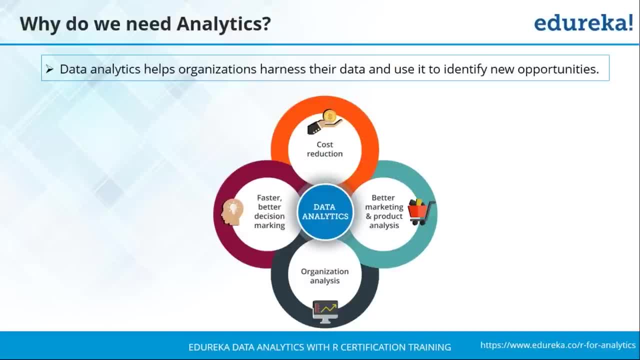 Now, if you have a good product by yourself, then almost everyone would definitely go for your product rather than any other product in that market. So this can be achieved through analysis. Similarly comes making better decisions with respect to your investments and marketing. Now, if I know how the market is, how the trend is, how things are working in the market, 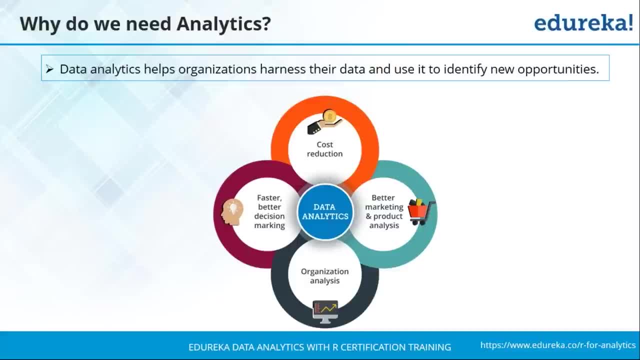 then it's easy for me to make a decision that could have normally taken a lot of time. This is basically because I've already analyzed- Okay, I've already analyzed- the market. I've already understood everything. I've understood the requirements, the needs and even tried out a few models where what 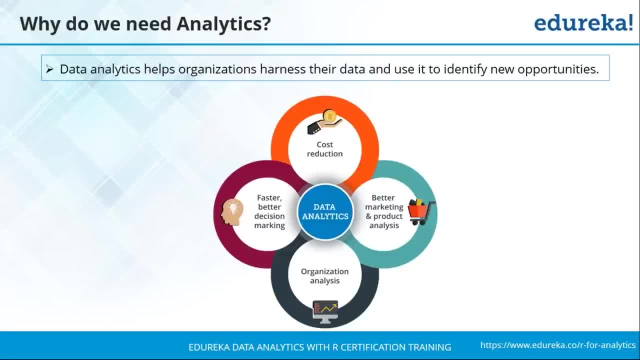 would happen if I had done this. I would have even tried out some scenarios with respect to that same. And once I've tried it, I've experimented all this, I've analyzed the complete result, then it's piece of cake for me to make a decision call there. 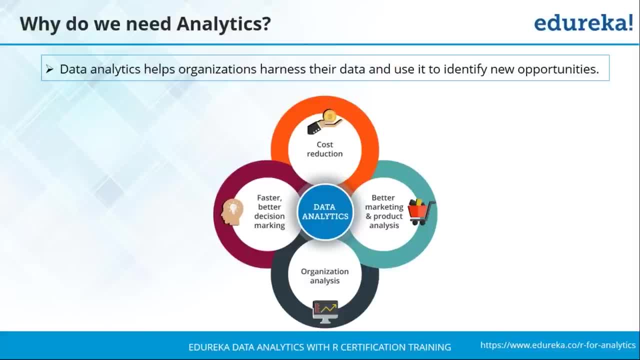 So it's quite fast when you compare to a rather risk taking situation where I have no idea how the market is. I'm not even bothered thinking of what is the requirements, but still, I'm just going with that flow. So data analytics definitely makes it easier for you to make better business decisions. 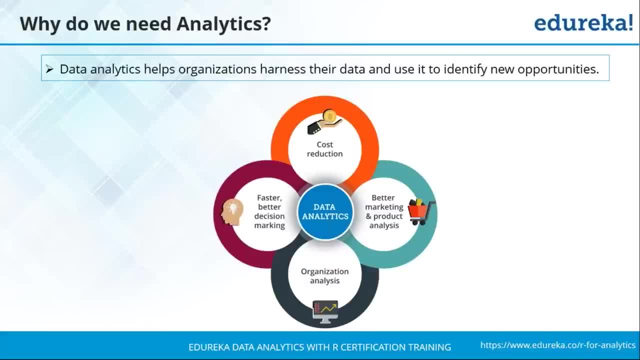 and better marketing policies. Finally comes organizational analysis. Now every company needs to understand where they are in the current race Now. to do that, one of the key factors is to help understand how they are performing themselves Now. organizational analysis helps them understand how they are performing as an individual, as 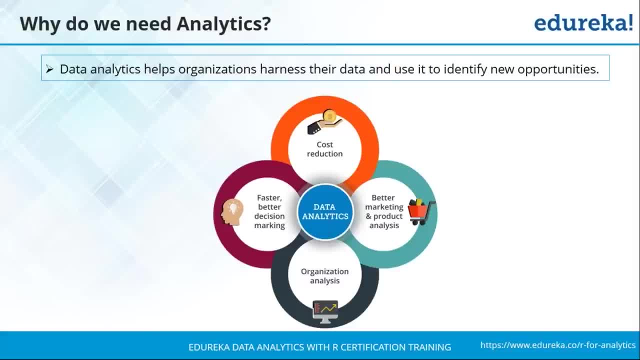 well as an organization as a whole. Now, we've all had our own data. We've all had our shares of reviews. there are quarterly reviews, there are yearly reviews. all that comes into picture and helps the organization understand better who's actually devoting more towards the organization and whom to take up up the chain with respect. 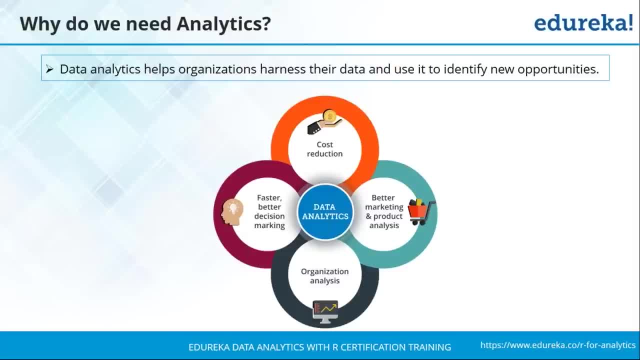 to that. Now we've definitely seen this on our day to day basis, because we've seen certain people who do perform extremely well being pulled up when compared to people who've got more experience as such. So always this analysis that is done within the organization helps you achieve better. 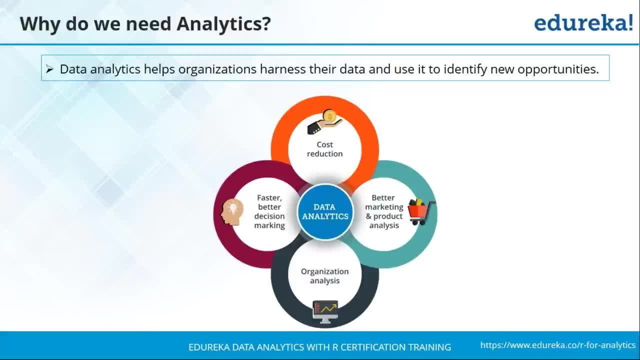 result as an organization as a whole. Now, with these four points, I hope you guys have got a simple understanding as to why we need analytics in an organization, as well as on our personal life aspect as well. Okay, so I've got a confirmation from Shubham Reshma, Eric Pankaj. 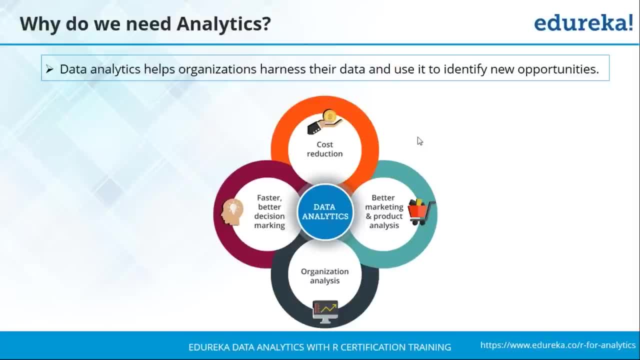 That's great to see guys. So again, please make sure at any point if you're not clear with any concepts, or if you have any doubts, Or even if there's something that you want me to repeat once again, You put it across in the chat box. 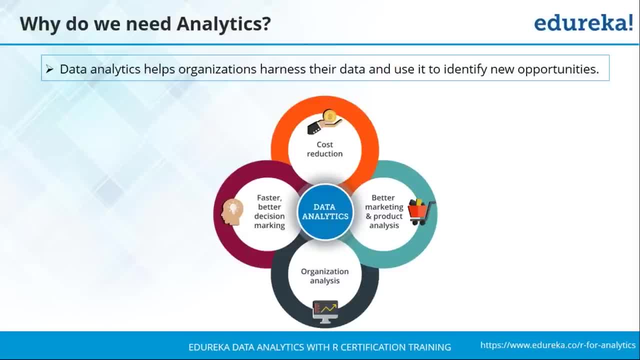 If I have to repeat a same concept 10 times, I have no problem, but I want to make sure that you guys are completely clear with respect to what we're discussing as part of today's session. Okay, Keeping that in mind, let's move forward and try to understand what exactly is business. 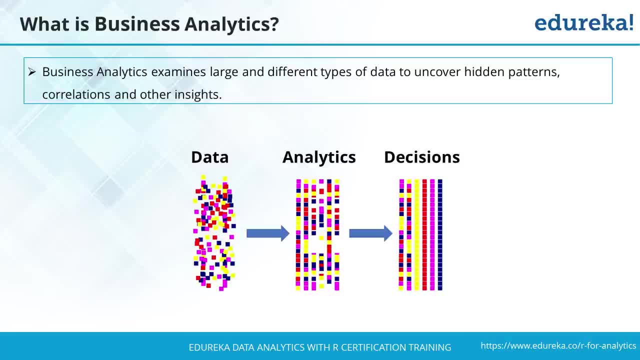 analytics. We've understood why we need it, but then comes the question on what exactly is business analytics Now? business analytics, basically, is the process of examining business analytics, Examining the large set of data that you have and achieving a hidden pattern or correlation. 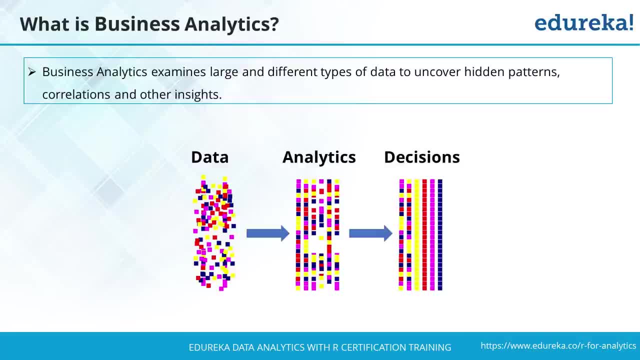 between that, or even a better insight as to what you need to do. It basically helps you understand with all the data that you have gathered. This could be your organizational data, It could be the market research, It could be your product research. Once you've completely analyzed all these data, then you could find something that you 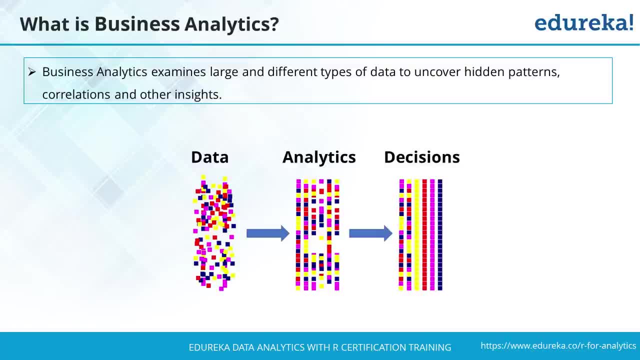 are lacking on. Once you've identified this, then it becomes quite easy for you to make better decisions, better products, better marketing strategies and so forth. Now again, if you look at the image here below, this is exactly how your data is at. 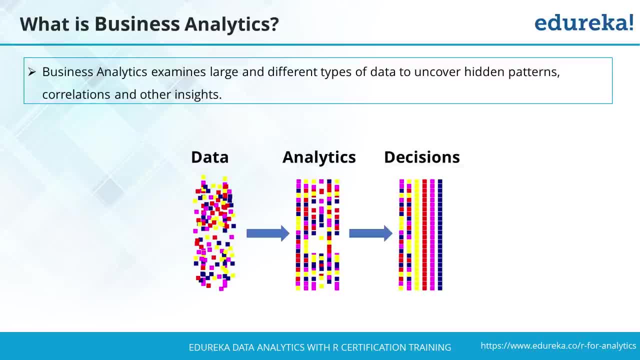 moment, It's a scattered mess. Okay, You've got everything that you want present in your data, but to find anything specific becomes a problematic, And to understand how you're doing is an even bigger mess. So to achieve all that, you need to use analysis. 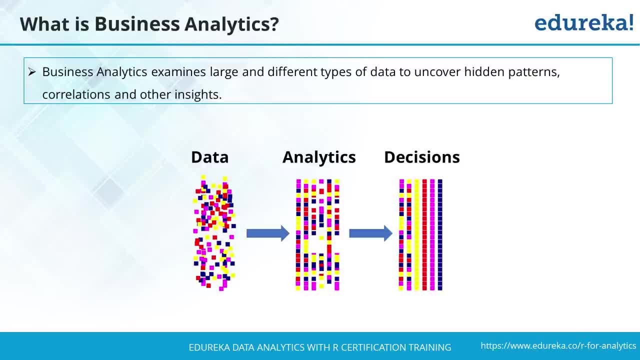 Through the analysis process, it becomes easy for you to make a correlation and a structure of data that you have, so that it becomes easy for you to go ahead and make the better decision Now. analytics is not the complete solution as such, and it helps you understand how you're. 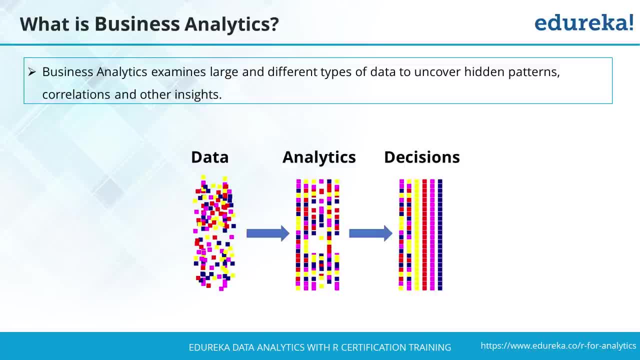 exactly doing at the moment with respect to what you have already tried out as well. So once you have established the path for you to move ahead, it becomes quite easy for you to make a decision on which path you want to go, follow and which path will take you. 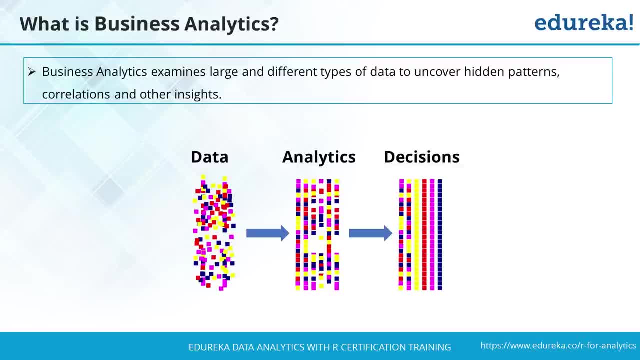 for the betterment of your organization. So clearly here. Okay, Now the result of this analysis that you've performed may not be something that could be always understood by someone who's not from an analytical background, And this at times becomes a hindrance, because you can't expect the people in the chain above. 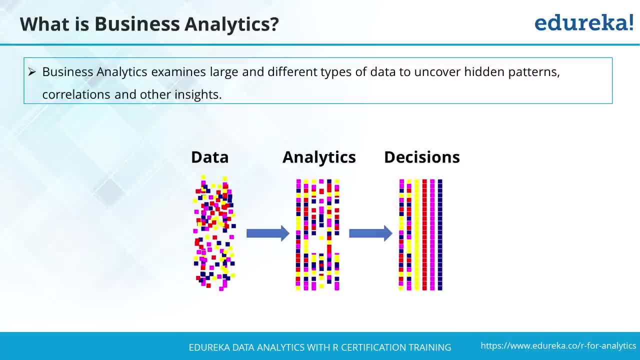 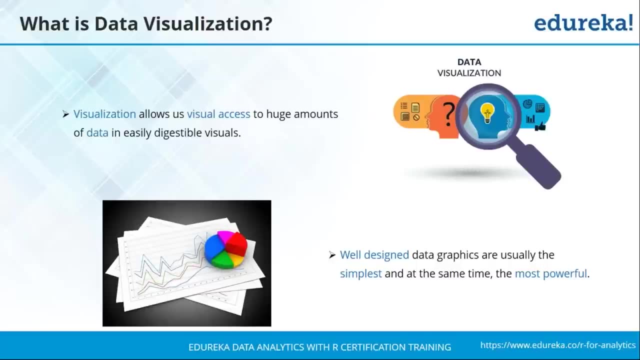 to always understand the raw data that you're providing them after analytics. So to overcome this gap, we have a concept of data visualization. But what exactly is data visualization? Data visualization, Basically, is a visual access to the huge amount of data that you have generated after. 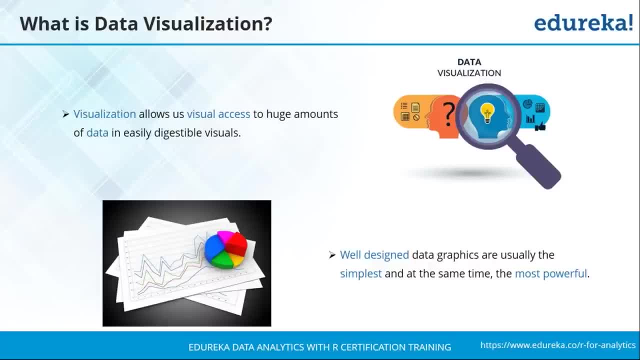 analytics. Now again, when you talk about why we need to use data analytics, it's a quite straightforward and a simple understanding that the human mind processes visual images and visual graphics more better than compared to raw data. as such, It's always easy for us to understand a pie chart or a bar graph better when compared. 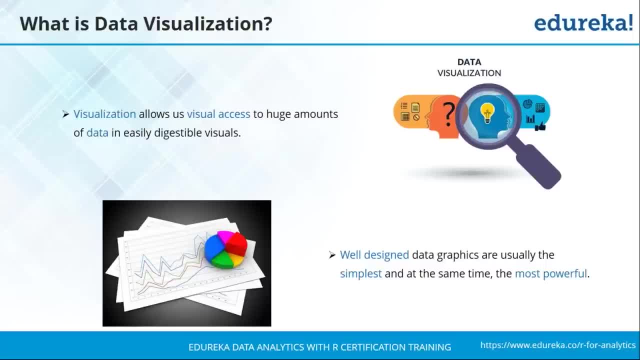 to the raw numbers that you would be providing me, And this is something that's common for anyone, Because this is how our human minds have been set. Now you may be wondering: how can you achieve data visualization from the data that you have already analyzed? 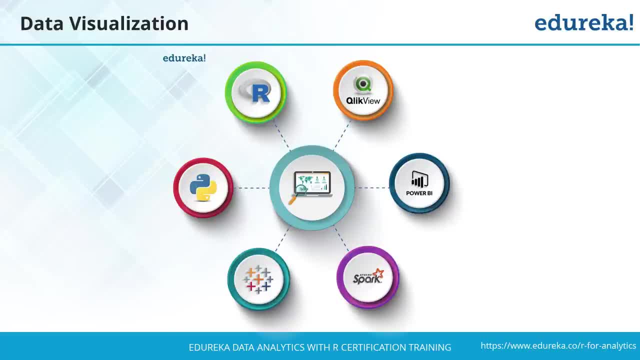 Now to do that. there are major tools in the market at present. These are some of the major players in the market at best Now here you have Tableau, ClickView R, as well as Pentaho BI, and you can see a lot. 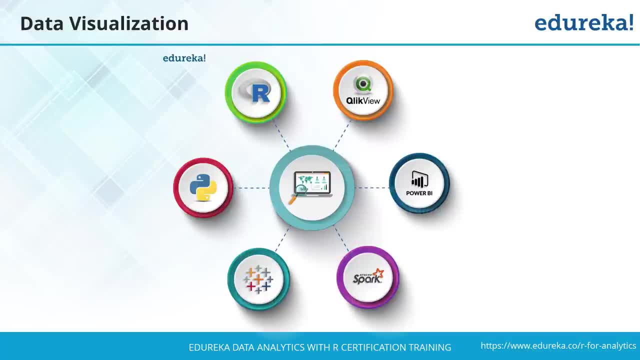 of other tools as well. Now, these are some of the major tools. Now again, when you look at Tableau and ClickView, those are tools that are completely different And you can see that they are very similar. They are completely dedicated to data visualization itself. okay, 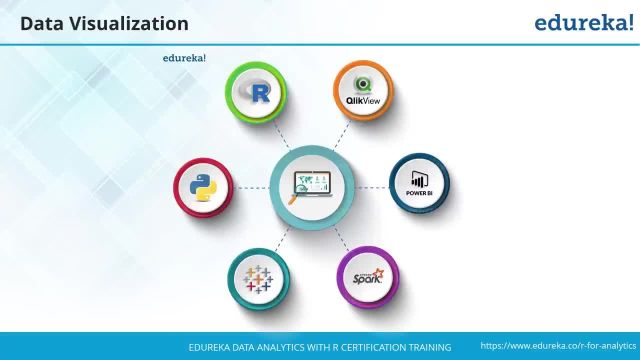 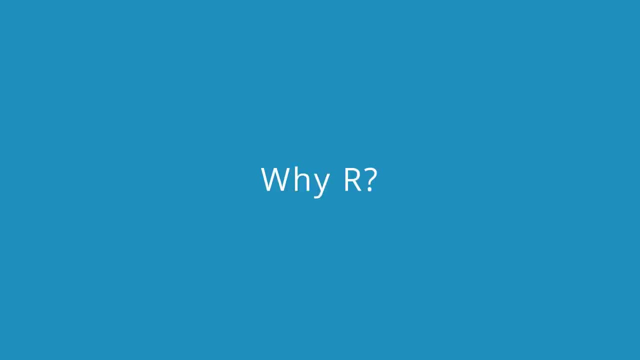 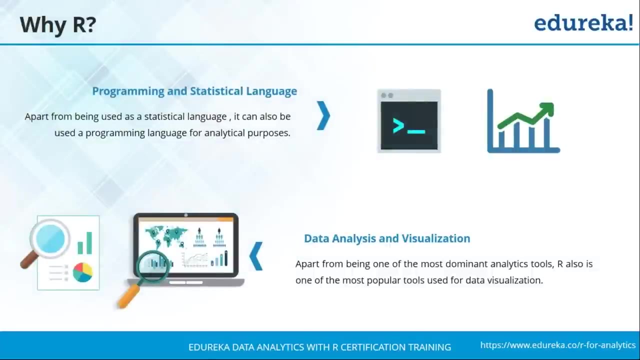 But then again, you all must be wondering: when there are already these tools that help you achieve data visualization and certain amount of analytics, why go with R? And that's exactly what I'll be explaining Now when we talk about why R with respect to other tools in the market, one of the two. 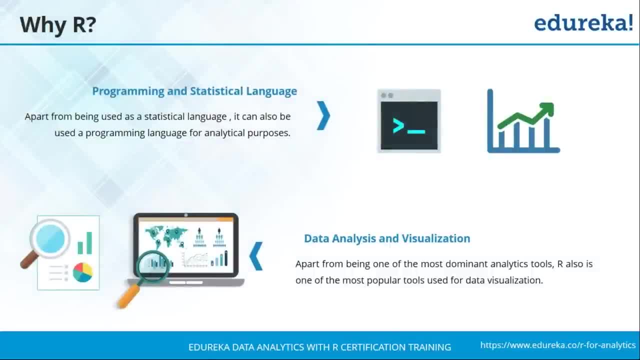 major points that I would definitely like to bring out. first. itself is: R is both a programming language and a statistical language as such. Now I'm going to talk about R. I'm quite sure that some of you would have at least heard that R is hard and is not one. 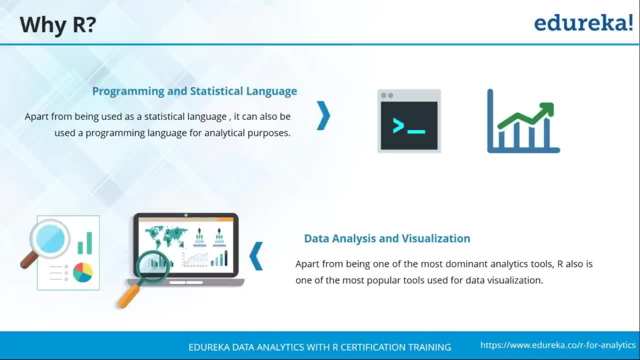 of the easiest subjects that you can pick up. But trust me, with respect to R's capability as a programming language and a statistical language, it is the best in the market. okay, And when you look at how easy it is to code in R, then you'll definitely realize how things. 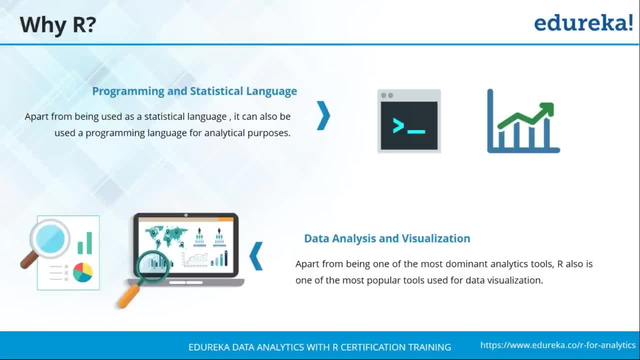 are. Apart from that, R can be used for both data analysis as well as visualization. Now, if you look at some of the other tools that we had seen in Tableau and ClickView, as seen in the previous slide, they are tools that are specific to achieving either data. 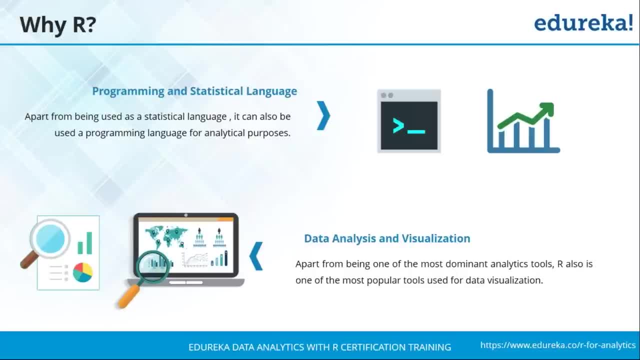 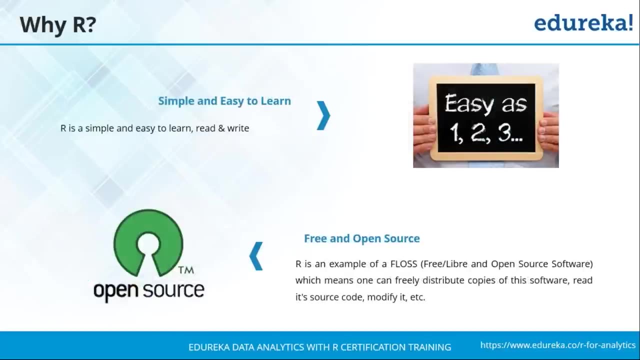 analytics or data visualization specific, But with R you can achieve both analysis as well as data visualization in a single tool itself. So here again, it becomes a tool for multipurpose. Now, apart from this, R is one of the simplest languages to learn, as I had mentioned earlier. 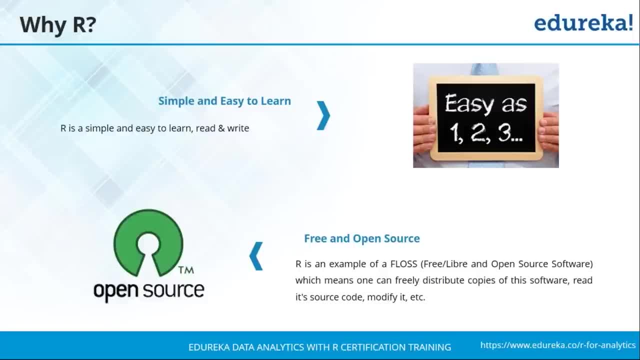 Now R is quite close to the English language. Therefore, writing codes in R is a piece of cake. Okay, In today's session we will be trying out a lot of codes as we're going into R, So at the end of the session you will completely be able to understand how easy it is to learn. 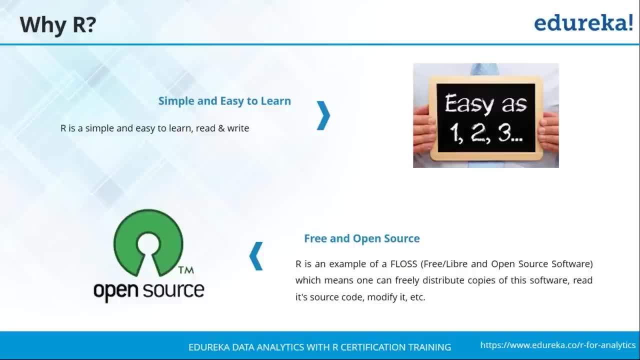 and how simple R is for performing various operations. Now, one of the key reasons as to why R is so popular is because it's a free and open source product. Now again, when you talk about free and open source product, it basically means that anyone 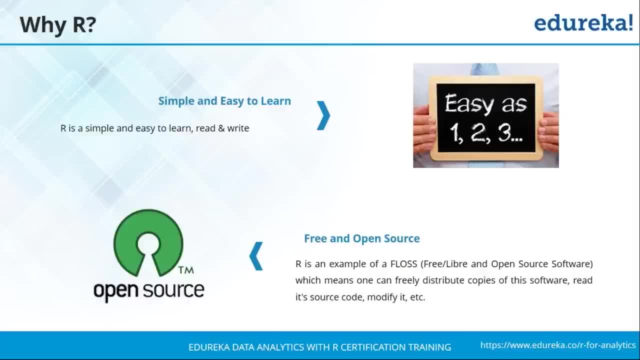 can download it, Anyone can modify the original source code of it And anyone can fix it, And anyone can feel free to redistribute this code as well. So R lets you completely play around with its source code itself. So if someone is actually doing that with their product source codes, then you can completely. 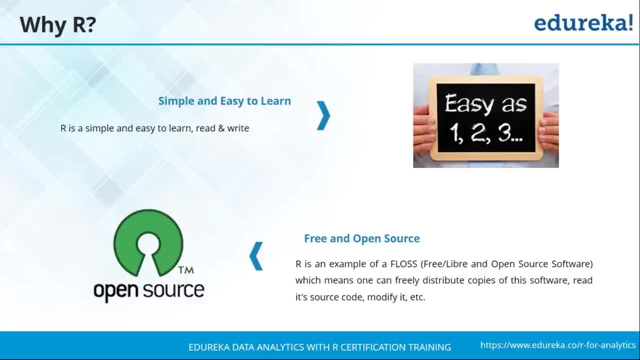 understand how popular, how open and how big the community is with respect to that tool. Now R has a very huge community comprising of both programmers and analysts, So here you can find both flavors and everyone is quite friendly and helpful. So at any point, if you have certain queries, 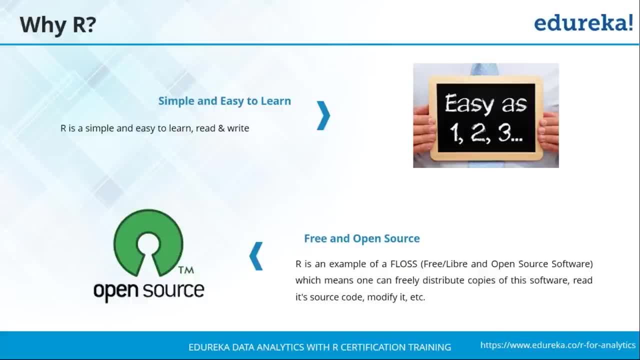 Along the line in your career using R. feel free to reach the R community and you can definitely find someone who will be able to assist you. So any questions still here about what is data analytics, what is data visualization and why R exactly. 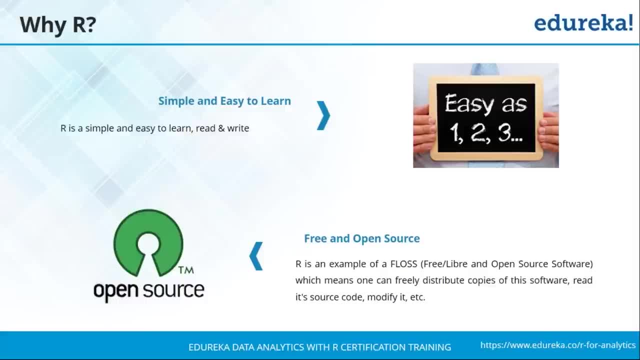 Okay, Pankaj is asking me: how is R better than Tableau? So, Pankaj, again here, when you see, definitely, I would say, Tableau helps you achieve better visual graphics, But for Tableau you need to always feed in and analyze data sets. 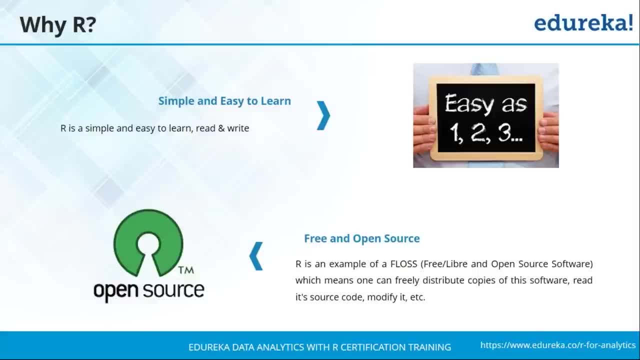 Okay, So there, once you have your analyzed data set, then it is. you can perform certain operations like filtering out or selecting certain amount of data, But through R you can actually completely perform the process of analysis and then, and there itself, you can achieve your data visualization. 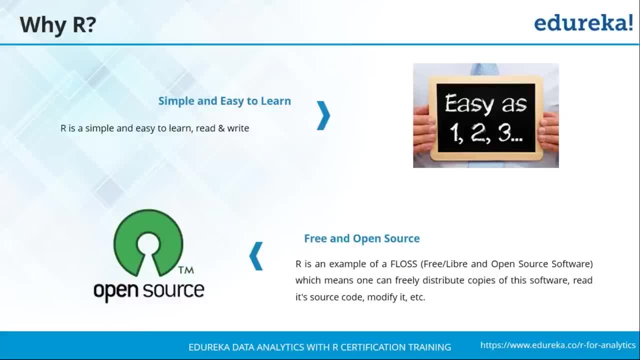 You don't need to depend on any other tool for achieving data visualization with respect to the data that you have achieved through analysis. So basically, you're reducing the need for another tool itself. Is that clear, Pankaj? Okay, So with this, it's time we begin deep diving into R, And the first thing that you guys 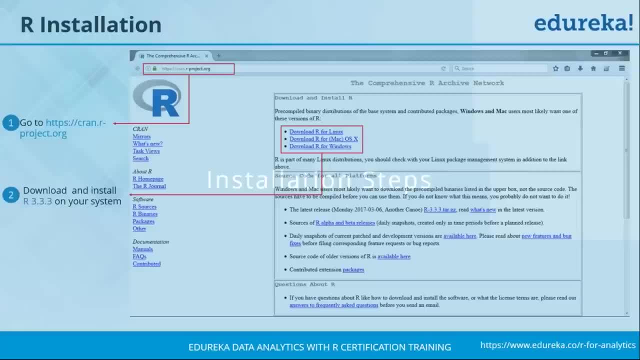 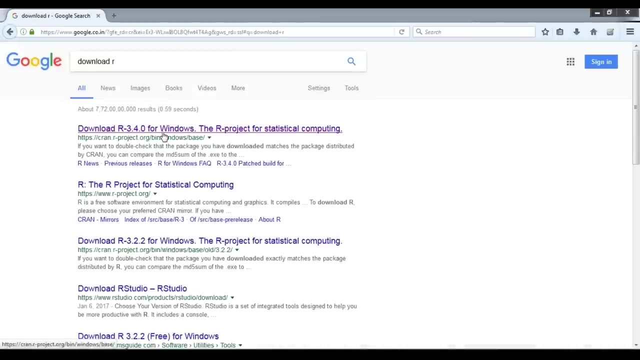 need to do is install R on your system. Okay, To do that, all you need to do is go to the official site of R, that is, cramr-productorg. Let me just show you that, So you can just open your browser and search for download R And you get the first link. 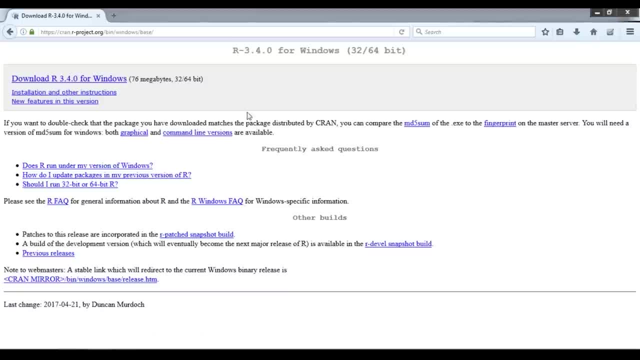 Now the first link is for Windows. for those who are working with Windows can directly click on this And go to click on download option. Okay, For those of you who are working with different operating systems, like Mac or Linux, you just need to go to their home page. 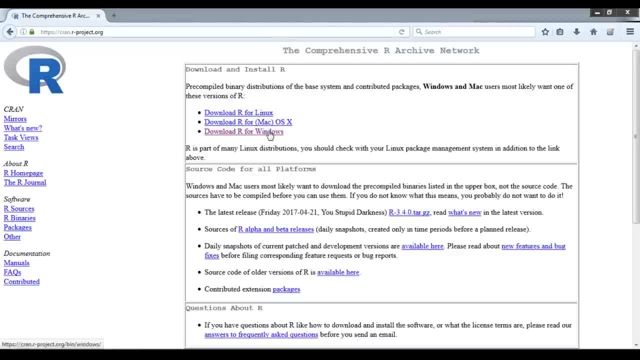 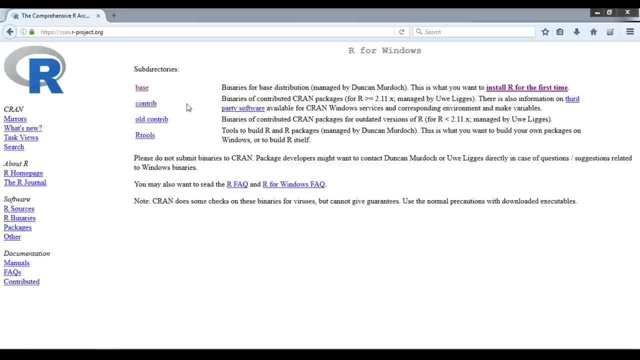 And here you have the option for Mac and Linux, Again inside Windows. you need to always ensure that you're downloading the base option, because that's exactly what you need as part of this session. So once you've gone ahead and downloaded this, an exe file would be downloaded. 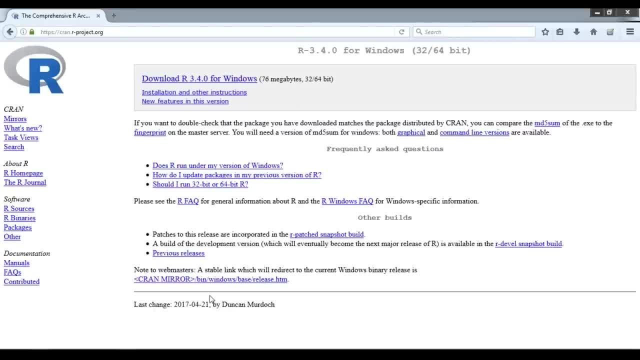 So again, if you click on basically redirects you to the first page that we had come in. So just click on download for Windows And you can see the exe file for downloading. So just save it Now. I've already installed it on my system. 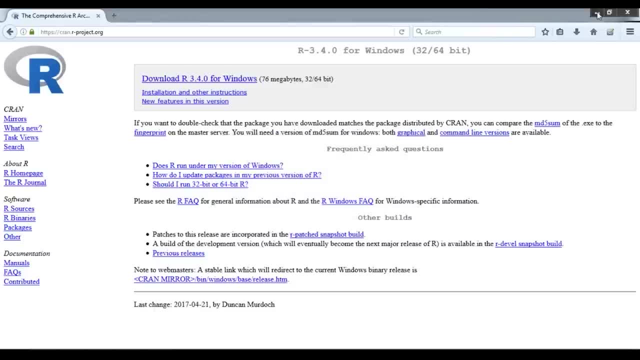 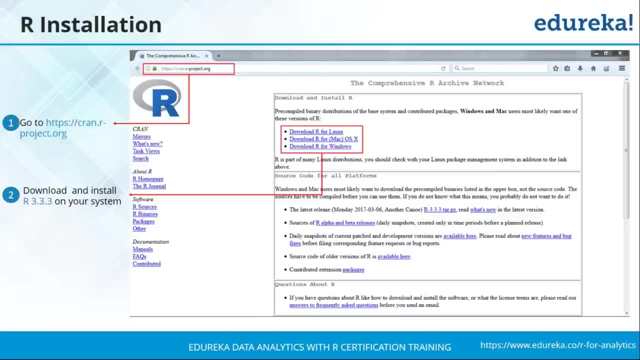 So you guys can download it and go ahead with the installation step. It's quite easy. It's all you need to do is just keep clicking on next. So please go ahead and install And if any of you are facing any troubles, please let me know. 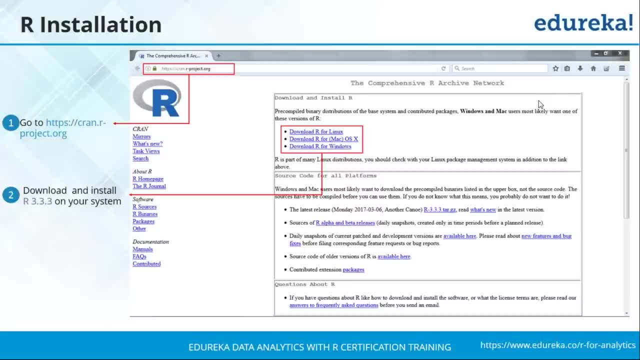 So that I'll be able to assist you. Okay, So it seems like all of you successfully installed R on your system. Now you can directly begin by coding in R, But what I would recommend is you go ahead and install. 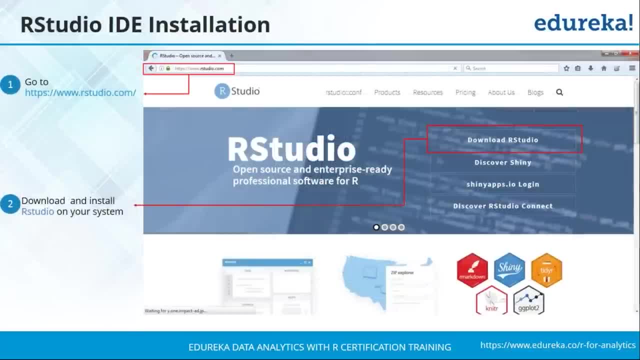 The RStudio IDE. Now, the purpose of an IDE is basically to make it easier for you to program and, as beginners, I definitely recommend that you begin with downloading and installing the RStudio IDE itself. So, again with respect to the purpose of downloading and installing, an IDE is basically 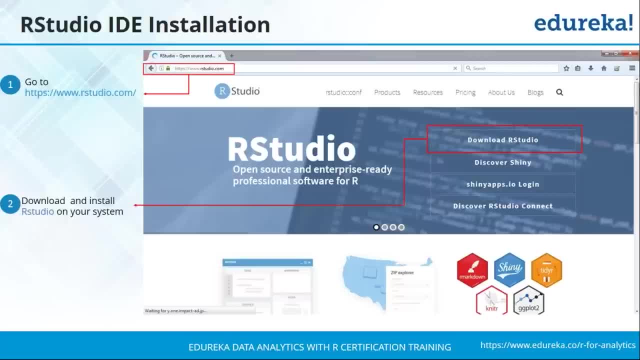 to have a common environment for working with respect to your data and as well as becomes easy for you to learn about the various possibilities and understand about your mistakes in an IDE, better You can go ahead to RStudio's website. Let me just show you. 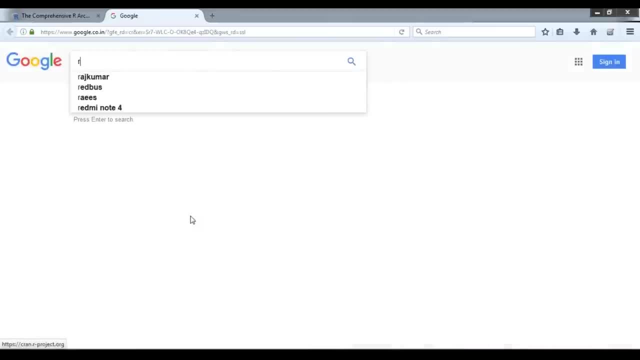 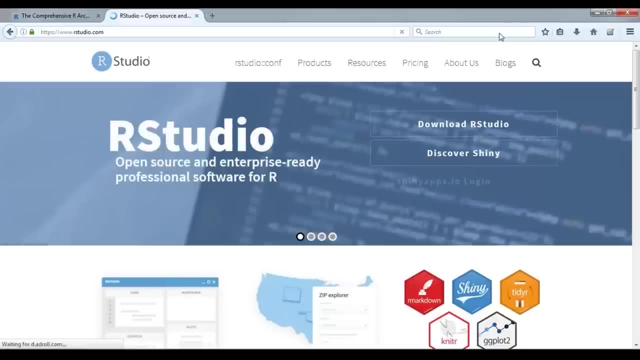 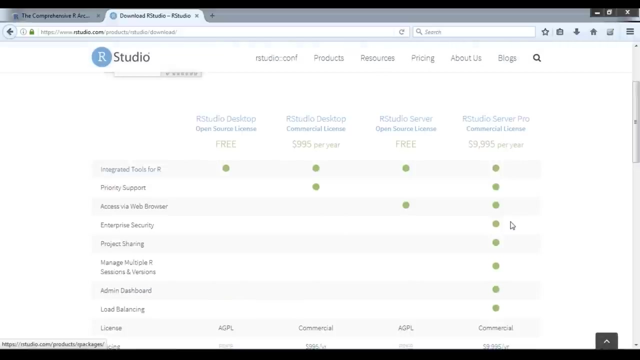 You need to search for RStudio download. So let me just show you the home page for RStudio. So this is the home page for RStudio and you just need to click on download RStudio option. So here you can see different versions of R that are available. 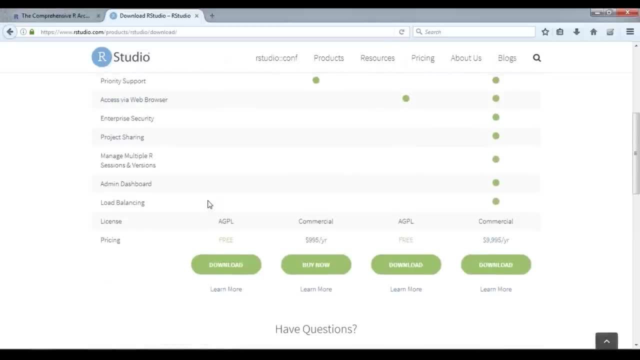 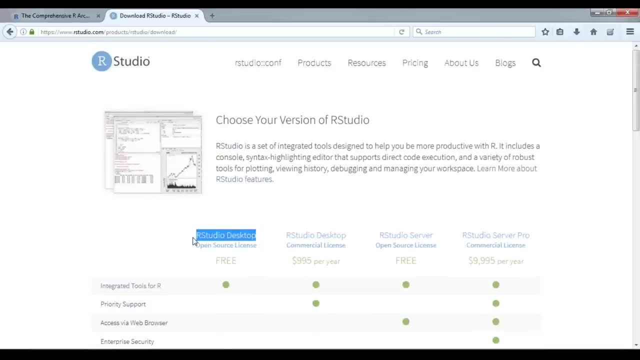 So I would recommend that you download the R desktop version here Now. apart from having a free version, they do have a paid version. But again, I would recommend that you go ahead and download the R desktop free version from this page. 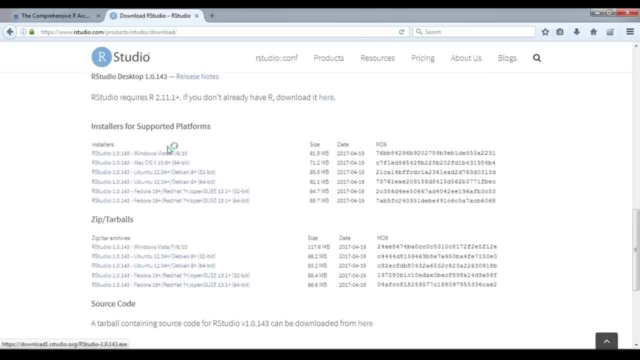 So if you click on download, you can see the various options with respect to each operating system. So again, choose the version that suits your operating system, Just download it and then again the installation is quite straightforward. You just need to keep clicking on next. 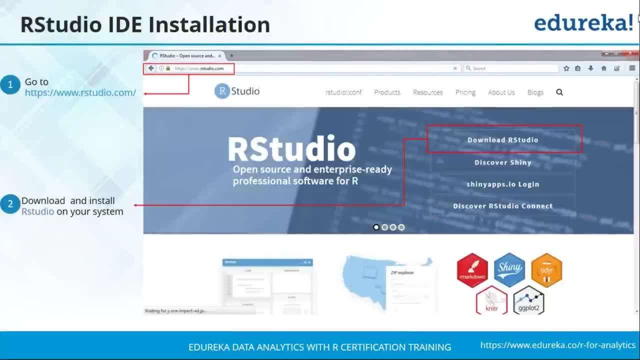 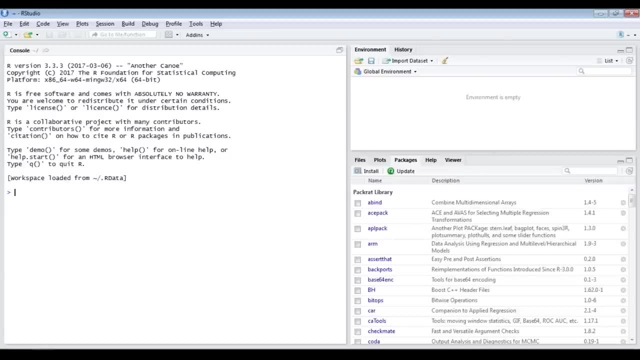 So if any of you are facing any troubles, let me know and then I'll be able to assist you with respect to that same. Okay, So now that all of you installed RStudio on your system, so this is basically how your 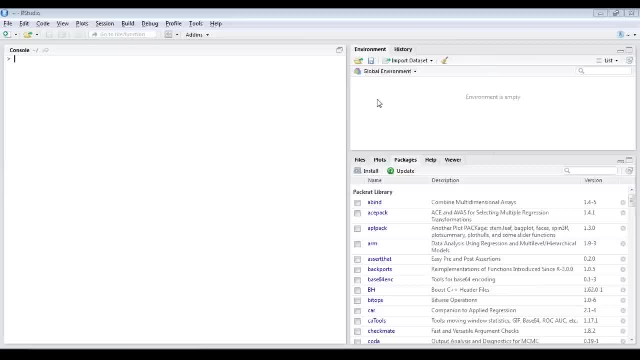 RStudio looks like. So to your left you have your console, to your right you have your environment window and finally you have one of the most important window, that is, your workspace window. Now, here, basically, you have multiple tabs here. Now again files that you want to work around with, you have your plot. so basically any. 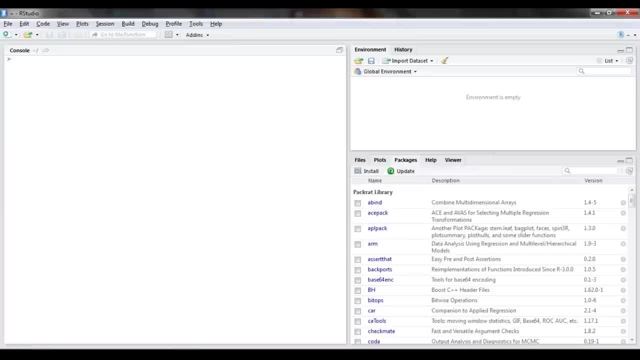 graph that you're plotting can be seen here, and then you have your packages tab. So these are very important options. So let's say you want to install a specific package for your RStudio. All you need to do is click on the install button here, and then you can select whichever. 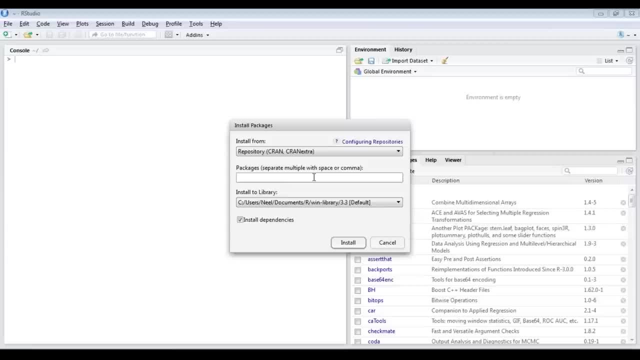 package that you want. Let's say, I want to install a package called ggplot2.. So again, I just have to type ggplot2, select it from here and then just click on install. So basically what happens is R actually checks with its libraries and then it goes ahead. 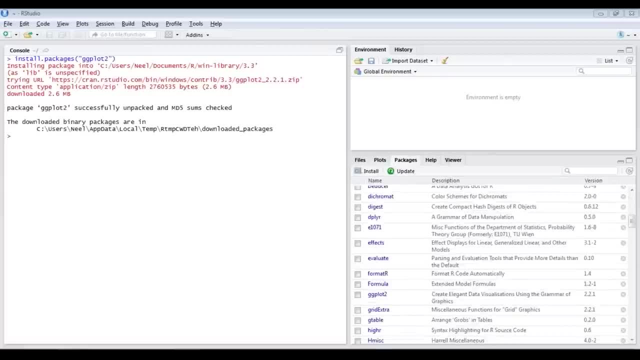 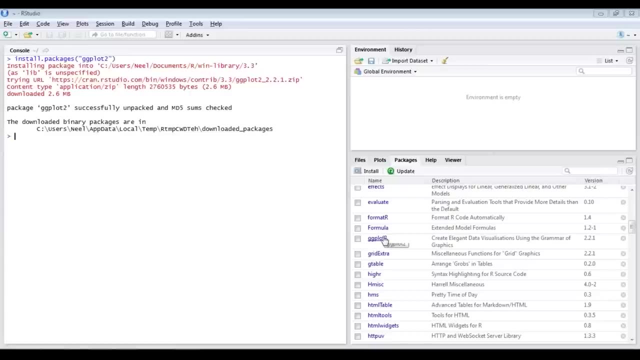 downloads the package and installs it as part of my RStudio. So once downloaded, you can find it here. So any package you want to understand what exactly it does or how it works around, all you need to do is just click on the package name and then here you can find the complete. 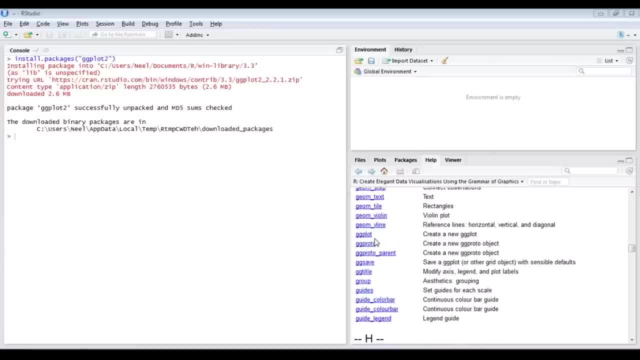 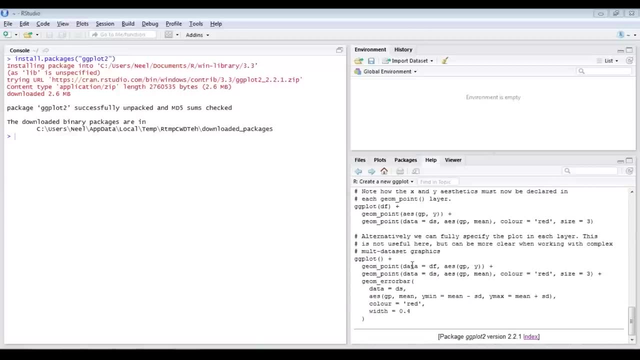 help page for that package. So here, let's say, if you go to ggplot, then you can find the description, the usage, the argument it takes, the details and so forth. So this is a package basically used for graphical representation. 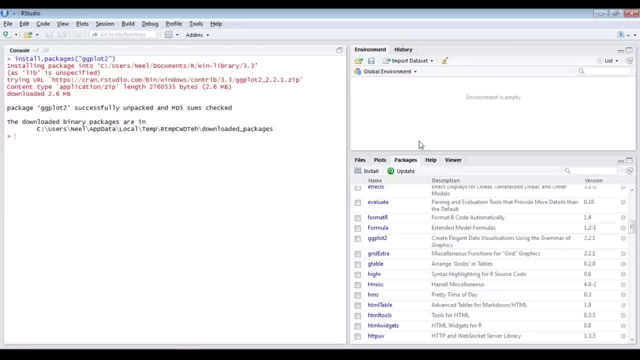 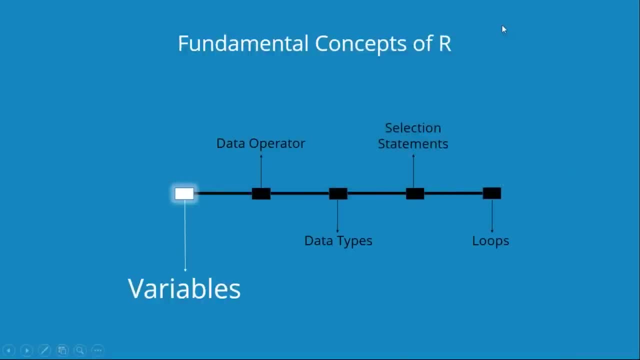 So I hope you guys have got a simple understanding on working with the RStudio. So now let's go back to our presentation and begin by deep diving into R. Now, the first topic that we'll be discussing as part of the fundamental concepts of R is a variable. 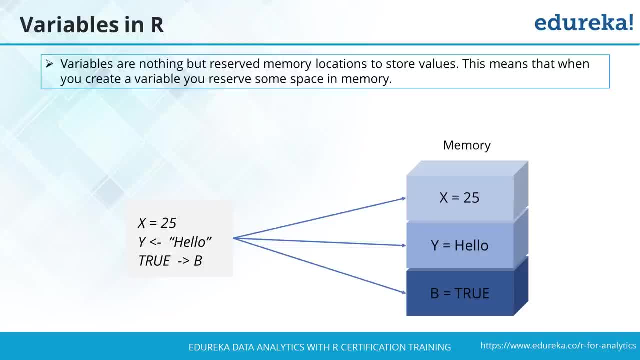 Now, a variable, basically, is nothing more than a reserved memory location used to store certain values, which again, in turn, means, let's say, if you're working with a value, then that value needs to be stored in that memory, and to store it in a memory you're going to be. 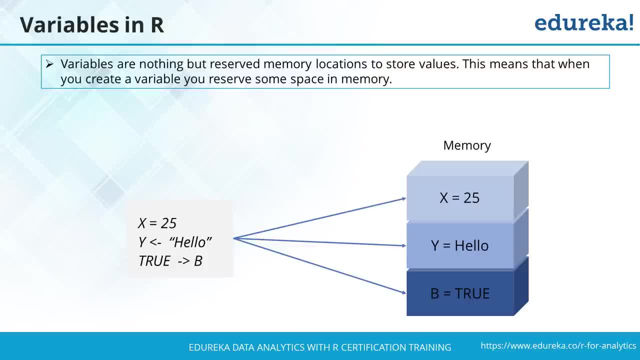 creating a variable. So it's a very straightforward, simple definition. Now there are three ways you can actually create a variable in R. Okay, if you look at the image here, Now again, I can directly write the variable name equal to the value. 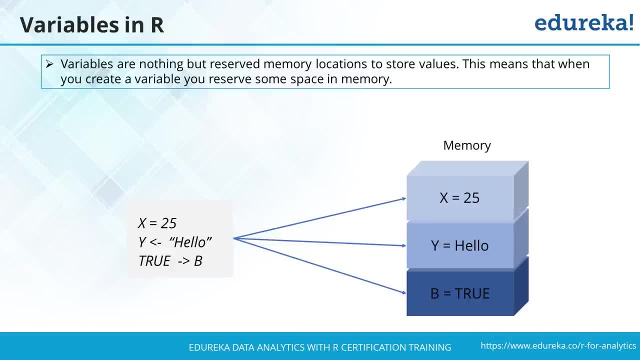 Or the variable name, a less than symbol, followed by a hyphen and equal to the value, Or even the value hyphen greater than symbol and the name of that variable. So these are again the three ways you can declare a variable in R, but again in turn. 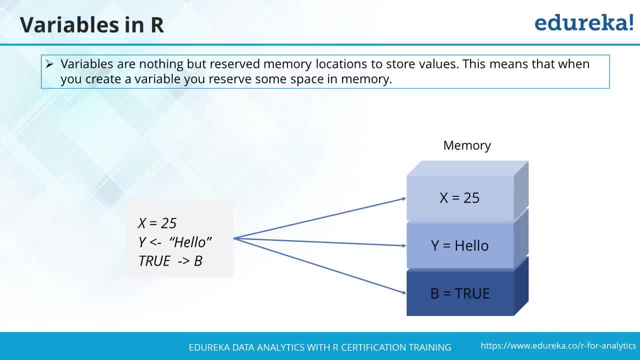 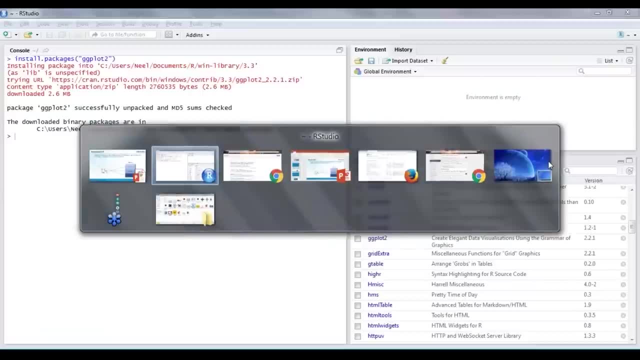 all of them have the same meaning in the memory location as such. Okay, so again, let me just show you how you can declare a variable in R and how it actually works out in the RStudio. So let's go back to our RStudio. 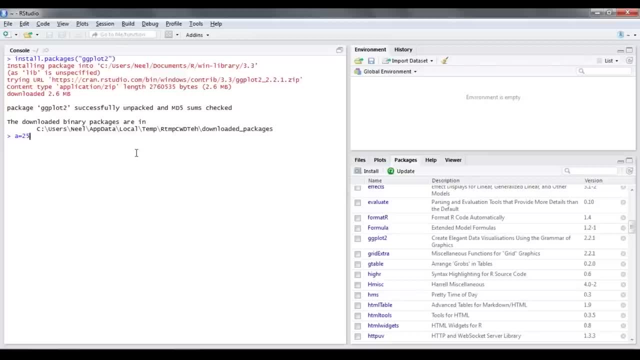 I'm going to say my A equal to 25.. Okay, So automatically when I type this, I want you to observe the environment window When I give enter. automatically a new entry has been pushed into the environment variable saying that the variable A, of numeric type okay, which is occupying 48 bytes, has the 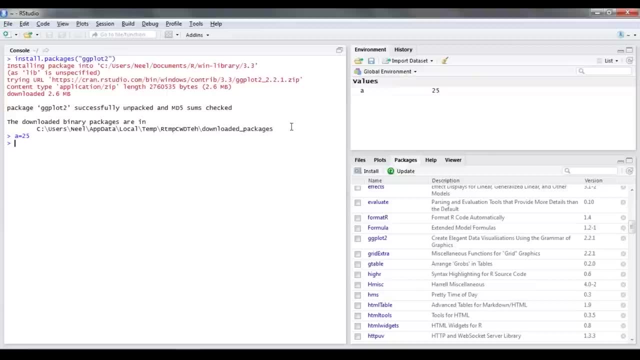 value of 25.. So this is something automatically done. Same way, let me say B and I'll just give a string value. So let's say: hi, how are you today? Okay, So this is a complete statement. When I give enter, you can see here the value has a new variable has been created called. 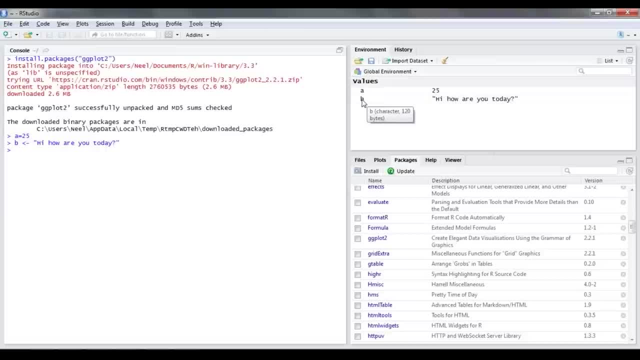 B. The value also has been set and you can see the memory location allocated to it. It's a character type and it's occupying 120 bytes, So apart from this, you can also work with Boolean value. Let's say true or let's say false. 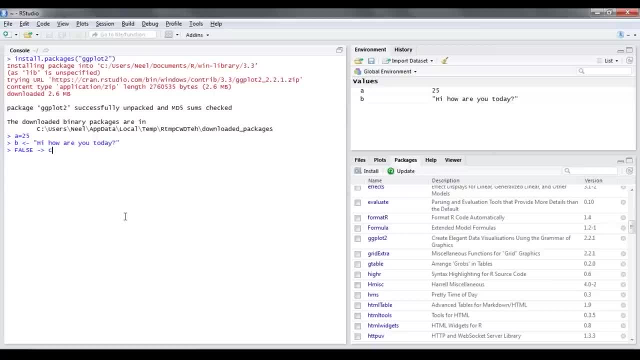 So I'll give it to value C, Variable C: Okay And enter. So here you can see. I've declared three variables, but again the way I have declared them is slightly different, but the end result for all three of them is the same. 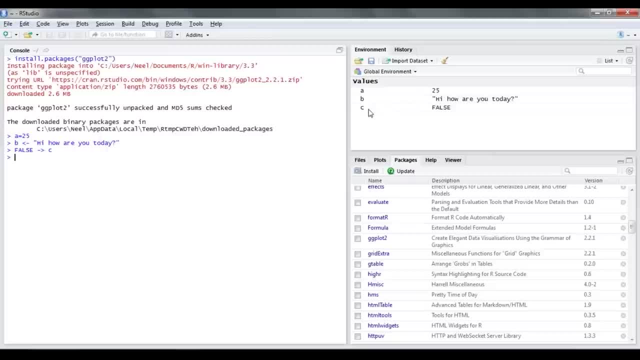 So again, a new variable is being created and the value has been assigned. So here, if you look at C, basically it's a logical type and 48 bytes have been allocated for it. Okay, So please go ahead and try these things. 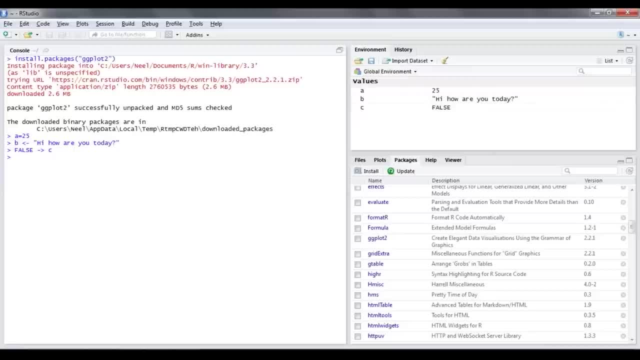 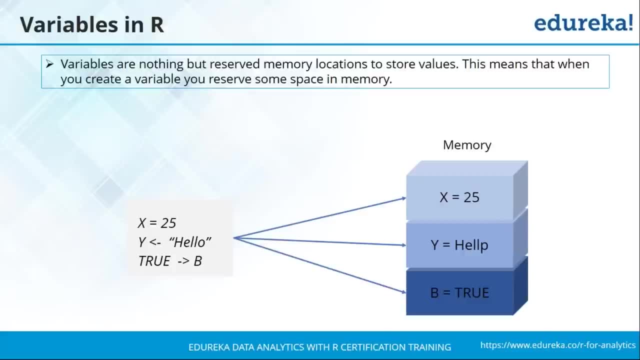 Okay, I know it's a very small thing, but again, it's quite important to understand what is a variable and how to work around with variables When you're working in R2.. Okay, Now, one key thing with respect to R, while you're in comparison to other programming. 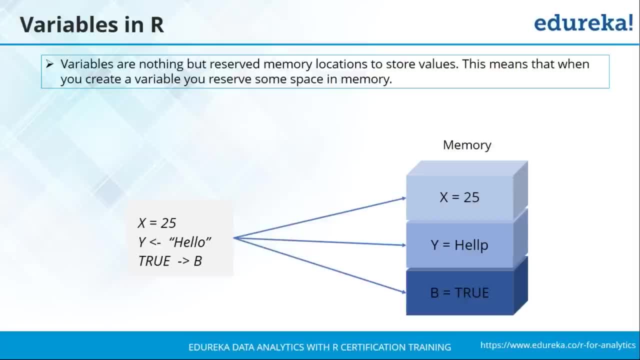 languages is that you don't need to actually define a data type for atomic data types. Again, what exactly is an atomic data type? we'll be seeing later, but to give you a simple understanding: your integer, your numerical value, your logical value, your strings. 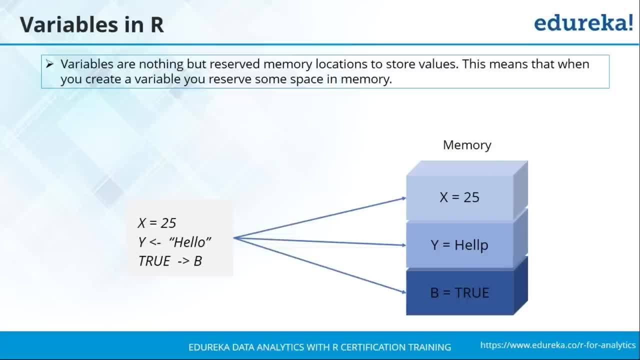 So all these don't need to have a data type defined while you're creating them. Again, it's a quite easy and straightforward language. Now, this is something that you would have seen while you were working with Python, if any of you. 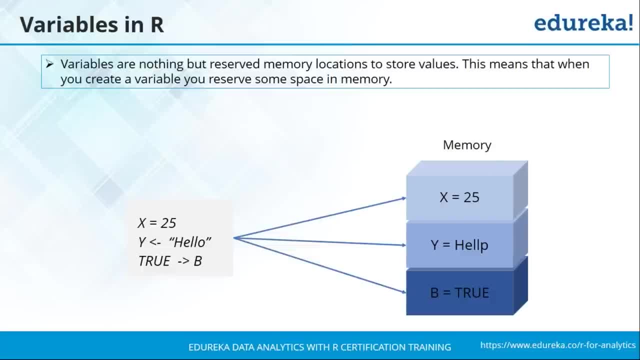 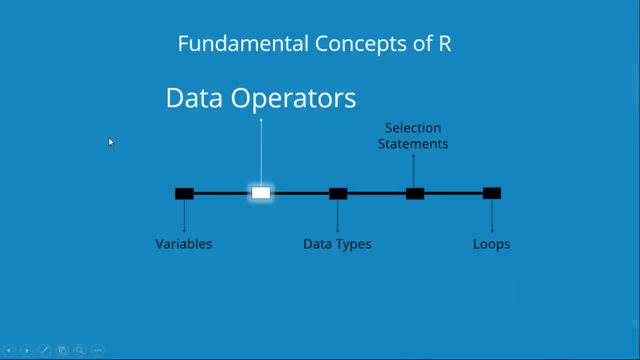 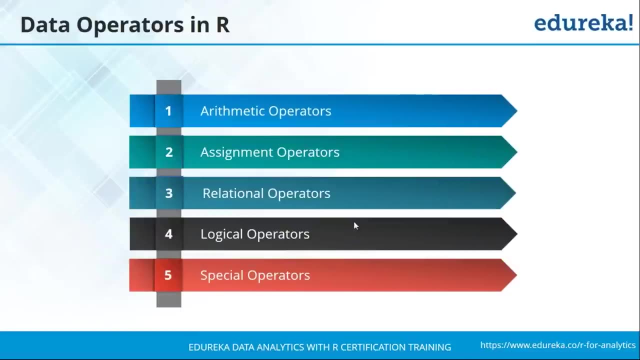 So clearly here with respect to what is a variable and how to declare a variable in R. Okay, That's great to see all of you've understood it. So now let's try to understand various data operators that are present in R. So there are mainly five types of data operators that you'll be working around with R. You 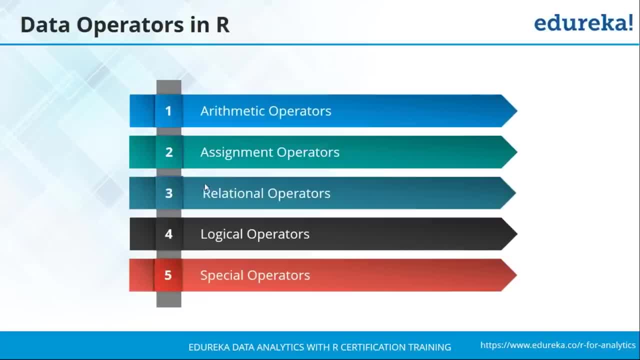 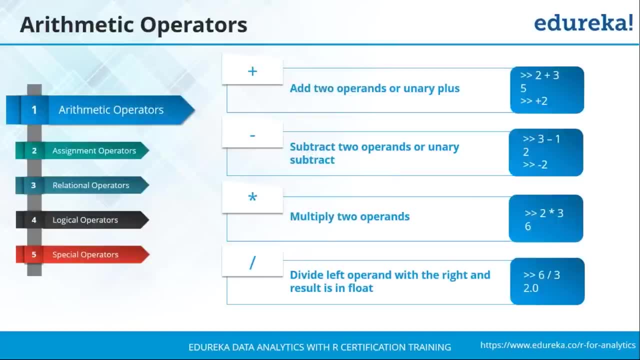 have your arithmetic operators. you have your assignment operators, relational operators, logical operator and special operator. Okay, So we'll start off by first understanding arithmetic operator. Okay So arithmetic operators are quite straightforward. You have your addition, subtraction, multiplication. 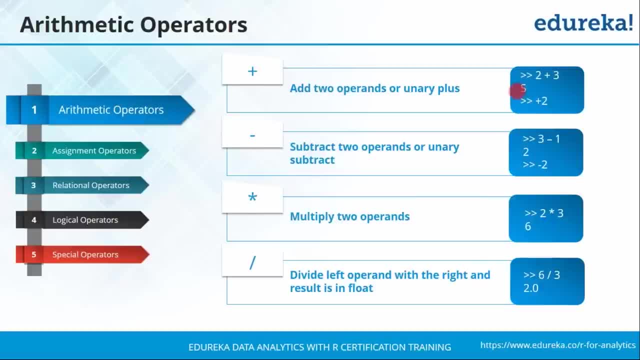 Now, if you look at the examples to the right here, again two plus three is giving me the answer. but plus two can also be a sign that it's a positive two value, Again same with subtraction. three minus one is giving me a result of two and minus. 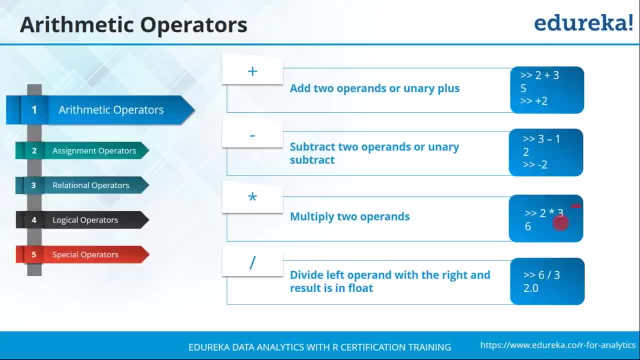 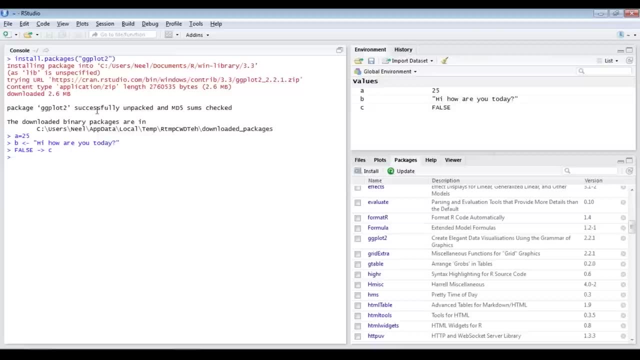 is actually used to denote that it's a negative two number, Multiplication and division are quite straightforward. Let me show you how they work out in R studio. So here, let's say I already have a variable a, So What I'll do is I'll create a new variable d equal to five. 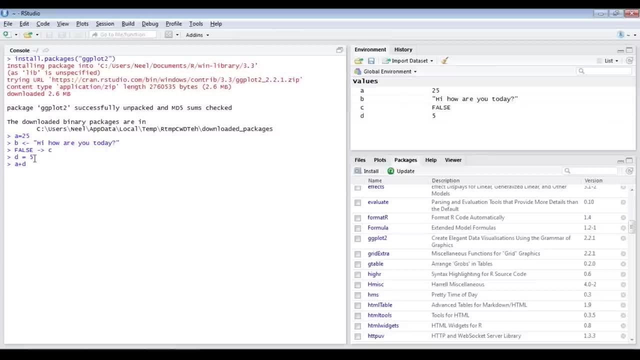 Okay, So let's say a plus d. You see the output as 30. A minus d Again. at any point, if you want to see the value of a variable, you can just type the variable name and the output is correspondingly shown there. 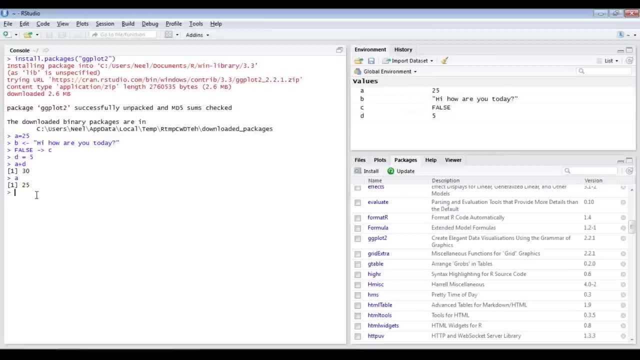 Okay, So apart from seeing the value here, you can always check it on your console as well. Now let's say: a into d is 125.. A divided by d is giving me the answer as five, And so far basically all your arithmetic operations can directly be performed here. 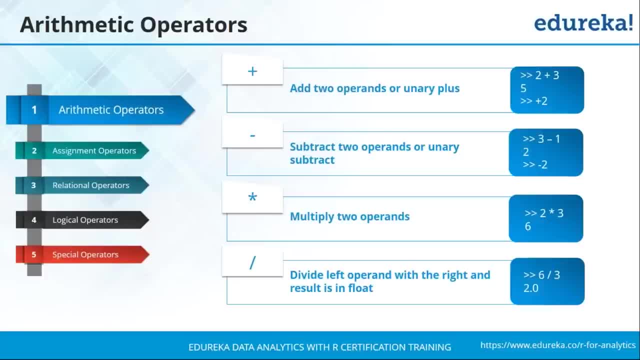 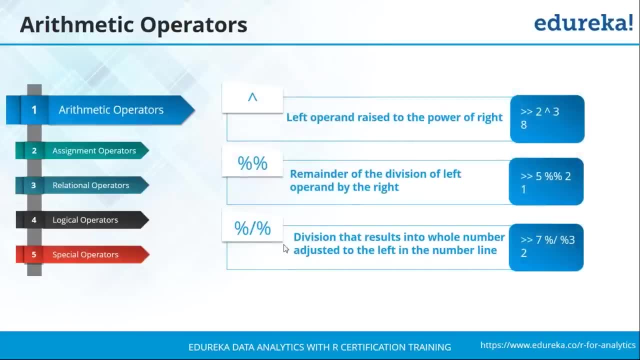 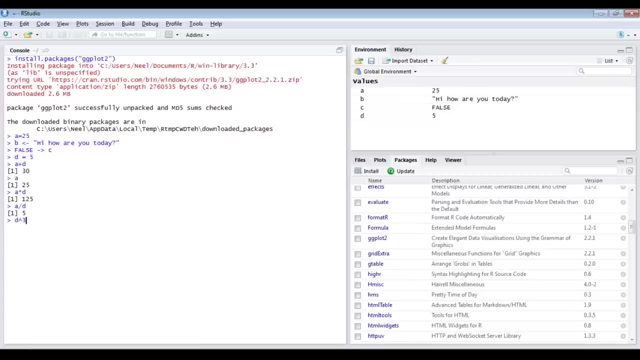 and then you can go ahead and execute it. Now, apart from these four basic arithmetic operations, you also have specific operators, where you have an exponent operator, and then you have a specific division operator. Again, when you talk about exponent operator, let's say d to the power of three. 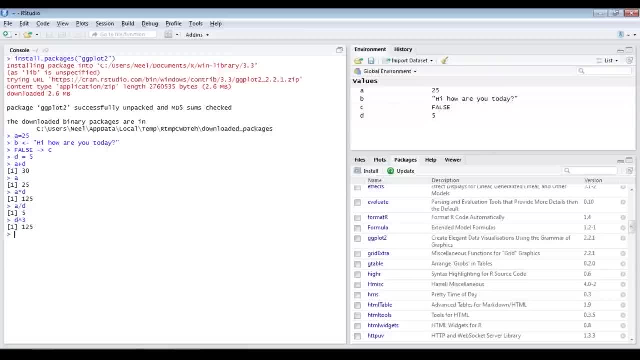 Okay. So basically, what I'm trying to tell is five to the power of three, That is 125.. Let's say d to the power of three, Okay. Let's say d to the power of eight, Okay. So this is the corresponding answer with respect to that same. 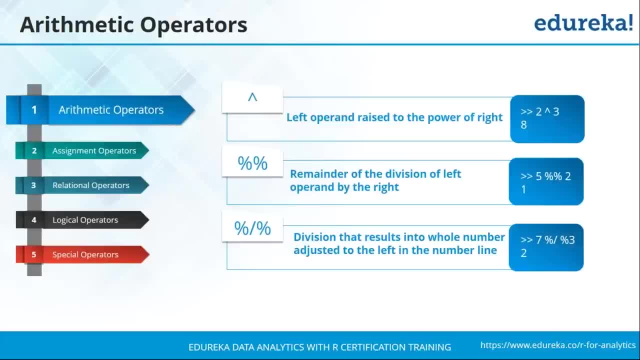 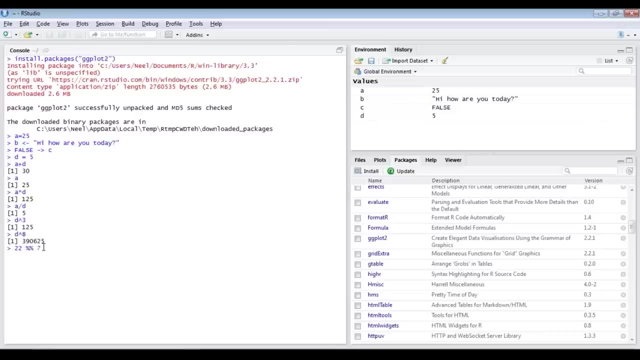 Now again, the second operator in this list is basically a modular division. What it basically does is it divides the number, But instead of giving you the quotient, it actually gives you the reminder of the division. Okay, Let's say I'm going to divide 22,. face percent, percent seven. 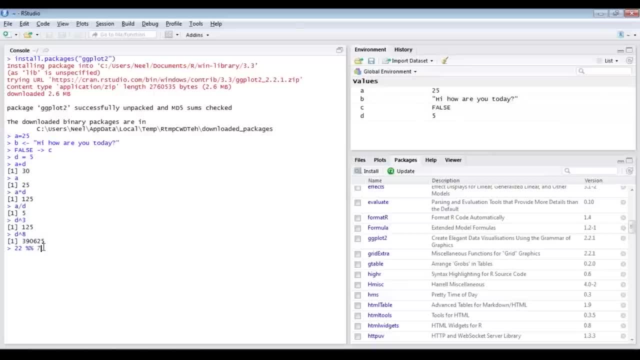 Okay, Now we all know this is going to give us the value of pi, But what happens if I do a modular division? Then it is actually giving a reminder of one instead of the value of pi. Okay, Instead of giving me the quotient, it is actually giving me the reminder and it's making the 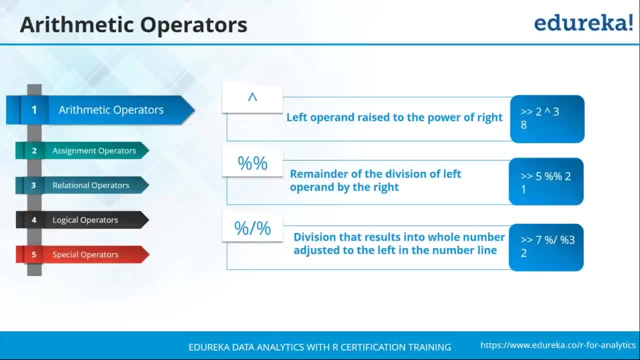 division as terminating. So the last division here is a floor division. What floor division basically does is it divides the two numbers, but the quotient that you get that is always rounded off to the previous value. Okay, So I'll just clear my screen in the R studio and let me just show you. 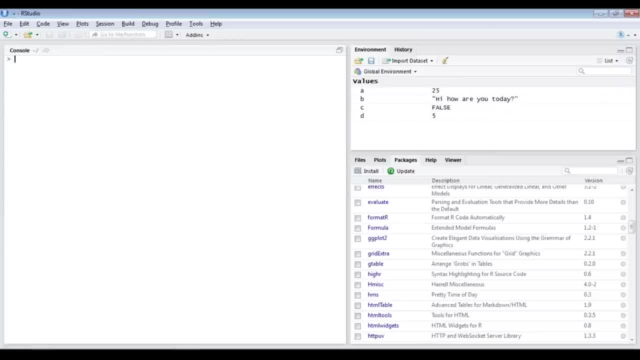 So let's take the most useful case Now again. let's say 22 when I modulo divide by seven, Okay, Now, we had seen the value to be one. Okay, Same time. But when I say, a normal division of 22 by seven is giving me the value of pi, that is. 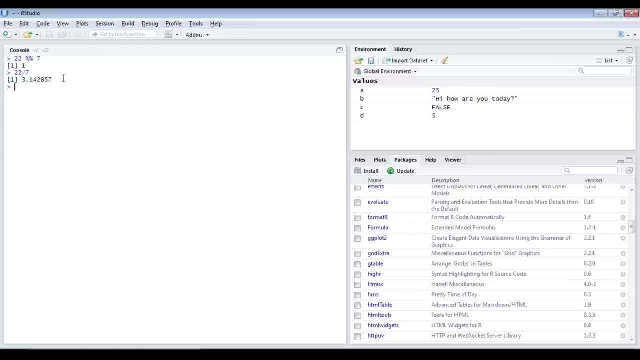 3.142857.. Okay, Again, this is a non-terminating, but it has chosen to put only six decimal points after the value. If I say 22 floor division, okay, of seven, then it is giving me a value of three. 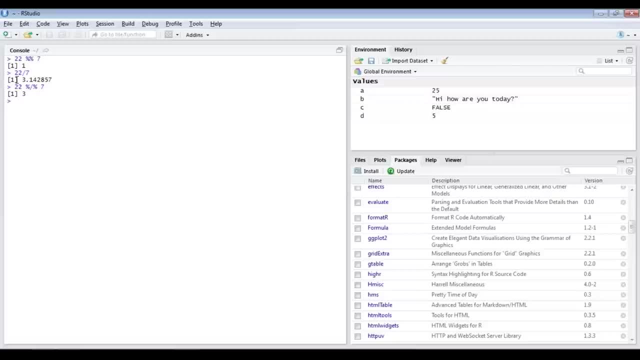 That is, it has rounded off this value to the value of three. So are you guys clear with respect to these arithmetic operators? Okay, So Reshma is asking me a question: What if the decimal point value is greater than five? Okay, 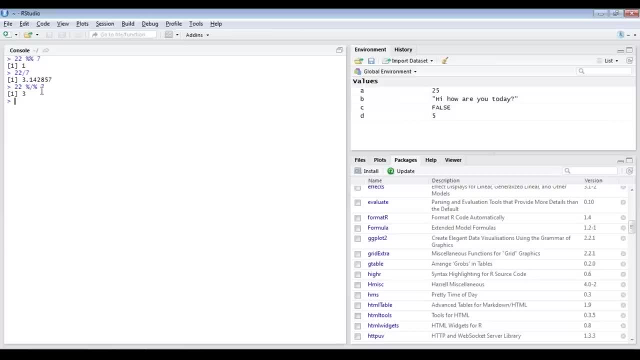 That's a very good question, Reshma. So I'll show you an example here. Let's take a random number here. Let's say I'm going to take 3.8.. Okay, 3.8 floor divided by two. 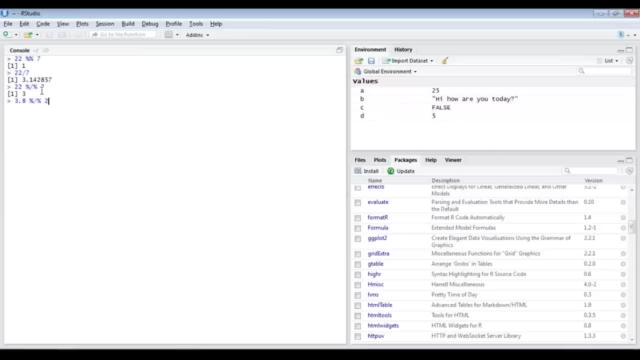 What's going to be the number, What's going to be the answer? Can anyone tell me? Okay, I have multiple answers here, both one and two, So let's just check this out. The answer is one Because, as long as it does not reach a complete whole number, it will always be rounded off. 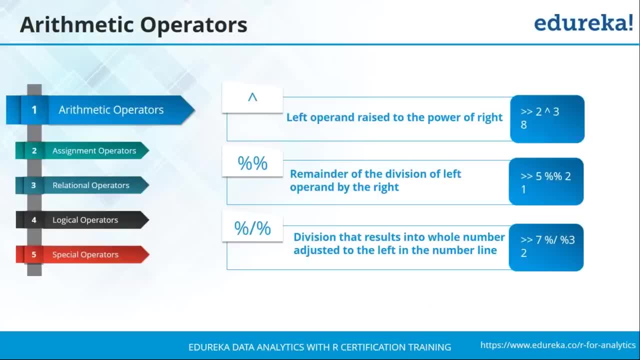 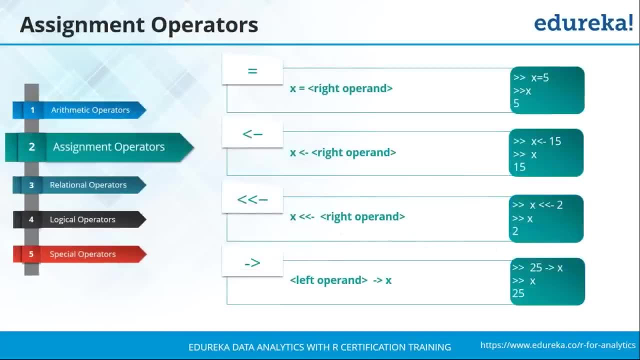 to the previous number. That is exactly what your floor division does, So does this clear your doubt, Reshma? Okay, That's great to see. Now the next operator is your assignment operator. Now, we've seen the assignment operator. 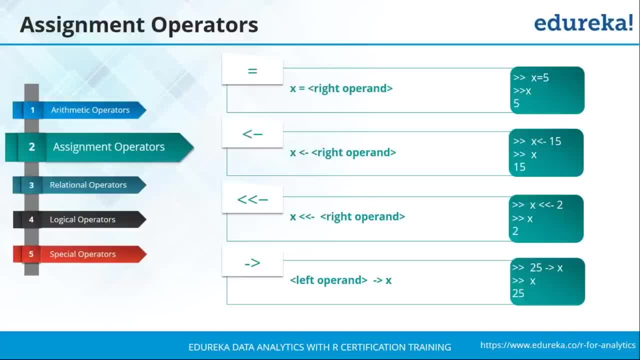 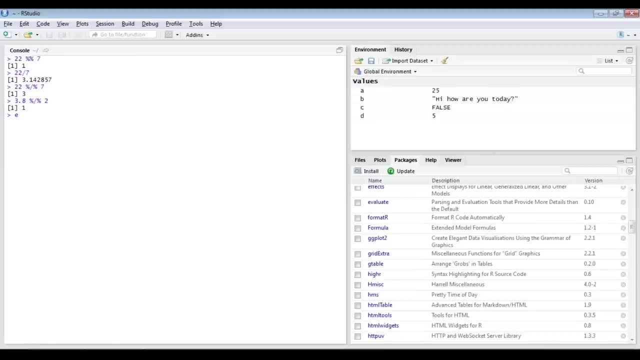 You can always use an equal to sign. You can use the less than, followed by hyphen. Now again, it can be a double less than as well. So I think we have not seen that. So let me say E equal to 50.. 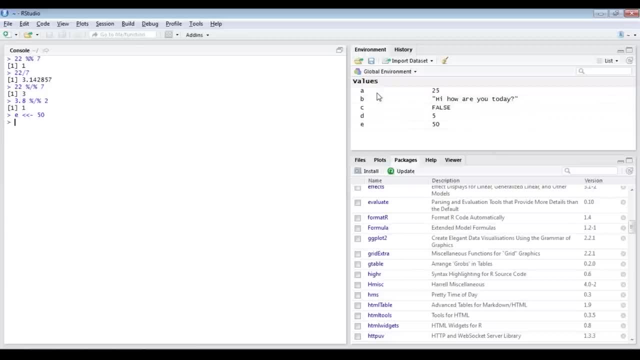 Again, same result. A new value has been entered into my environment, So you can see. E is of a type numeric which is taking again 48 bytes and the value is 50 here. Okay, Now again, same process can be followed for assignment to the right hand as well. 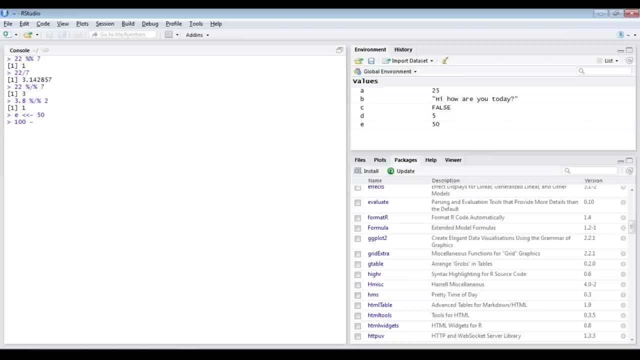 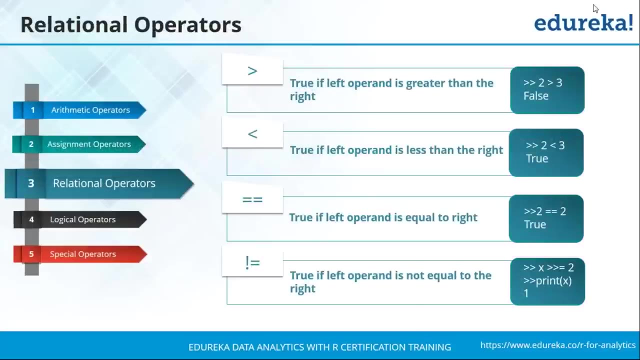 Again, let's say 100 hyphen greater than greater than to the variable F. So again, F has been added to my variable list with the value of 100.. Okay, So these are how you work around with assignment operators. The next set of operators are relational operators. 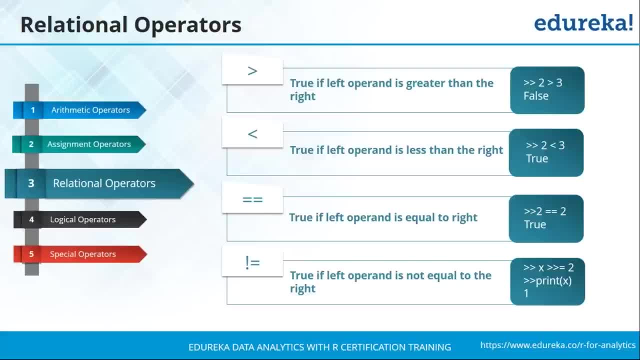 So relational operators are some of the most interesting operators. I like working around in R because these actually act as a base to various different operators that we'll be seeing ahead. Various statements, Various operators, Various operators are dependent on these simple relational operators and they're quite 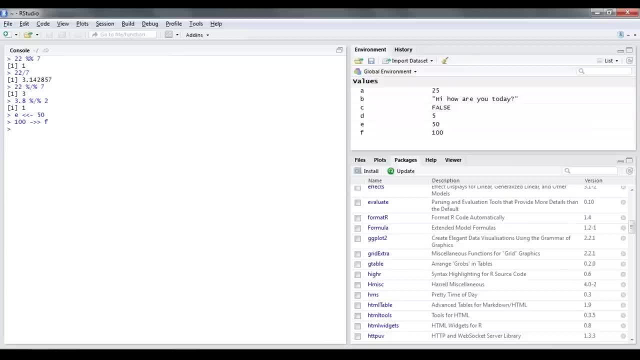 useful as well. Now again, all your relational operations will give you a Boolean value as your output. Okay, So let me just show you an example here. Let's say my F is greater than E. Okay, It's a simple statement here. 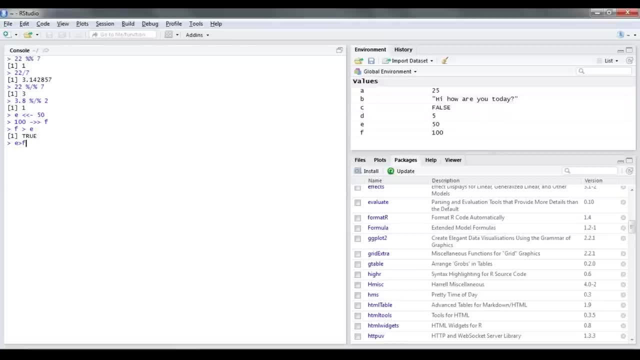 You can see the values. If I say it is true, But let's say E is greater than F, then basically it's returning me false. Same case you can see. and when you want to compare two operators, then you're going to. 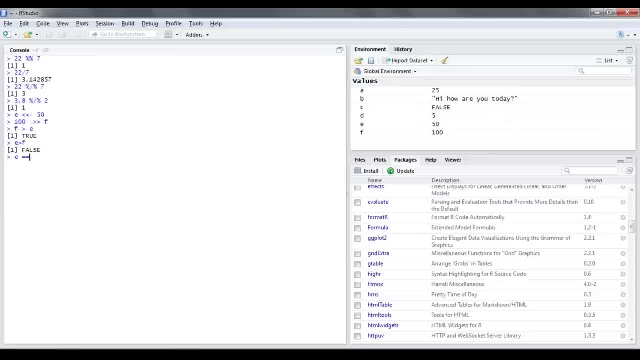 use a double equal to operator. So say E equal to equal to F, Then it says false, no, they have different values. And when you want to check whether two values are not equal to, then again it's quite straightforward. Let's say D not equal to. 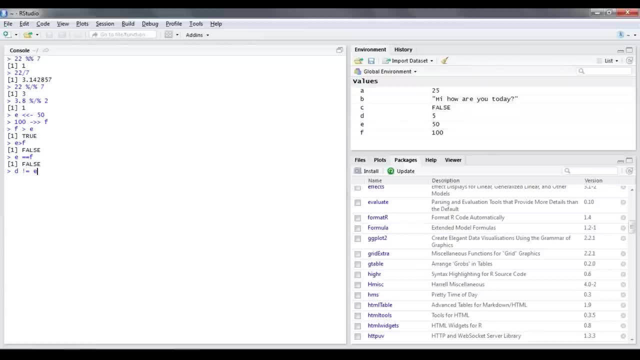 So again, not is denoted by an exclamation mark. Not equal to E, Then it says: true, both D and E have different values. Again, if you check in my environment, list D has a value of five where E has a value. 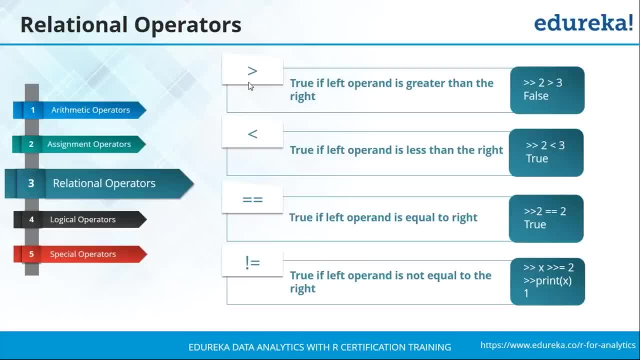 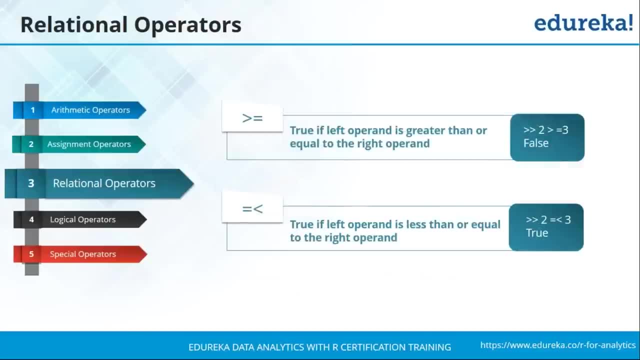 of 50.. Now, apart from a single operation of less than or greater than or equal to or not equal to, you can combine the equal to with both less than and greater than, where it becomes to greater than or equal to and less than or equal to. 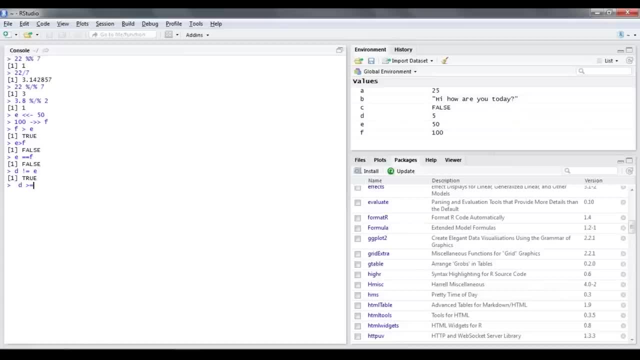 Now let's say D is greater than or equal to E. It's false. But let's say I'm going to take another variable, say G equal to five, okay, And then I'm going to say D is greater than or equal to G. 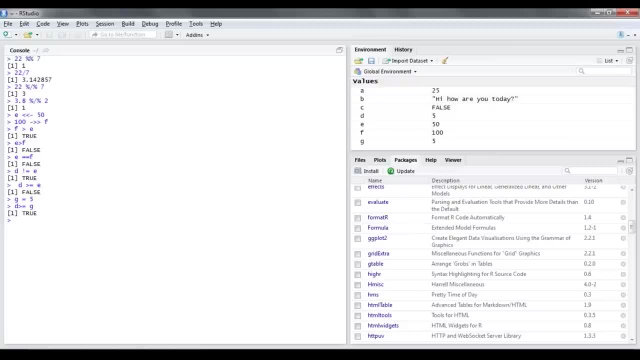 Okay, Here it is giving me true, because both conditions are being checked, whether D is either greater than G or is it equal to G. Only when you've tested these two conditions, whether it is greater than no, it's false. 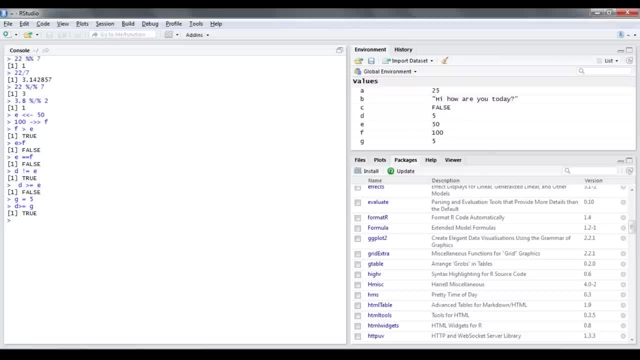 And whether it is equal to no, it's false. Only in that case will you get an answer to be false. But if either of the conditions are found to be true, then the answer comes back as true. So are you guys clear with respect to the first three kinds of operators? 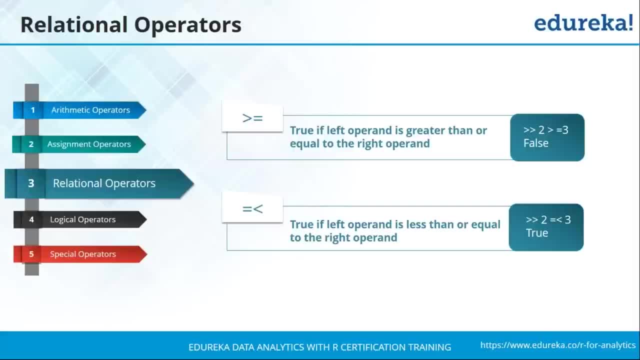 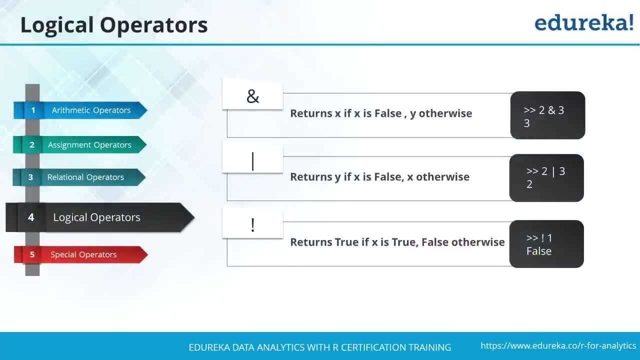 That is, arithmetic, assignment and relational. Okay, So moving forward, let's talk about the next type of operators, that are logical operators. So, with respect to logical operators, there are mainly three types of operators. You have your AND operator here. 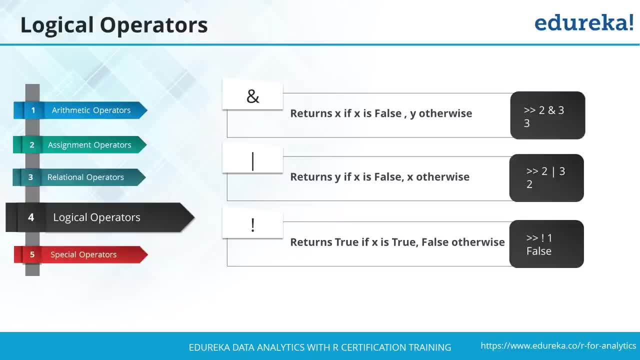 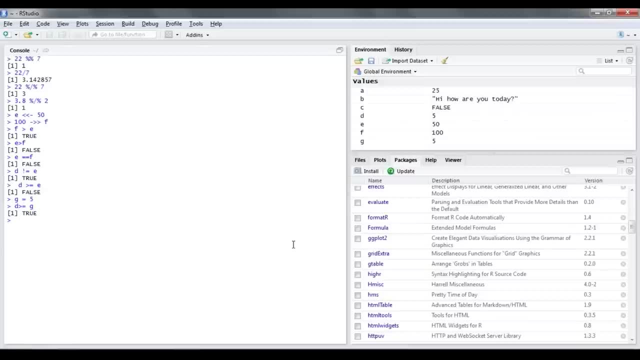 Then you have your OR operator and NOT operator. So, with respect to your AND operator, let me just show you how it works out. Okay, So here what happens is I'm going to assign two new variables. Let's say X is equal to true and my Y equal to false. 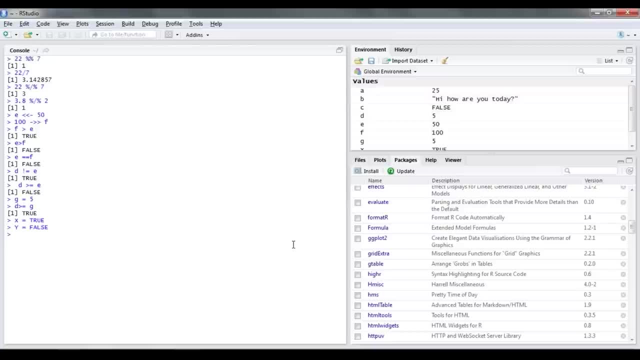 Okay. So let's say X and Y. So let's say X and Y. Okay, So the value of one is true, the other is false, But it is giving me an output to be false. But at the same time, let's say X and X is giving me a value of true. 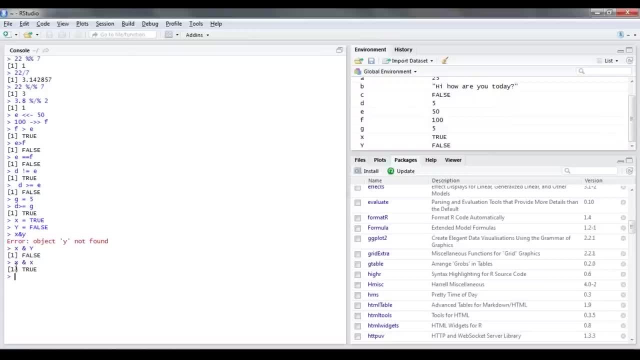 So your AND operator gives you true only and only if the value of both your operands, that is, your left operand here And your right operand here, their value is true. Unless, and until both these values are true, you do not get the output to be true. 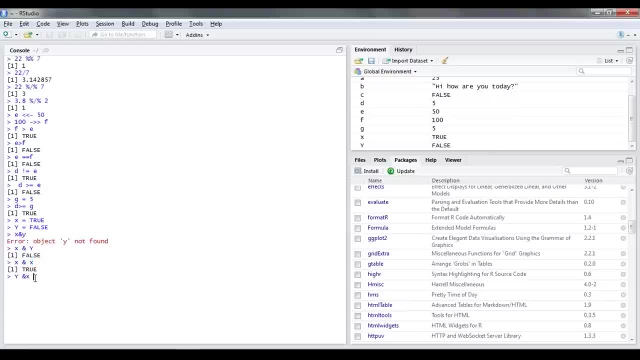 Now again, let's say Y and X. So this is false and true. Okay, It's giving me false. And let's say Y and Y is giving me false. So here you can see. the only case where I'm getting true is when both my left operand 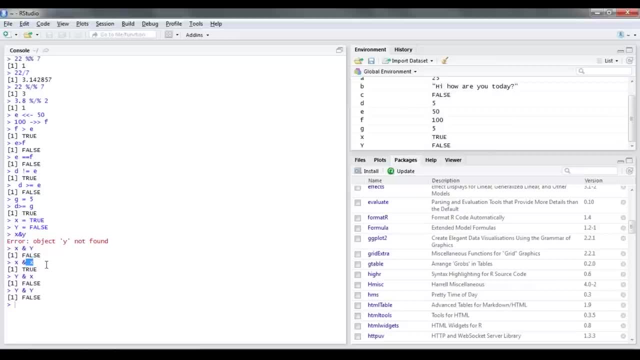 and my right operand is having a value of true. Now keep this in mind. This is something that is going to be very important while we're working with conditional statements, So make sure you're quite clear with respect to how a logical AND works. 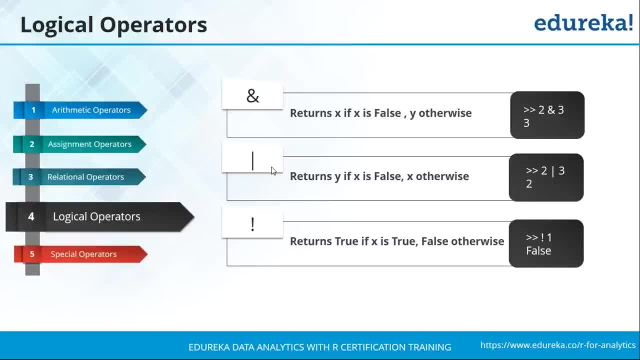 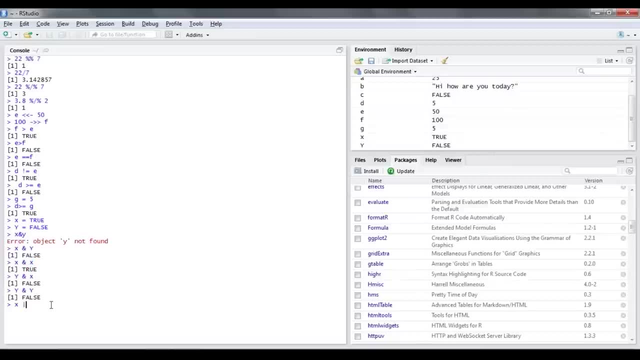 Okay, But similarly, when you look at the next operator, that is, OR operator, this is quite interesting. Now again your OR operator. let's take X again here. And your OR is again denoted by a pi symbol, like your AND was denoted by an ampersand. 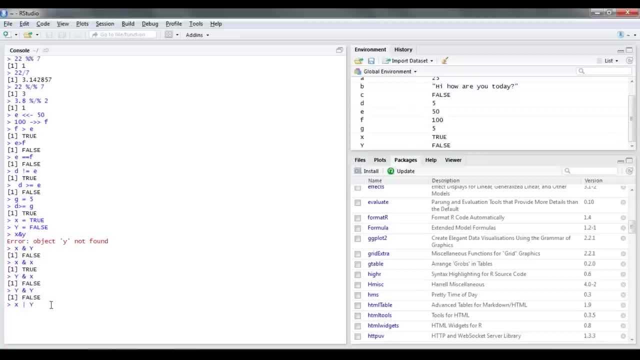 Let's say X and Y. Okay, This was the first condition that we had checked. Okay, Now here, what we're checking is X or Y. When I pass it, it gives me the value of true. Your OR operator is opposite your AND operator. 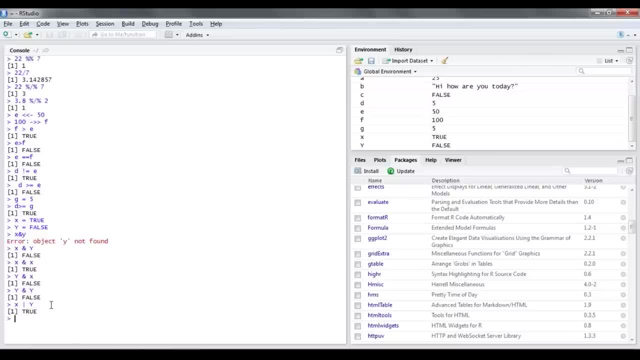 What it basically does is if any one of the two operands is having the value of true, then it returns your output to be true. Earlier, what we had seen with respect to the AND operator was only if both the values are true do you get an output to be true. 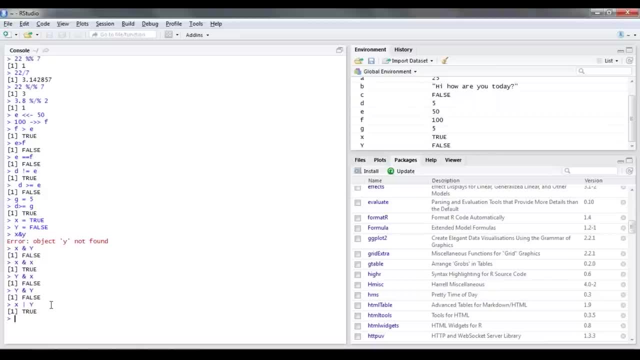 But with respect to an OR operator, as long as at least one of them is true, then the value is said to be true. Now again, let's say you've seen X or Y. let's say Y or X. okay, this is false and 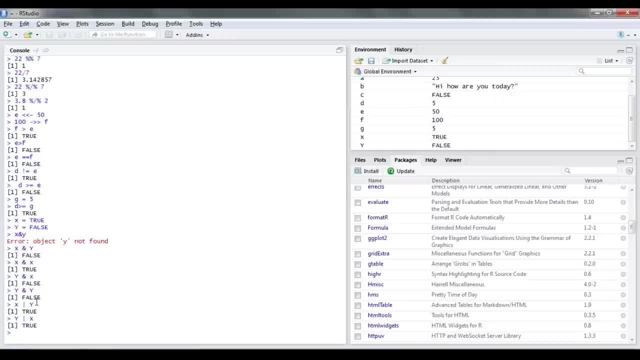 true is giving me true. Let's say Y or Y, then it is giving me false. So again, since I have both my operands to be false, it's giving me the value to be false. Now, the final logical operator is the NOT operator. basically, it converts the present. 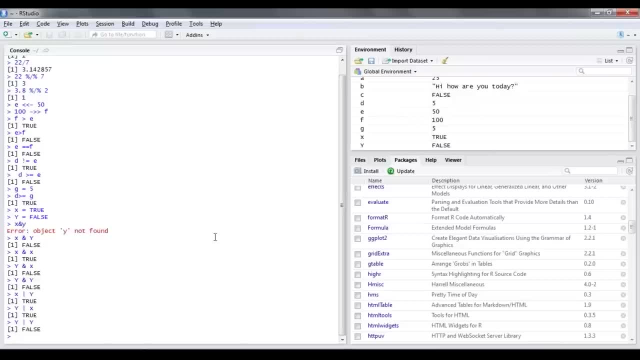 value to the opposite value. Now, If I know my Y has a value of false. now what I'll do is to that Y I'll add a NOT okay, NOT Y, and I pass it. it gives me the value of true. 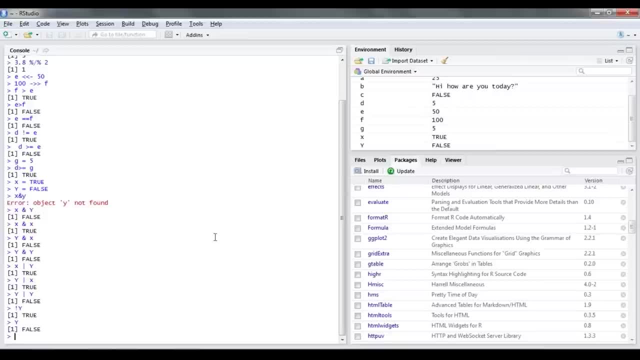 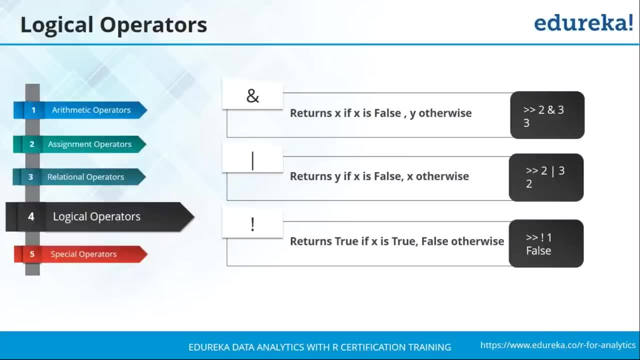 But again, when you check the value of Y, it is false. So your NOT negates the current value. That is, if it is true, it becomes false, and if it is false it becomes true. So are you guys clear with respect to the logical operators? 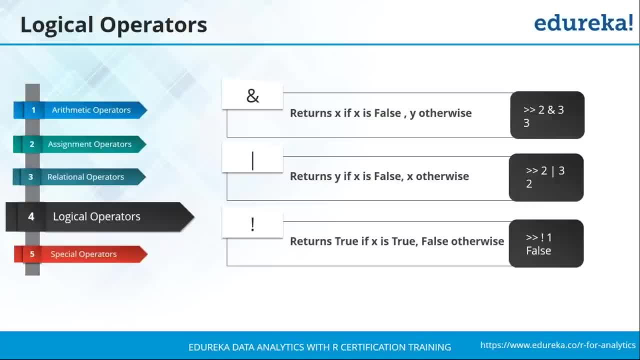 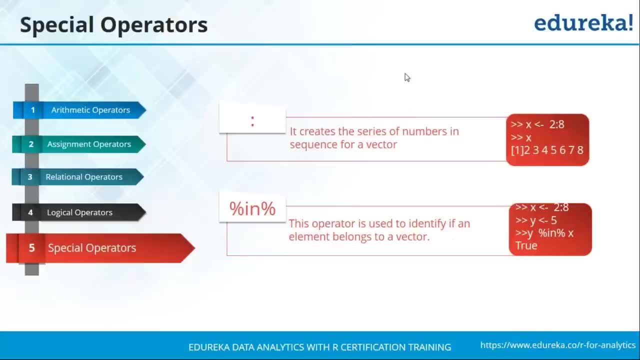 It's quite important that you understand them well. So all of you seem to be clear on this. So let's move forward to the final operator, And that are special operators in R. okay Now, the first is the range operator. So your range helps you identify, that is, store a sequence of numbers within a specific 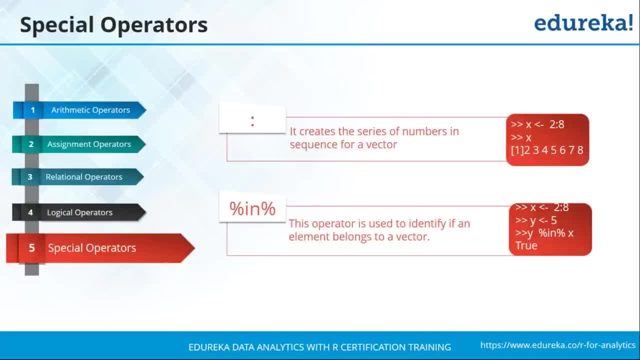 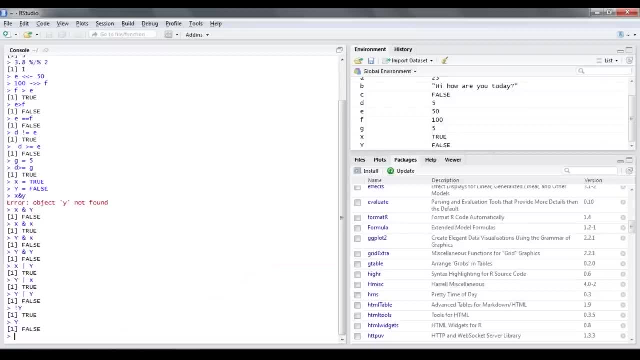 range. Now you need to specify the first number and the last number on the left hand and the right hand of the colon. This tells that all the values present in this range have to be stored in a variable. Now again, let's say I'm going to create a new variable, say H, that is going to store 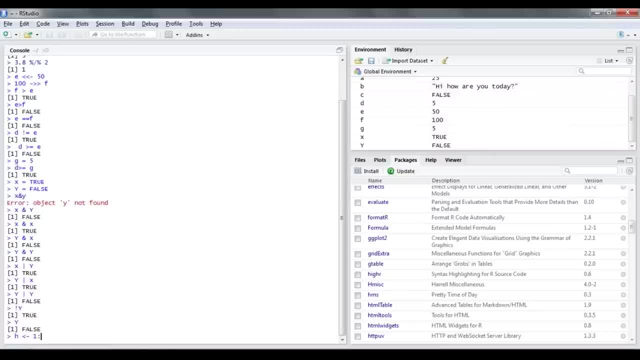 a range from 1 to 10.. So 1 colon, 10.. And if you look at H value here, okay, it's having an integer value which is storing the values from 1 to 10.. Again, if you want to check the value, you can also print it on your console, just type: 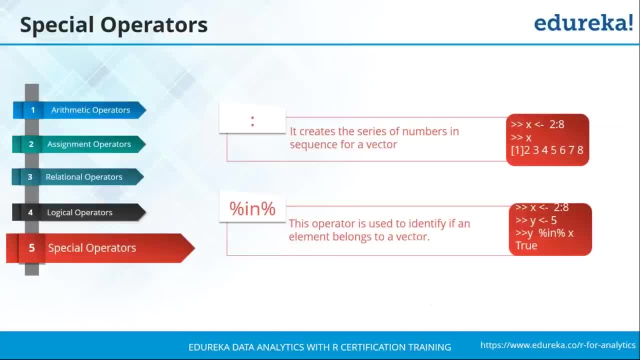 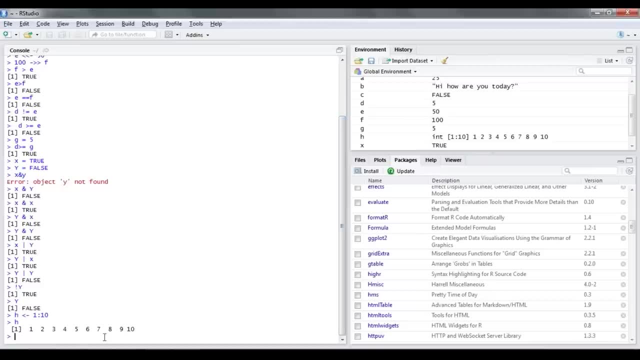 the variable name and you can see the values here. Okay, the next special operator basically is an IN operator. It checks if a specific element is present in that value. So this is something that you'll definitely be using in a range of values. 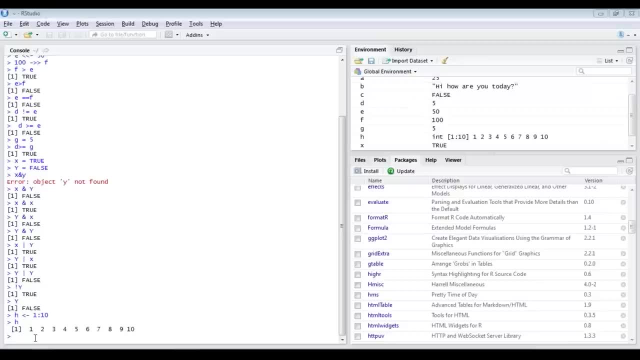 Now let's say I want to check if a variable, let's say, is 6.. Okay, So I'm going to check that If a variable 6 is present, okay in my H variable. So what it does is you're checking if a value 6 is present inside your variable. 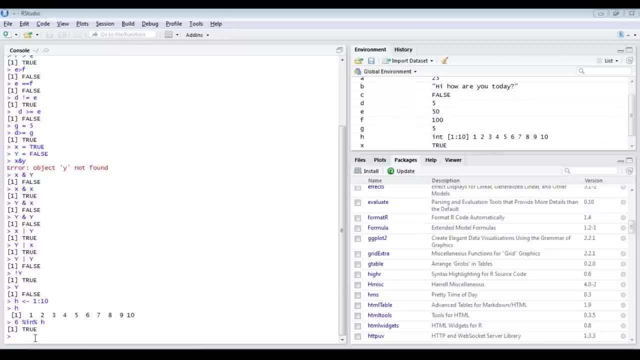 And it is giving me a Boolean value, whether it's true or not. Now, let's say I'm going to check a value 15 in H. Now we know that H is a variable that is storing the numbers from 1 to 10, so this should give. 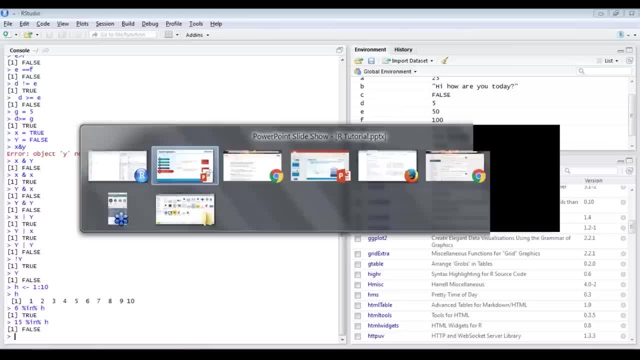 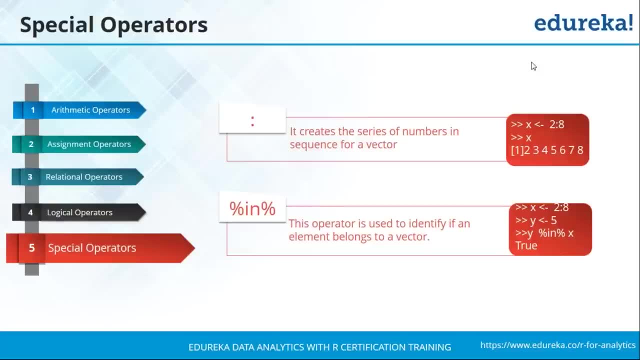 me a value of 5.. So are you guys clear? So we've come to the end of the various operators in R. So any doubts with respect to this, Any of the operators that you're not clear, that you want me to repeat? 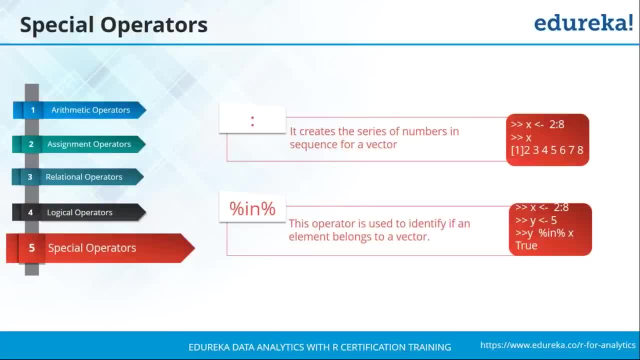 Okay, so I see everyone is clear. That's great to see. I mean, as an instructor, I'm quite happy that all of you are following. So again, remember, at any point you're not clear with anything, make sure you put it. 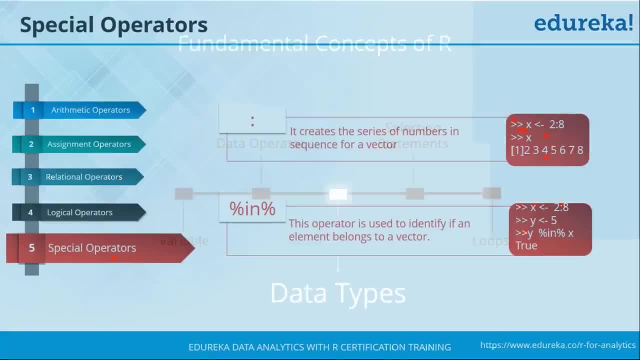 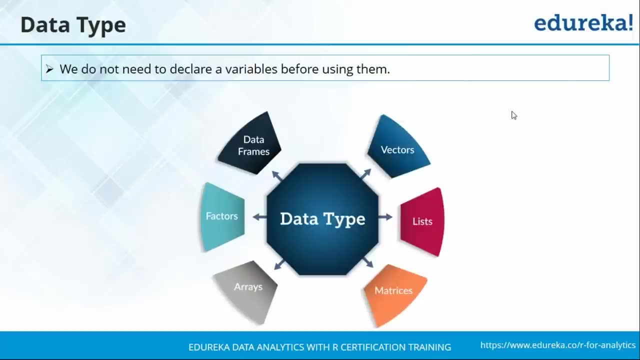 across in the chat box. So let's move forward to talk about the various data types that are present in R. Now, talking about the various data types in R, there are mainly six data types present in R. You have vectors, you have lists, you have matrices, arrays, factors and data frames. 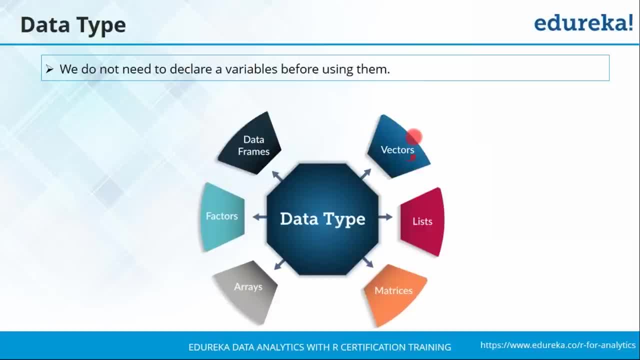 Now vector in itself have six atomic data types, but not going into that right now. One thing you may have noticed is that at any point when you need a variable, you can go ahead and declare it as part of your code, So this becomes quite easy for you. 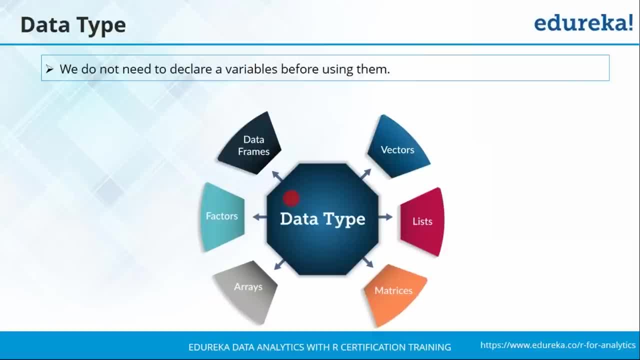 You don't need to declare it first itself. or let's say, while you're working on your code, suddenly you realize a new variable has to be created. You don't need to go to the start and then declare it So at any point. 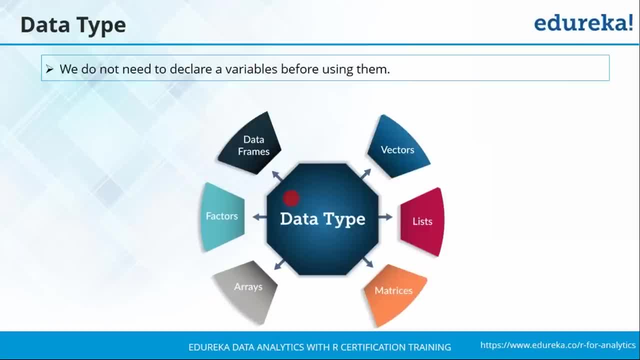 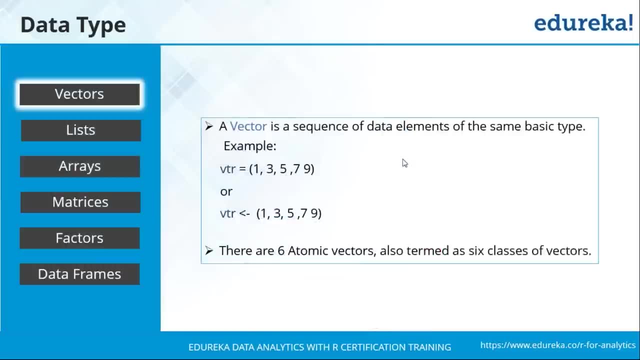 When you need a new variable to be created, you can create it right away, And we followed that same process here as well. So let's deep dive into each of these data types. We'll start off by understanding with vectors Now. vectors, basically, is a sequence of data elements that are of a basic data type. 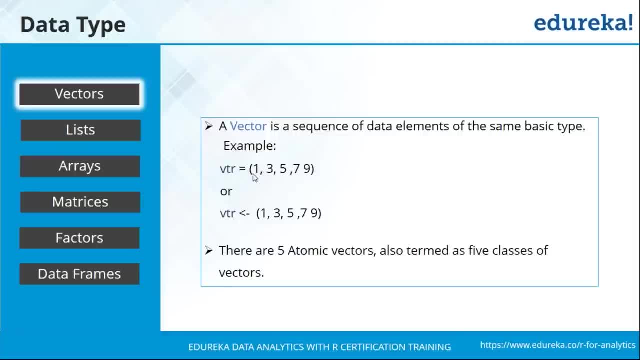 Now, if you look at the example here, what am I doing is I'm storing numerical values into my vector. Again, the assignment with respect to the vector can vary with usage of the assignment operator, but vector in itself can be classified into five different attributes. 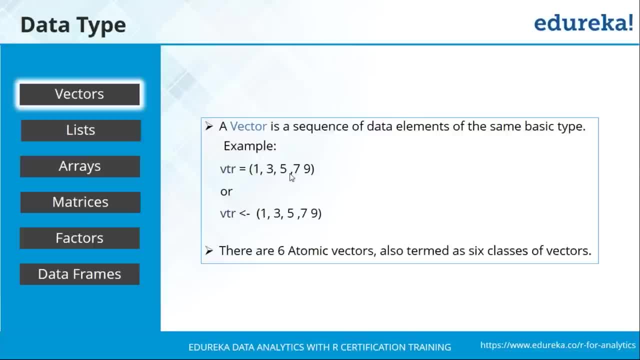 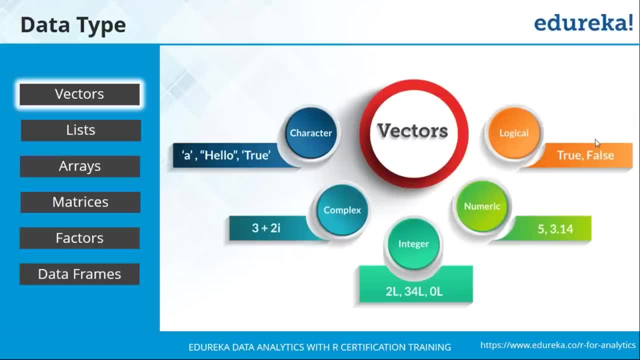 Atomic types, or they're better known as the five classes of vector. These are your character, complex integer, numerical and logical value. Now, in your logical value you basically have your true and false. In numerical it can be a numerical value and an integer can have an integer value. 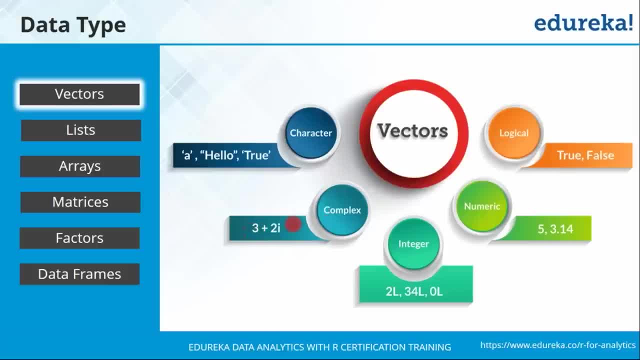 Okay, You can also work around with complex number, where there's a real and an imaginary part, And you can also work around with characters. Characters could be a single character, It could be a word or even a sequence of words or a sentence. 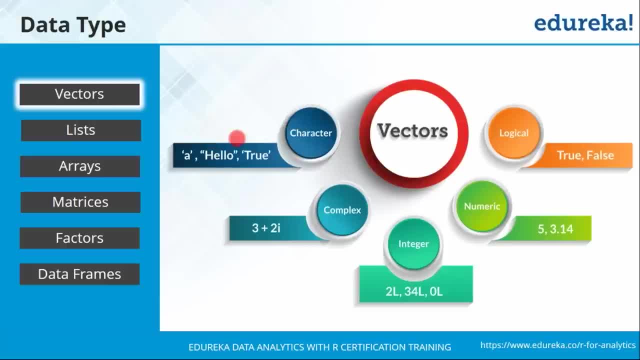 So your character variable would take a corresponding size, and R always takes care of the memory management, So you don't have to worry with respect to that. Now let me just give you an example for each one of them. Let's go back to RR studio. 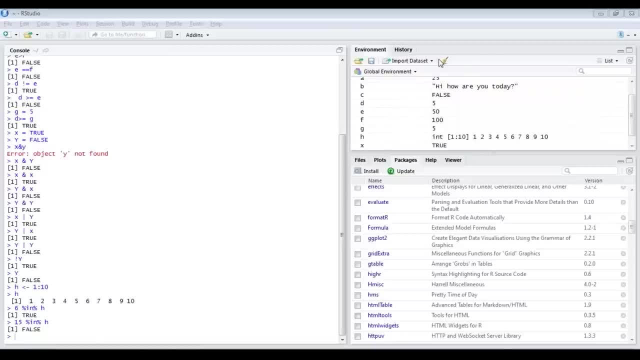 Now here let's say, if you want to clear the variables in your memory, all you need to do is click on this operator and automatically every object in your environment will be clear. Okay, Same for clearing your console. Just press control L and your console is also clear. 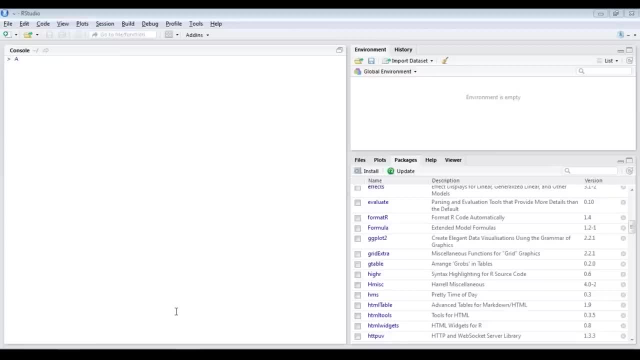 Now, with respect to your logical variable, let's say A okay equal to. you have both true and false. So again, true has to be written in capital because this is a reserved keyword, And when you write true you can see corresponding value has been set. 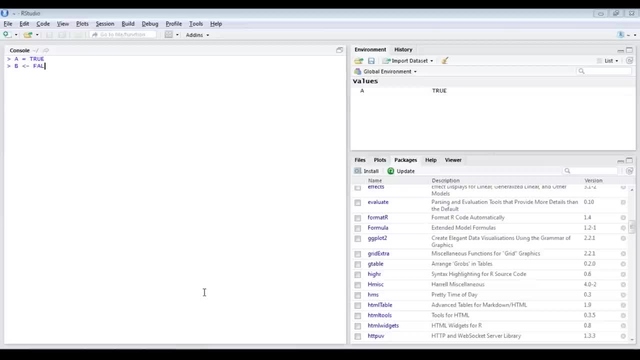 Same can be with respect to B, which is going to store false value. Again, these are reserved keywords that have a certain definition already present in R, So they would. you would get a correctly prompted response. So A and B are true and false. 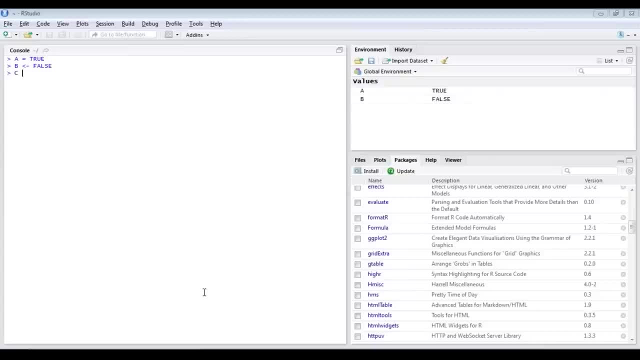 Now, with respect to numerical values, let's say C is going to store five. okay, And I'm going to create another variable which is going to store an integer value. So D is equal to five and to denote that it's an integer, you need to add a corresponding. 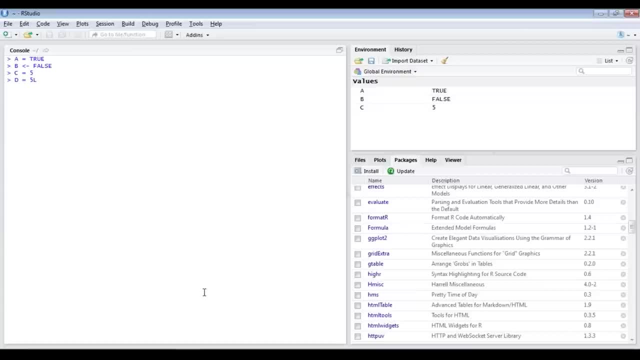 L associated with it. This basically tells R that this is an integer value. Now here, when you look at your environment, C basically is a numerical value which is storing 48 bytes. But when you come down to D you can see it is of an integer type that is using 48 bytes. 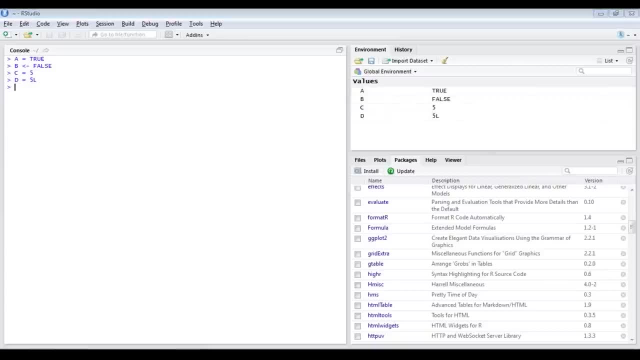 for its memory location. So Gayatri is asking me: how is integer different from numeric? That's a very good question, Gayatri. Okay Now, if you talk about integers, they are actually used to store whole numbers. You cannot store a decimal pointed value or a fractional number inside an integer. 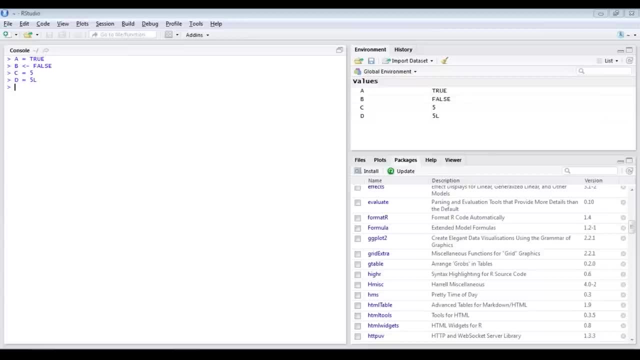 But in your numeric you can store decimal values in the float class as well as whole numbers. So numeric could be the whole set, where your integer is basically a subset of your numeric. Does that answer your question, Gayatri? Again, if it's not clear, let's say E equal to 8.5 L. 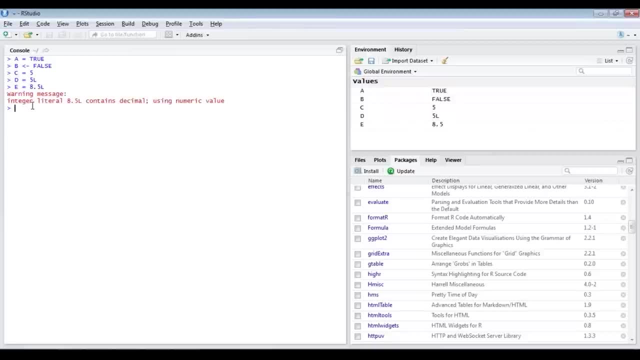 Again, when I try to do this, it gives me a warning that integer literal 8.5 contains decimal use numeric value. Okay, But when you see a new value has been created in my memory and if I go there you can see. 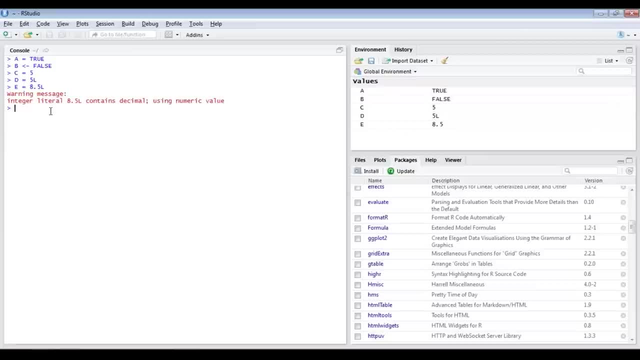 it is of type numeric and not integer. So does this answer your question, Gayatri? Okay, Now, apart from this, let's say I have F, which is going to store a certain character value. Let's say R is fun, and there you have it. 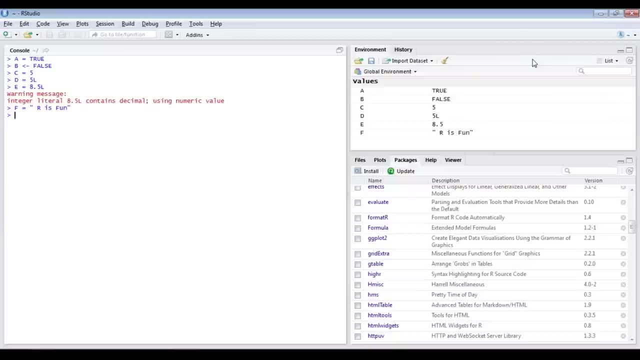 So any doubts with respect to the data types that we have discussed till here The five basic atomic data types. Again here, one thing you need to remember is, while you're working with these atomic classes, you don't need to specify the data type for them, for the variable that is. 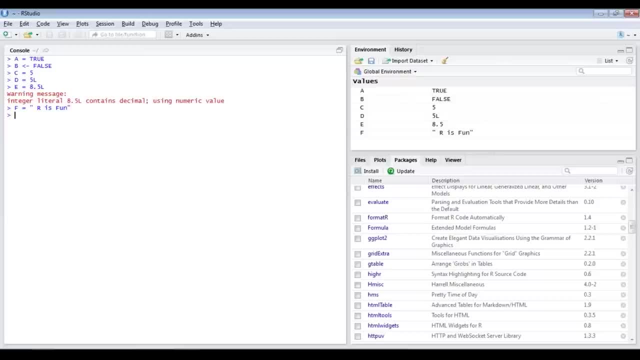 Okay, Automatically, R checks the value and decides And assigns the data type for these variables. Okay, So it basically reduces your effort by half. All you need to do is decide a variable name and then fix the value for the corresponding variables. 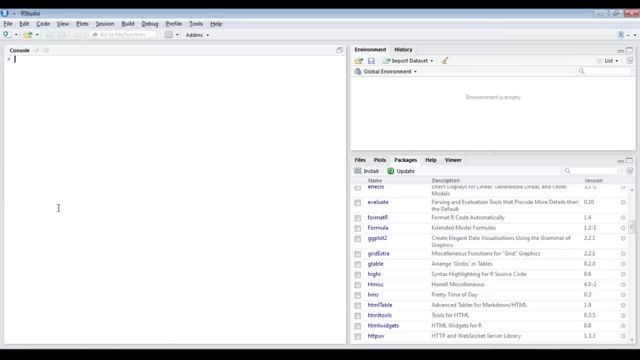 Okay, So any doubts? Now let's take a new empty workspace. Now, as we had mentioned earlier, a vector basically is a collection of different data types. So let's take a vector, VTR, and to that let me just store a sequence of numbers. 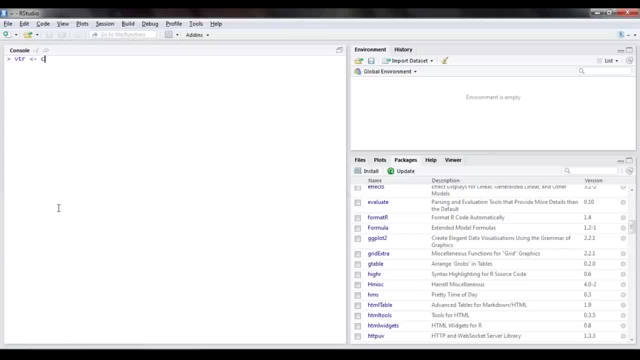 Now again, we had done this earlier as well, When we had seen, We had seen these special operators. but again, let's take the same case here. Let's say I'm going to store one, I have three, then I have five, there's 11,, 45,, 23,, 67,, 55,. 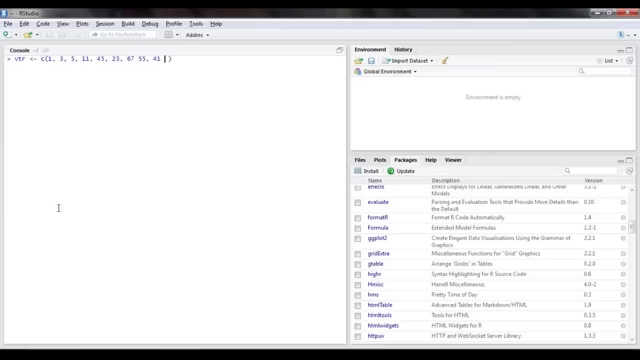 and finally, I have 41. So these are the numbers that I'm going to store inside my vector. Okay, So, As you can see here, there's a missing comma between 67 and 55. So, again, it makes a big difference when you're specifying different values, because it becomes 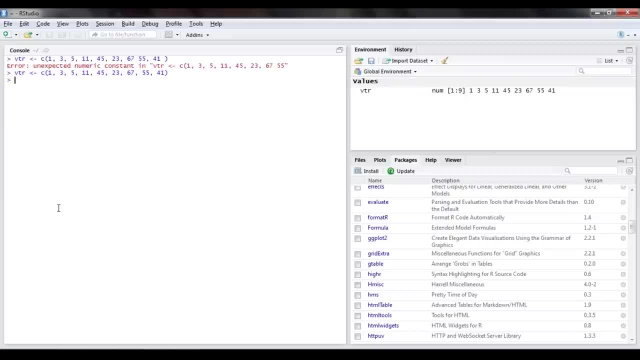 hard for R to identify the different values. Okay, So now you can see a new vector has been created. I have nine elements, starting from one it goes all the way to 41. So this is a simple collection of vectors of numeric type, and nine values are stored. 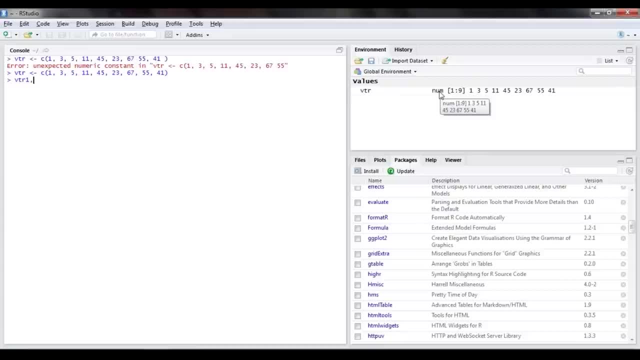 here. Similarly, you can have another vector, one that is used to store different characters. I'll say: Half One, Hi Another, Hello Again. characters need to be in quotes. Okay, These can be single quotes or double quotes, but always make sure you put it across. currently. 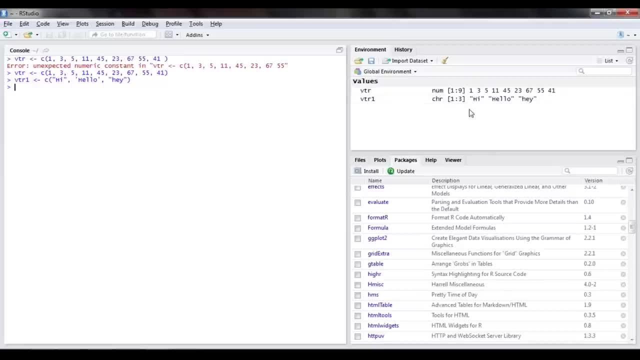 And I'll put in: hey, So again, you can see. these have been added correspondingly to the new vector. So even if you have a single element or if it's a collection of elements, it's always a vector. Are you clear with this? 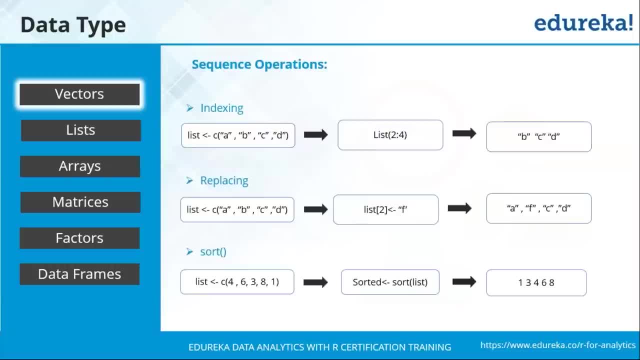 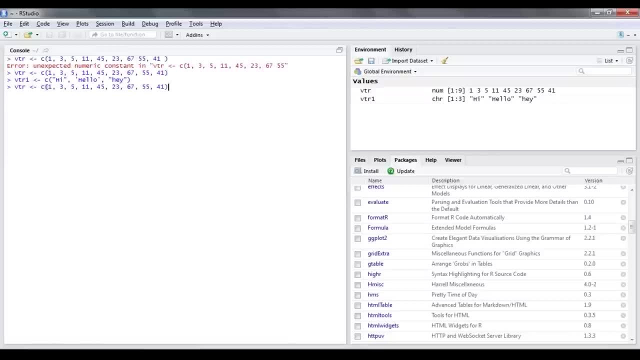 Okay So. So some operations that you can perform using vectors are basically indexing, replacing sorting, So let me just show you these operations as well Now, Okay, So this is a vector of different numerical values. So to sort it, let's say I'm going to create a new vector, say sort, and to that 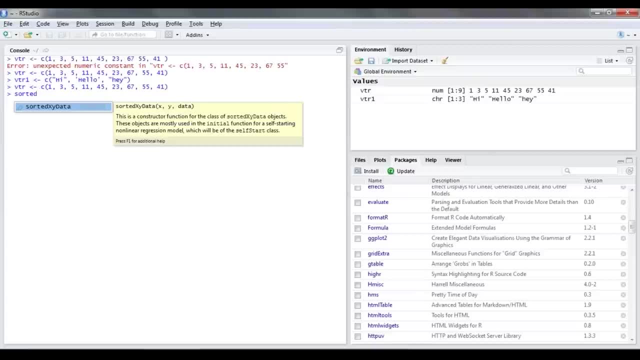 Okay, Sort is basically a keyword, So I'm going to say sorted VTR. Okay To this. I'm going to sort my vector and then store it. So sort is an inbuilt function. You can call it and you can pass the data type here. 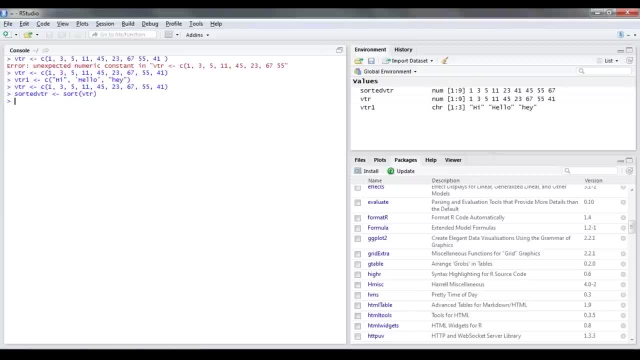 So vector is what I'm going to pass, And then if you print sorted vector then you can see the complete list has been sorted and it's getting printed here. So in it out with respect to the same. So this is something that you can perform for any data. 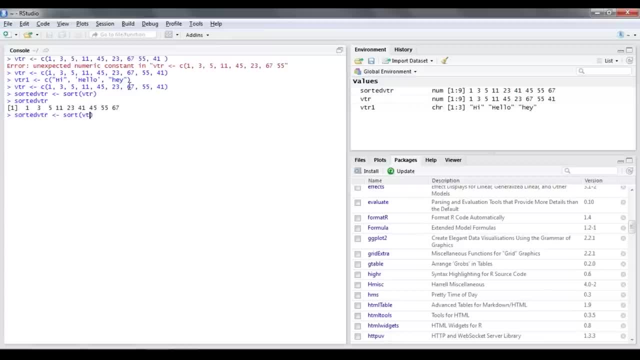 If you pass a character data type, then what happens is basically sorts based on alphabetical order. So here let's say VTR one, And if I print it again So you can see, it's rearranged Everything in an alphabetical order. 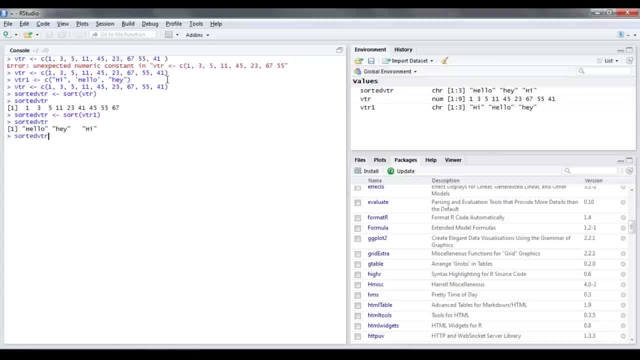 So as long as it's a vector, you can perform the sort operation. Apart from that, let me just take the vector VTR And here, if you want to access any specific elements, in that case just use a square bracket and you can specify which element you want. 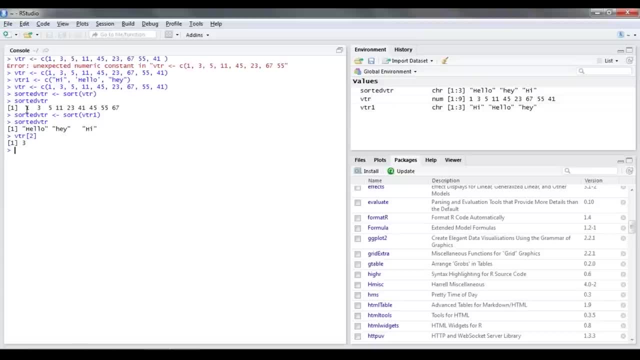 So let's say the second element, then press two. So if you see the complete vector, the second element is three. But let's say you want a range of values, Then what you can do is two colon. I want the values from second position till sixth position. 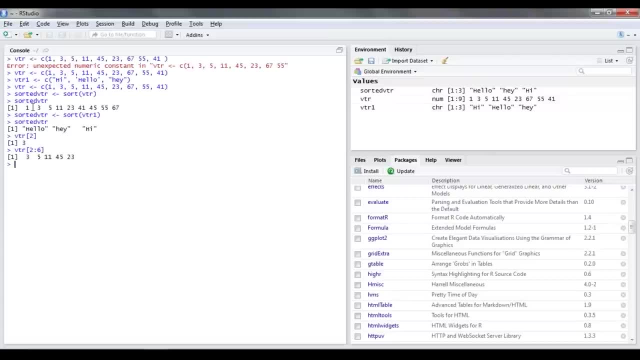 Then you just need to specify the start point and end point of that range and all the values get printed with respect to that same, Including the range values, That is, number two, three, four, five and six. Okay, so who can tell me what will happen if I give minus one here? 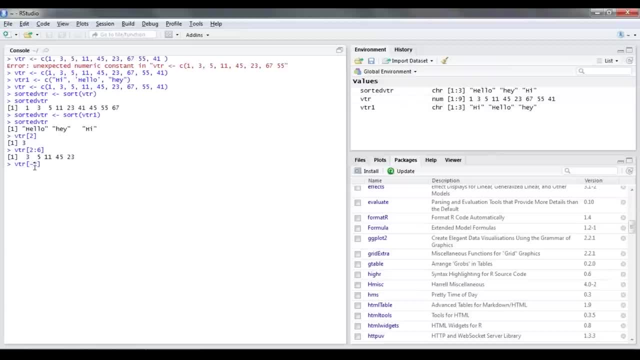 Okay, so all of you are telling me the last element will get printed. Okay, let's see what happens. Can anyone tell me what happened here? Yes, When you say minus of an index, it basically means excluding that index. Okay. 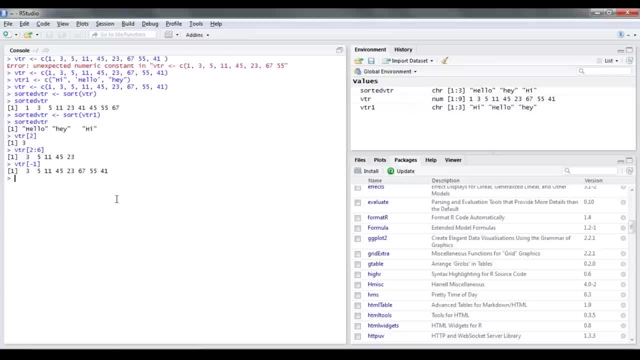 Okay, great. Now again, let's say if you want to replace a specific element in your vector list. So let's say, I want to replace the third element in my vector, that is five, with, let's say, 15.. It's a quite straightforward process. 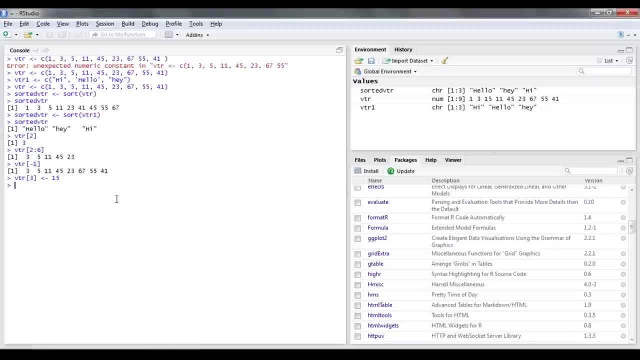 You just need to specify the index, followed by the new value, And if you print the vector now. so now, if you just print vector VTR, you can see the updated value. where I had five originally, it's getting replaced by 15.. 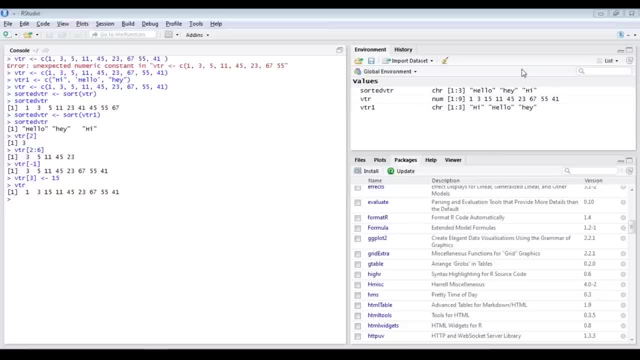 So this is basically a replacement of a specific value. Are you guys clear with this? Okay, so one last trick question: What happens if I say, replace it by 11?? So I have nine positions here. If I'm going to put 15th in my 11th position, what will happen? 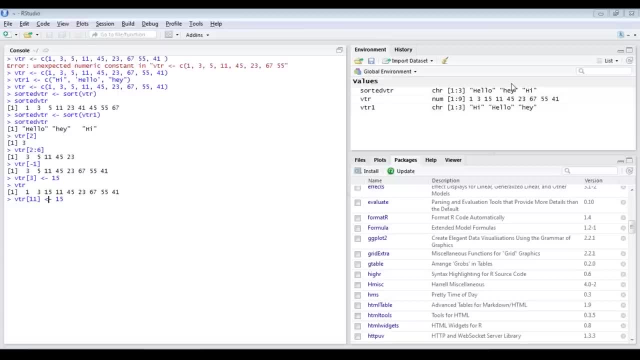 Okay. so some of you are telling it will not get added. Some are telling it will get added to the 10th position. Let's see what happens. Do you think this command will execute successfully? Okay, I find a lot of yes and no. 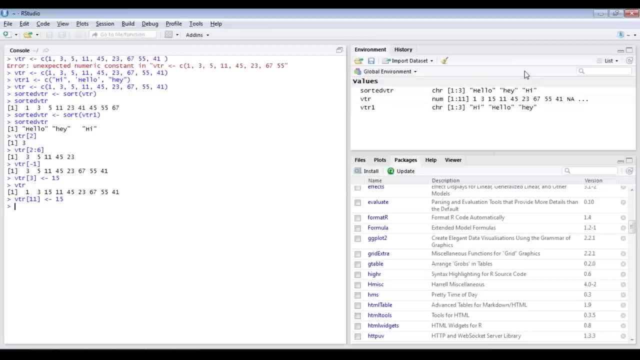 So let's try that first. Okay, it's got successfully executed. Now let me just see what my vector looks like after inserting to the 11th position. So you can see here: it has been inserted into the 11th position, leaving a blank at the. 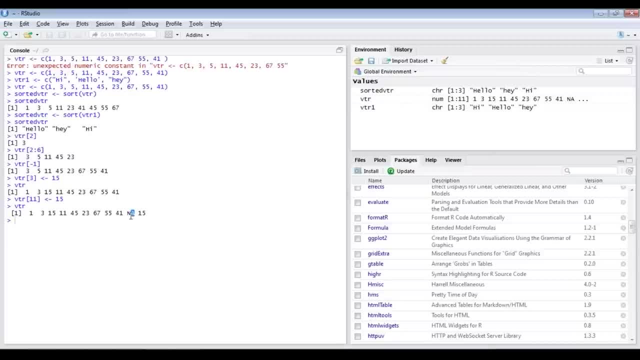 10th position. That's the reason you're getting not applicable NA here. Okay, so if you are adding a value to the index beyond the range with respect to some gap- now I had nine, I'm leaving a gap, I'm putting 11, then all the values between that. 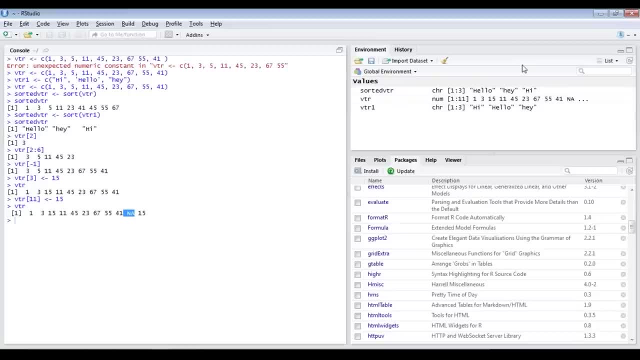 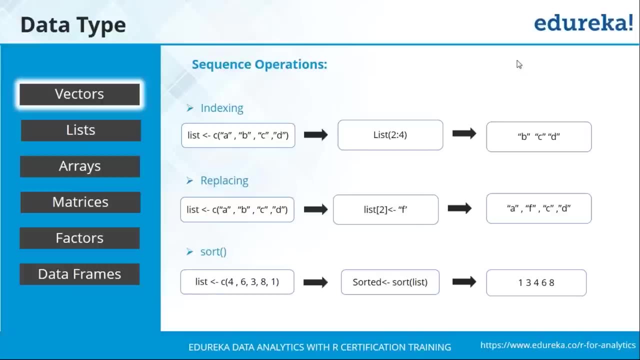 range becomes not applicable, But your value will get inserted into that position. So with this, we've come to a conclusion with respect to vectors. Are you guys clear? Any doubts still here? Any doubts with respect to vectors? Okay, so with that we've actually come to an end with dealing with vectors. 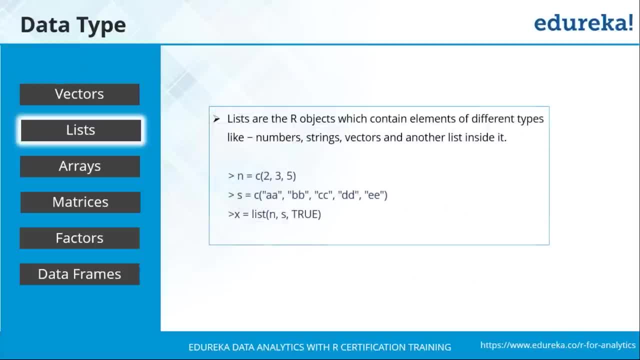 So let's move forward and talk about lists. Now, lists are basically R objects that contain elements of different data types. Now again, so you can have strings, you can have integers, numerical values, Boolean values, all that So you can have any number of elements. 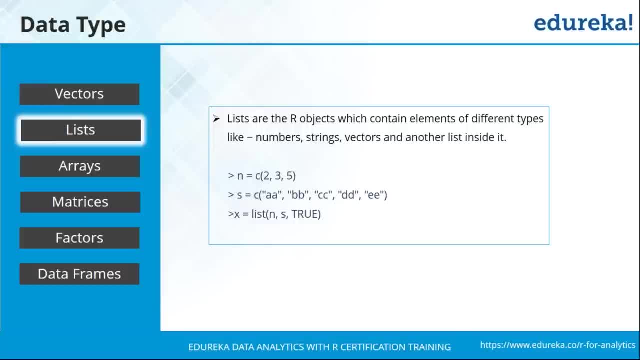 So that's how it is slightly different. with respect to vectors, It's the same thing, but it is just different with respect to what kind of data types that you can store In vectors. we had seen that you can only store one kind of data types, but in lists 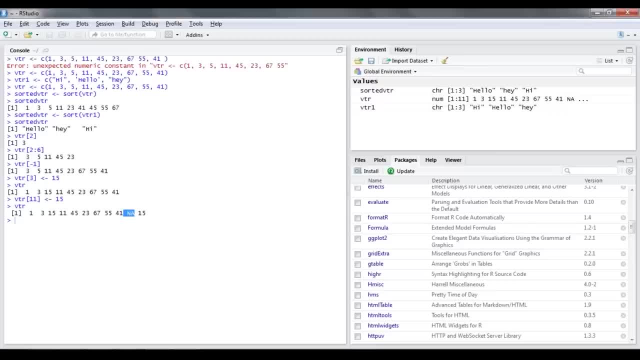 you can store different data types. Let me just show you how to do that, Okay. so before that, let me just show you how vector converts your data if it's of different data types. So let's say, vector two- okay- is going to store high. 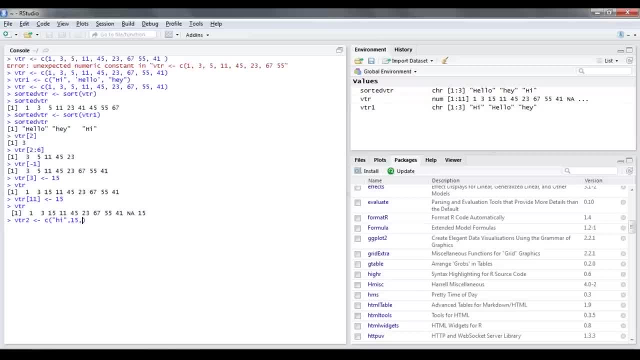 Again, it's going to store a numerical value of 15,. I'll give an integer value of 21. And finally, I'll add in true as well. So with this, I'm going to save it and it saves it. 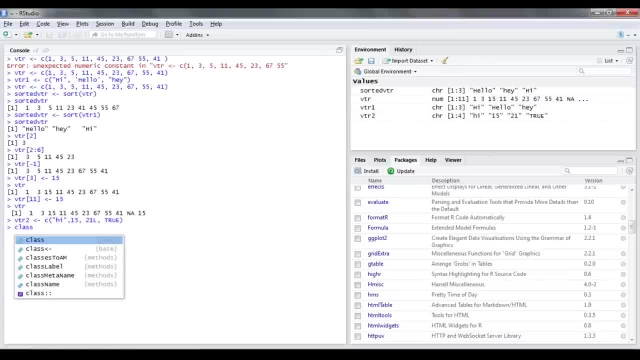 But what data type is it storing? Now, to find that, let's say, class of class is a function that helps you identify which class each variable belongs to. Okay, so vector two is the variable which I had stored. different kinds of data types. 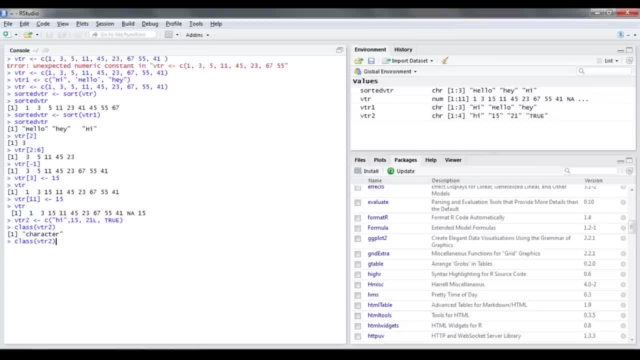 in And if I say enter, it tells me it belongs to character class. What does this mean? It basically means that all the values in vector two have been converted as characters. So you can see every value: high, 15,, 21, and true are in quotes. 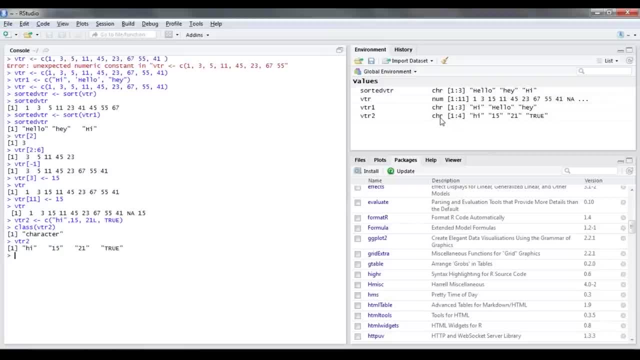 That means each one of these are characters. You can also verify that in your variable environment. So you can see this vector is basically of a character type and every value is being stored as a character. okay, So same time, let me create a new list that's going to store different kinds of values. 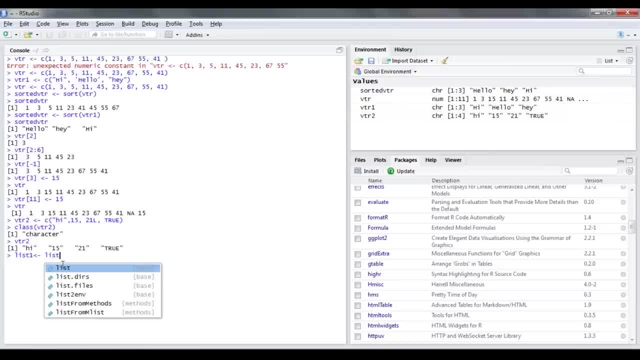 So let's say list one, And here you need to specify the type. So list of: okay, let's say hey is going there. I'll add false as well. I'll add 54, and 35 as integer. Now, if you save this, there's no error here. but let's see what is present in list one. 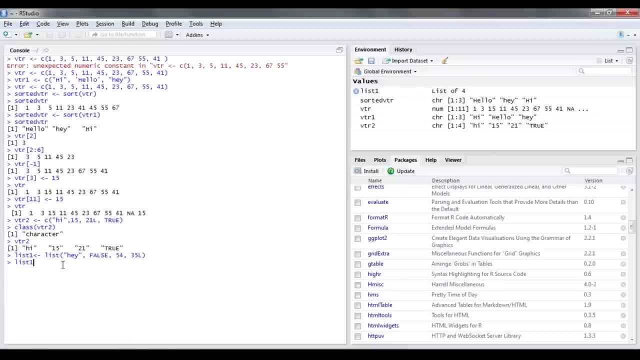 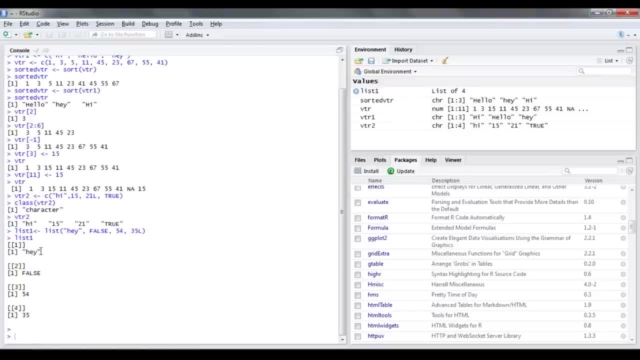 whether they're being converted to character or not. So you can see here each of them are being stored as their original data type List: 54 is being stored as character, false is set as false. 54 is 54, and 35 is set as 35.. 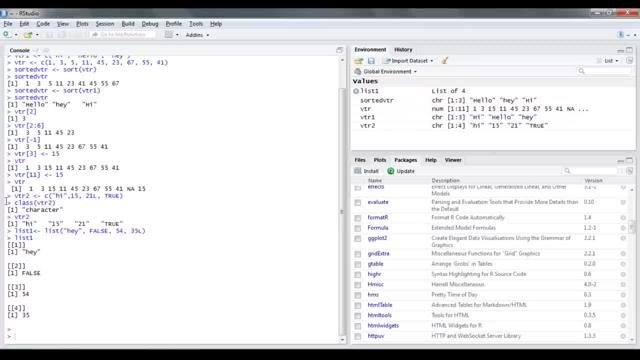 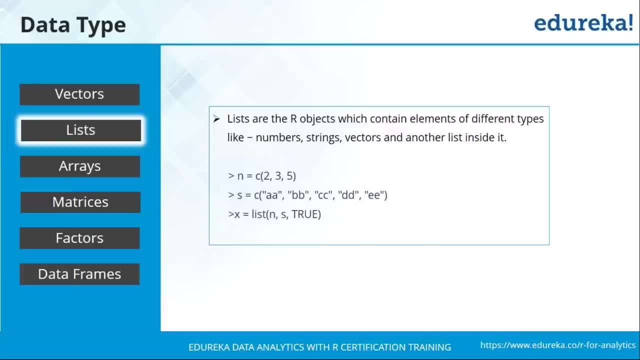 So here each of them retain their original data type, but whereas in vectors they get converted to character data types. So are you guys clear with this Right, So you can perform the same set of operations that you had performed with vectors as well? 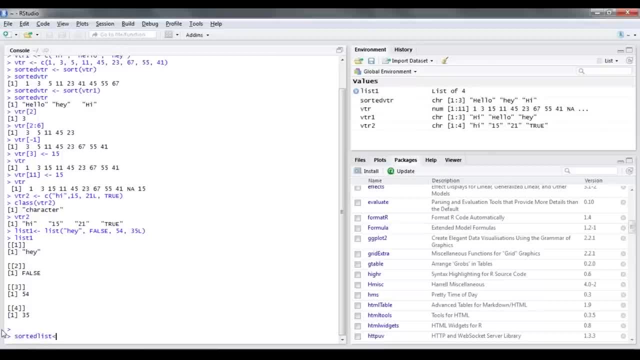 but one thing that differs is: let's say I'm going to create a sorted list for my list. So here I'm going to say list one, and who can tell me what is going to be the output of this? First, tell me whether this command will get executed or not. 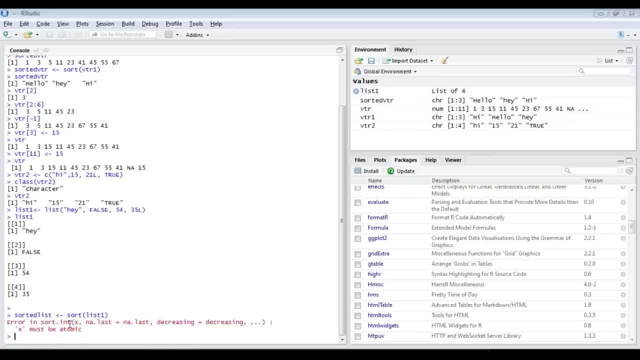 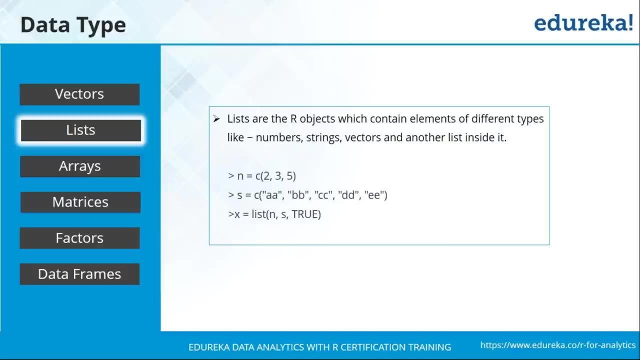 Okay, let's go ahead and try it. It says it cannot Because, again, what happens is, since you have different data types present here, it becomes hard for R to identify on what parameter it needs to sort out this data. Okay, let me just clear this workspace. 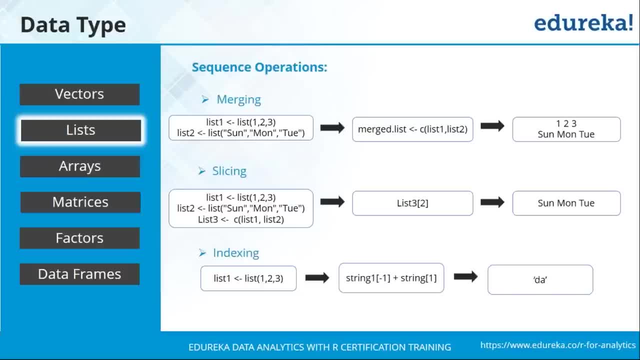 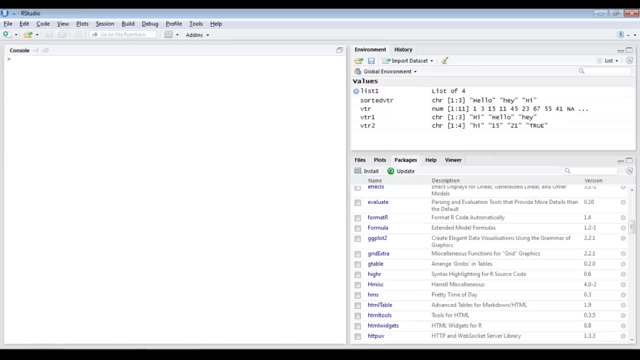 So, apart from the operations that we had seen earlier with the list, These are some of the specific operators here as well. So let's say you want to merge two lists. Now these two lists can be of any type. So I have list one, let me create list two that is going to have a combination of both. 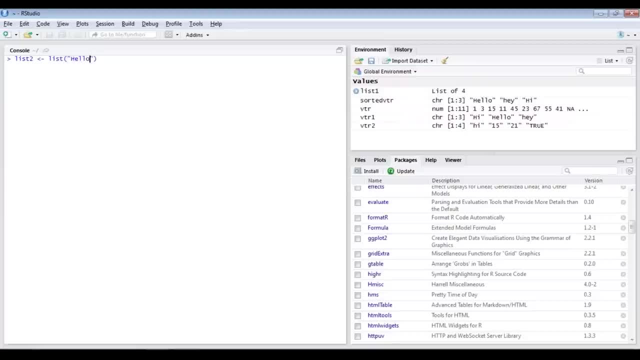 characters and numerical values. I'll say hello. I'll add a new. put an R as well. I'll add 45.. Okay, 45 and 28.. So this is a list that contains both character and numerical value. Now let's say I want to create a new list that is most of my list one and list two. 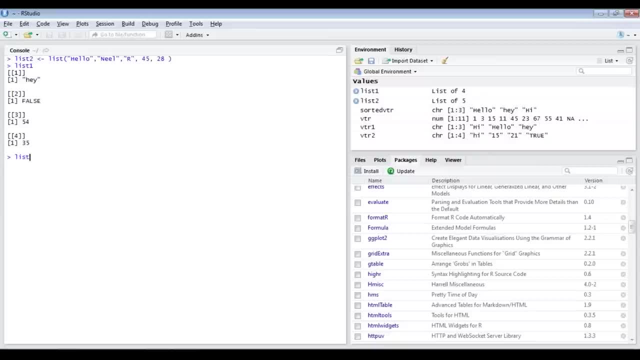 So, before that, let me just show you list one. This is what my list one looks like, and this is how my list two looks like. So I want to merge these two data. So, for that, what I'm going to do is I'm going to create a new list three. okay, in which? 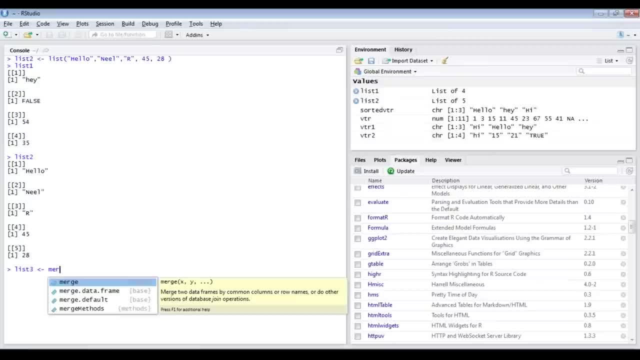 I'm going to merge this Now. to do that you need to use this function Merge, and here you can pass list one from a list two And you can see if you print list three. then you can find a merge list with respect to. 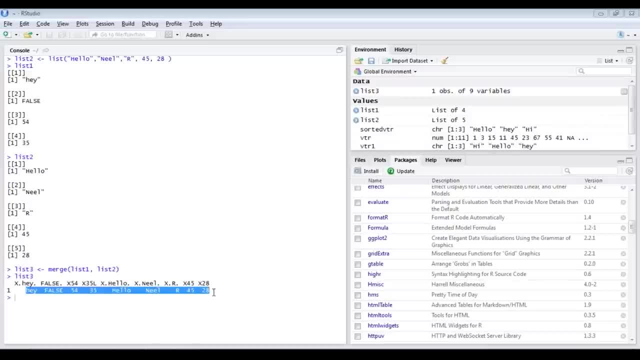 both of them. Okay. So here you can see: all the elements of that list have been merged to a single element. So you can see: hey, false, 54, 35 from my first list, and then, hello, Neil, R 45 and. 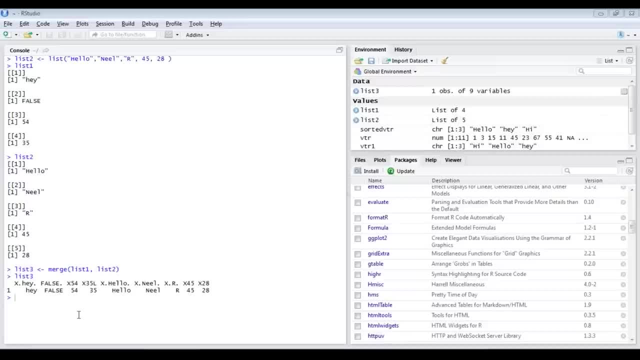 28 from my second list. So these two have been merged to a single list. So any doubts with respect to merging lists? Okay Now, apart from this, another way that you can combine these two is basically using them with respect when they're declared itself. 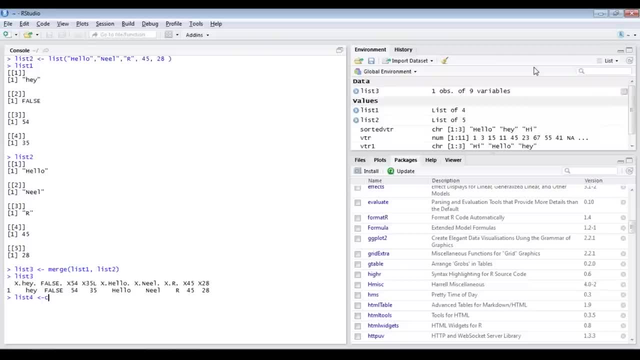 So let's say four is equal to a combination of both my list one and list two. Okay, now if I print list four, you can see the elements present here. But let's say I just want certain elements from my list four, then what I can do is I: 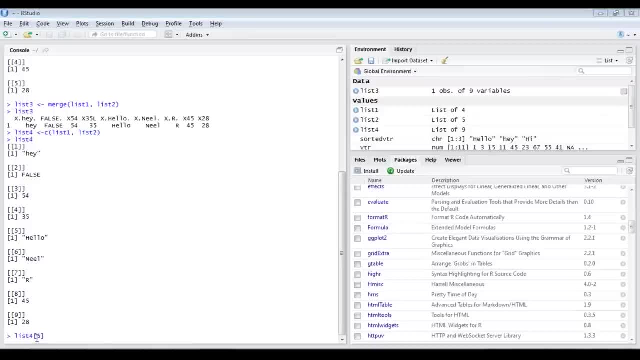 can use an indexing parameter here. Now, if I say five here basically extracts hello. So one, two, three, four, five here. So this is basically extracting an element from a list. So I hope you guys are clear with list. 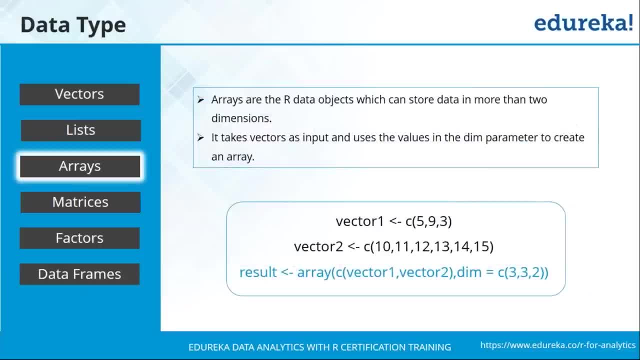 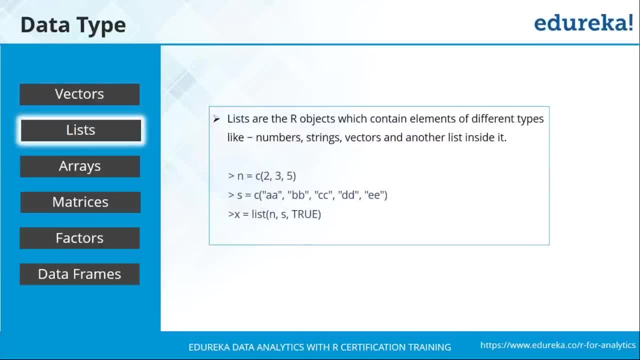 So let's move forward to the next data type, that is, arrays. So now, after vectors, comes list. Now, with respect to list, they're basically similar to your vectors, But the only key difference, being with respect to vectors, is that they can store elements. 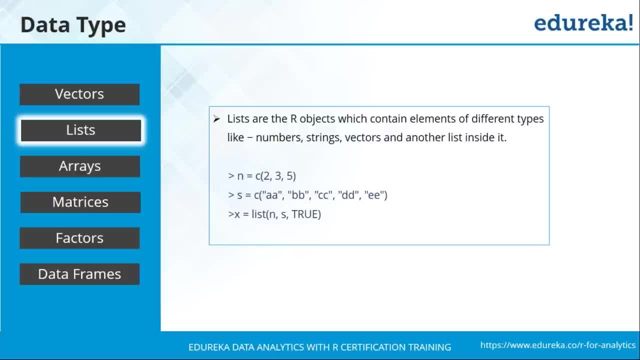 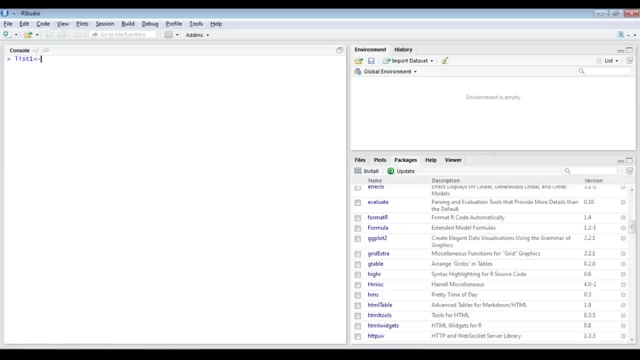 They belong to different data types itself. So let me go ahead and show you on our studio itself. So I'll begin by creating two vectors, itself called list. one, okay, which is going to store numerical values, Let's say one, five, seven, 13, and 15,. okay, eight comma, sorry about that, okay. 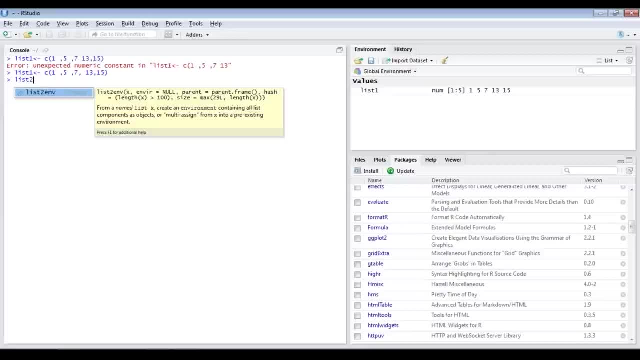 So I'll go ahead and create another list, say call it list two, okay, and this is going to have character elements. So let's say I'll give it colors, say red, blue and green. okay, So these are the elements of my list. 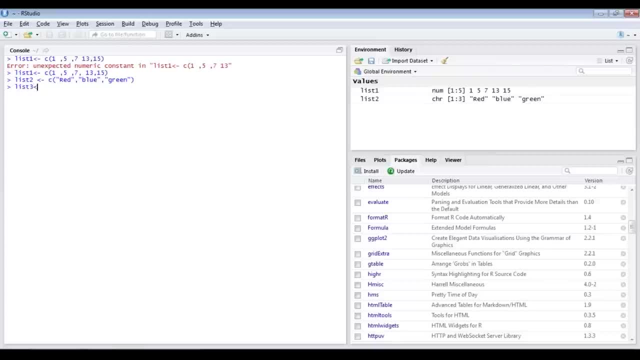 Now, what I'm going to do is I'm going to create something known as list three, which is going to store both of these. Now, these are basically vectors. okay, So if I directly write list three equal to C of list two, one comma, list two, then what? 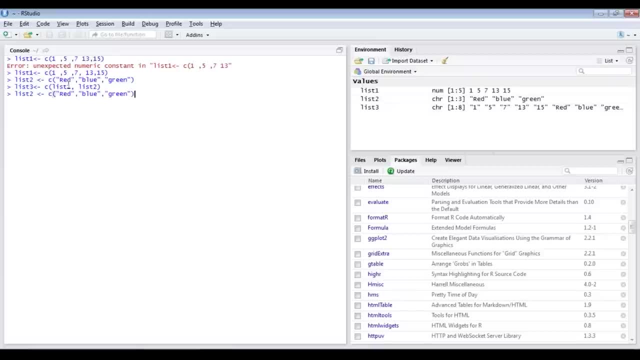 happens is It gets created. but when I print list three, okay, all the elements of my list are considered to be characters because, again, here it's just a vector that's being called list. To convert this to an actual list, what you can do is here you need to first change it. 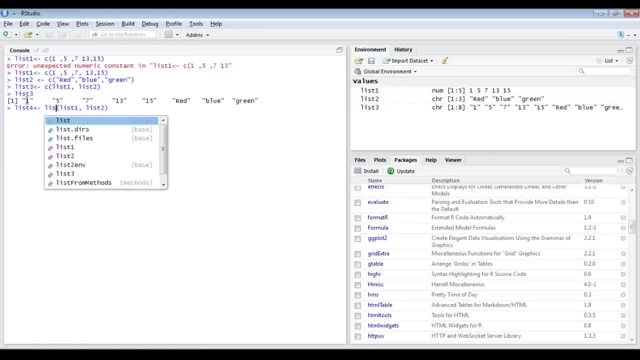 and rename it as list four and you need to specify: this is of a type list. Now, when you do that, automatically R understands that list four is going to be of type list and then, if you create this, Let's try printing here: 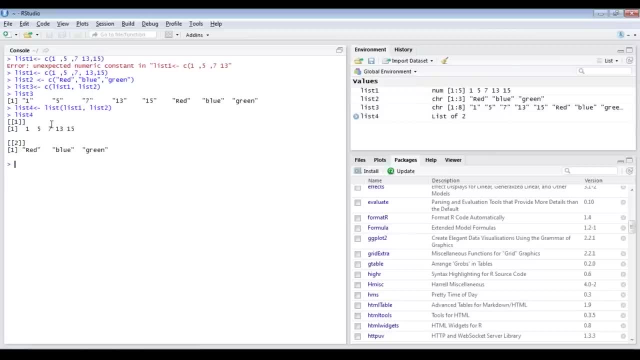 List four. So here you can see both the lists. One is completely retaining its numerical elements and two is completely having characters. They are not being converted completely, as we had seen with vectors. Similarly, if you create list five which has a combination of all these elements, let's 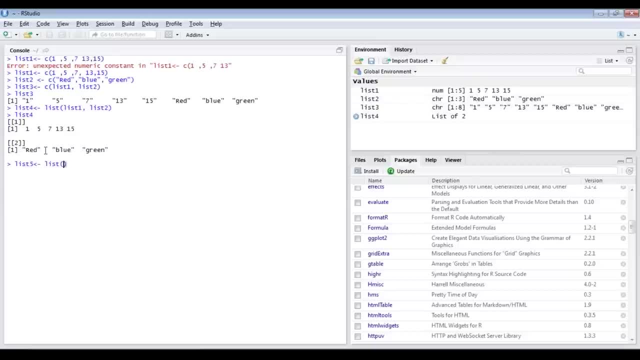 say list, and here I'm going to add 35, 49L, then I'll put in true and I'll add Neil. Okay, So I'm taking four atomic data types and I'm creating list five. When I print list five, you can see here each one is actually retaining its original data. 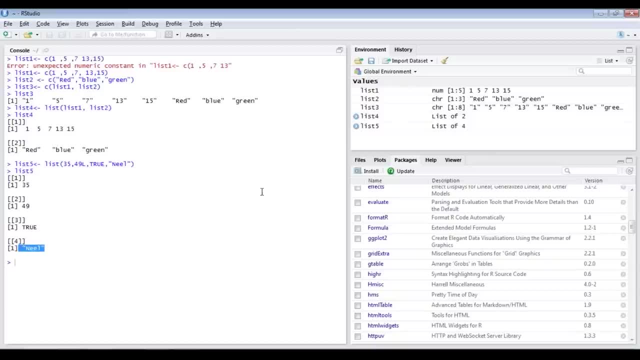 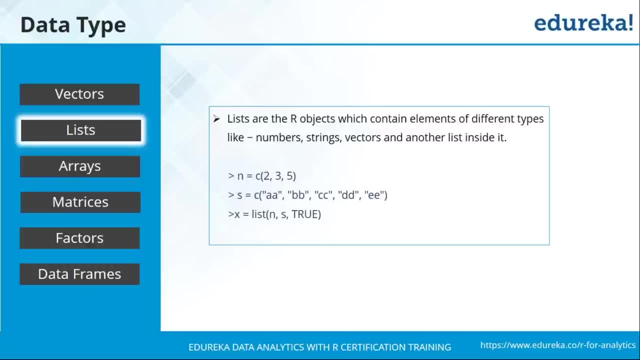 type and they're not getting converted to character, as we had seen with vector. So list can help your objects retain their original data types. So are you guys clear with this and the difference between lists and vectors? Okay, Now, apart from the operations that you had seen earlier, there are certain operations. 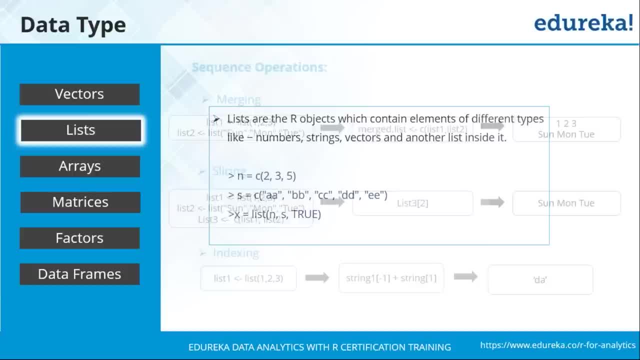 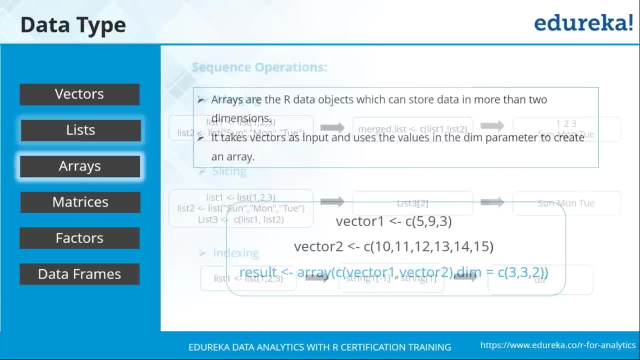 that we have already seen. Now again, you can merge to list as well as you can perform slicing, Okay, Apart from that, you can standardly perform your indexing as well as slicing, So that's something that you can definitely try out. 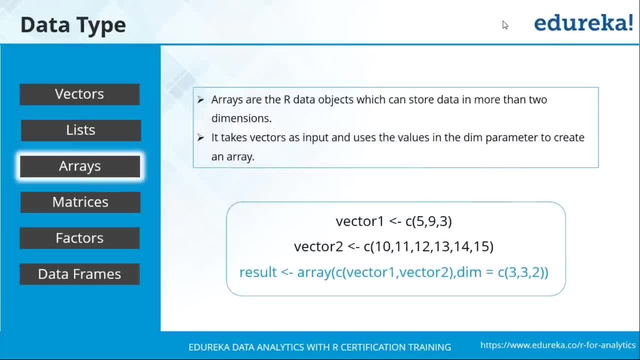 Now coming to the next data type is arrays. Now, basically, the purpose of arrays in R is to store your data in more than two dimensions. Okay, To store it in two dimensions. you have matrices, but we'll talk about that in the next part. 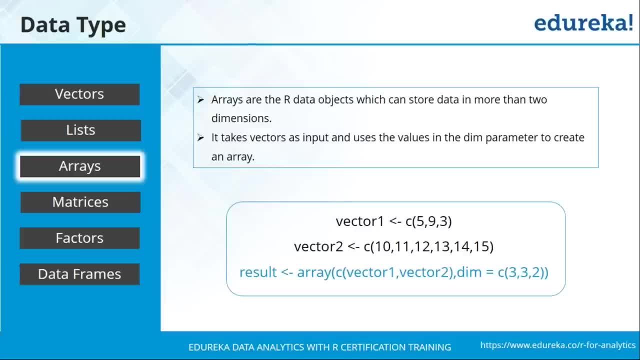 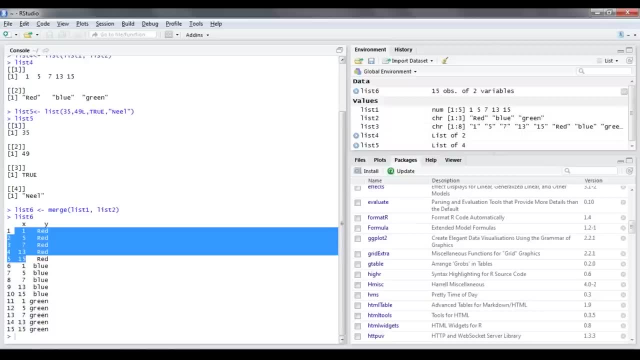 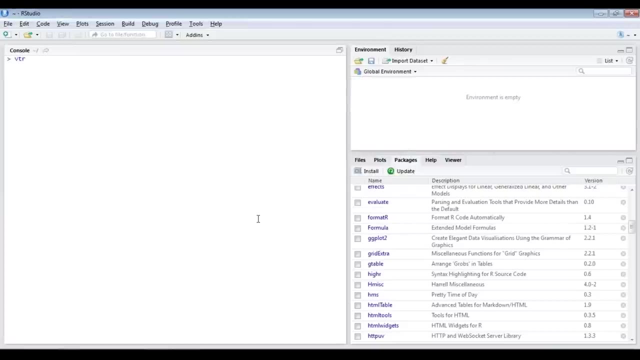 But basically, what you need to understand is that array helps you store data in more than two dimensions, and it usually takes vectors as input parameters. Okay, Now, what I'll do is let me just clear all this. So, talking about arrays, basically I'm going to create two vectors here. 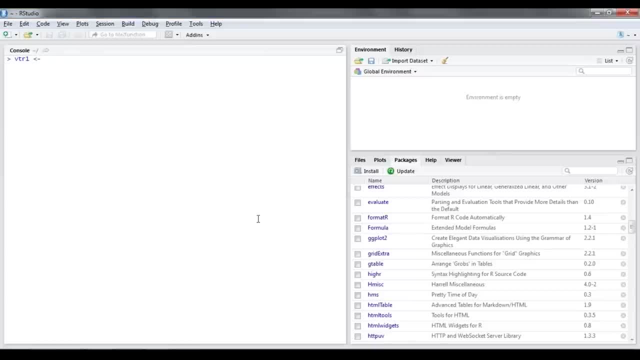 Vector one which basically is going to have five numerical values. So here I'm going to have values two, then I have six, I'll add 14. So basically certain random numbers, itself, then 22. So five values present in my first vector. 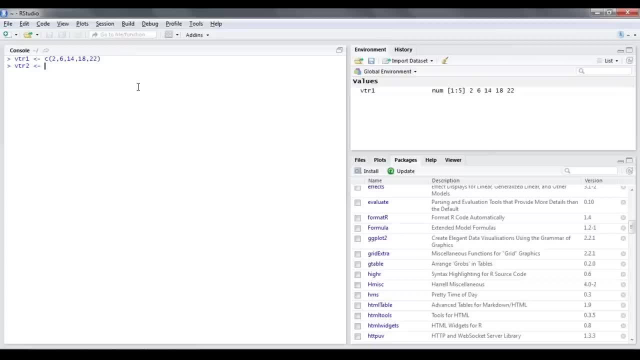 Okay, Vector two, in which, let's say, I have five, I have 15,, 25,, 45,, 65,, 85,, 105, and 125.. So basically, I have two vectors present here. One has five elements, the other has eight elements. 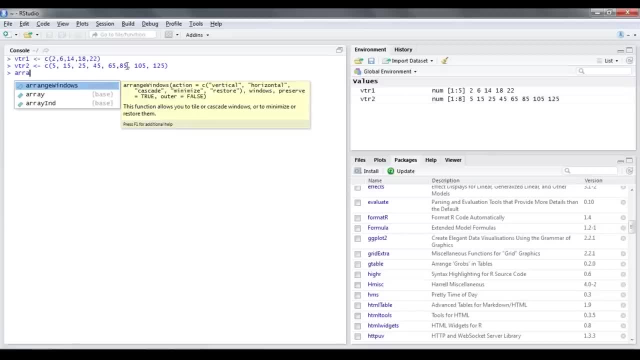 Okay, Now to create an array. what I can do is I can say arr, let me just call it my array, arr. Then, following that, I need to specify the array type. So, basically, this is my array type, and then I need to provide it an input. 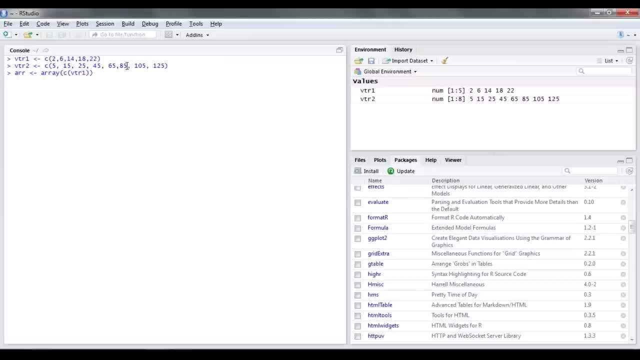 So let's say C of vector one. So now what I'll do is now I've just created a single dimensional array. Let me just show you how the array looks like. So if I just print arr. so this is how my single dimensional array looks like. 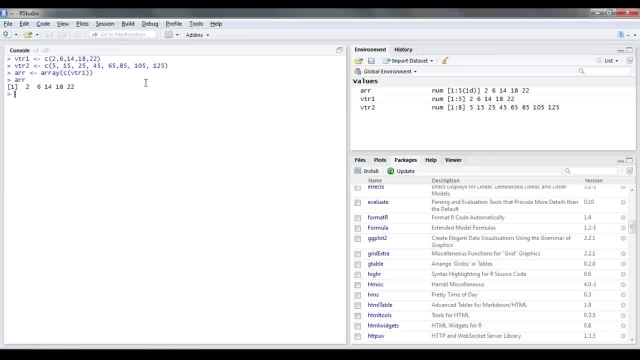 Now, the purpose of array is to create it as multi-dimensional, So let me just show you how it's done. Okay, So what I'm going to do is I'm going to make a multi-dimensional array here, So I'll just call it array two. 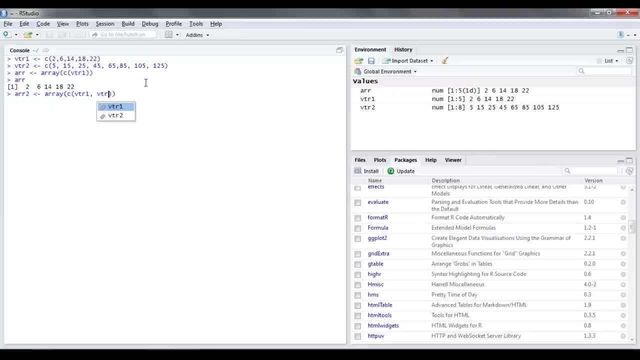 And instead of just passing vector one, I'll pass vector two as well. Now, apart from this, I'm going to specify the dimension how it has to be. So I'm going to slightly change the dimension here. So to do that, just use dime. 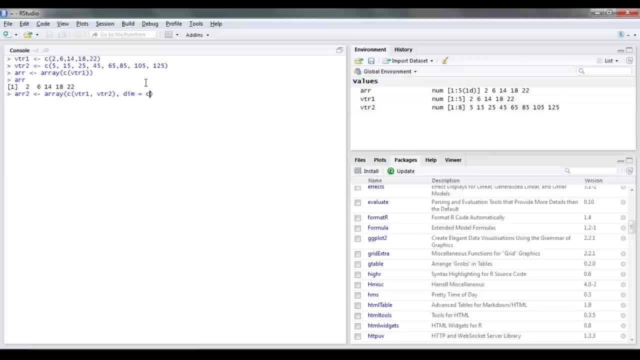 Again. dime, basically, is supposed to set the length, and here I'll pass a vector which tells how the dimension should be. I want to have five elements in my first row, five elements in my second and three elements in my third. So this is basically how I'm going to define it. 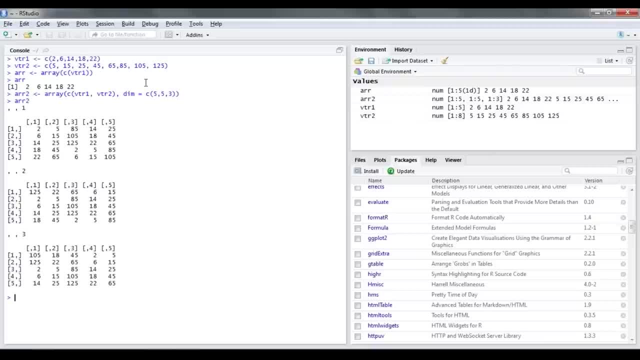 Once I've done this and if I print arr two so you can see how my matrix looks like. So if you see the values here, it may look slightly jumbled, So let me just help you understand this better Now. I've taken first five values from vector one and then I've stored it in my first column. 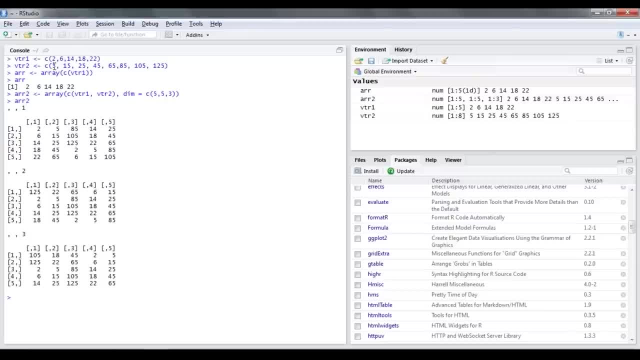 So if you see that they've been stored correctly, Then what happens is in my second column I'm taking continuous values. So five- 15,, 25,, 45, and 65- have been stored. So that is my limit. 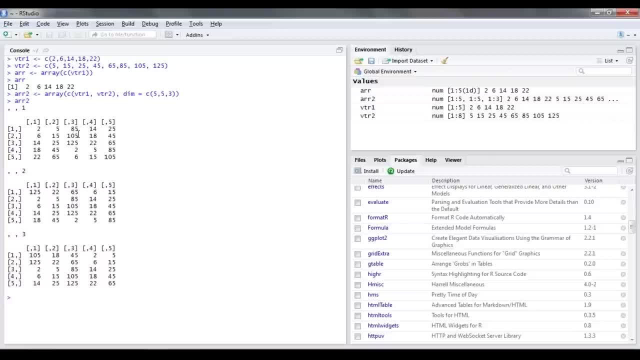 The values following that will start from the next column. Okay, So again, 85,, 105, and 125.. I'm at end here, But again, since I have to store the values continuously, again you're starting from two, six, 14,, 18,, 22, and again you're starting from that next list. 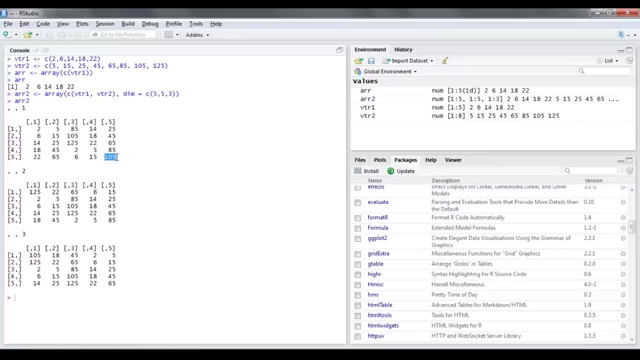 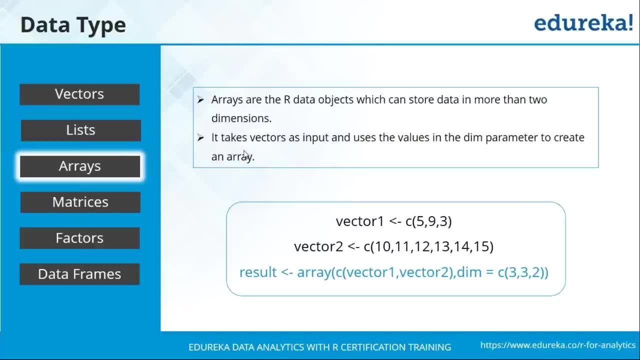 Since there are three copies being created, the order continues where it stops at 105,. you're starting with 125 in the next one. So I hope you guys are clear with respect to how our data is being stored in an array in R. So any doubts with respect to arrays or lists? 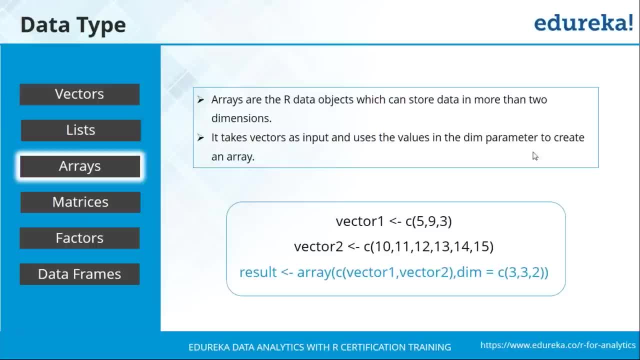 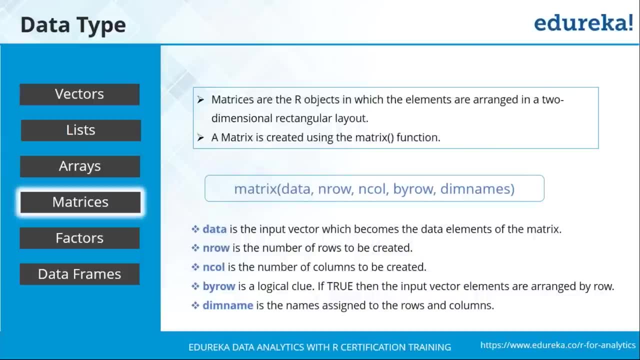 Okay, it's great to see that you guys are following. Now, apart from arrays, comes your matrices. Now, matrices are quite similar to your arrays itself, but only difference with respect to your matrix to arrays is that it's not a multi-dimensional, it is just two-dimensional rectangle. 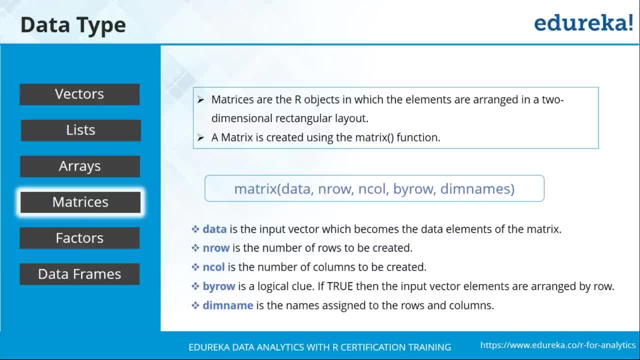 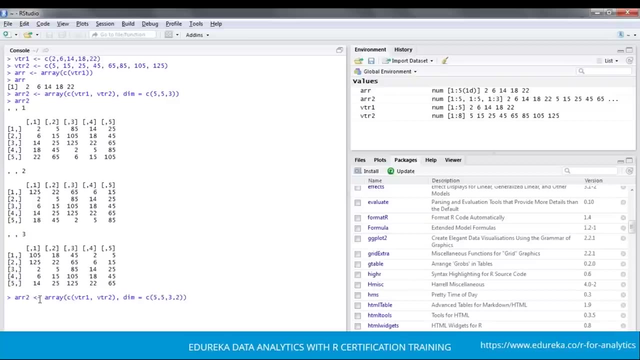 So there you had seen, we had created a combination of a matrix of five cross five and we had created three of them in a single array. Now, if you go back to that, let me just show you another feature there. Okay, Now here let's say I'm going to add another value, let's say two, and I'll call it array. 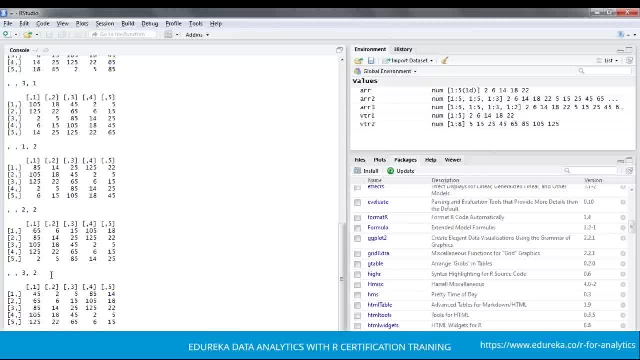 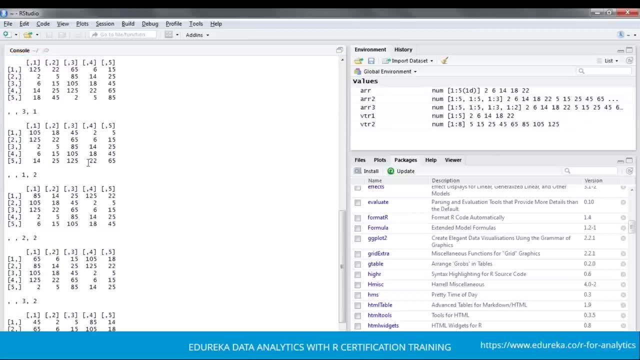 three, And if I print array three, then you can see it is storing it into a multi-dimensional form. So I have a matrix here which is again in turn getting stored inside another matrix. So you can see, these are the first three rows for the first column. 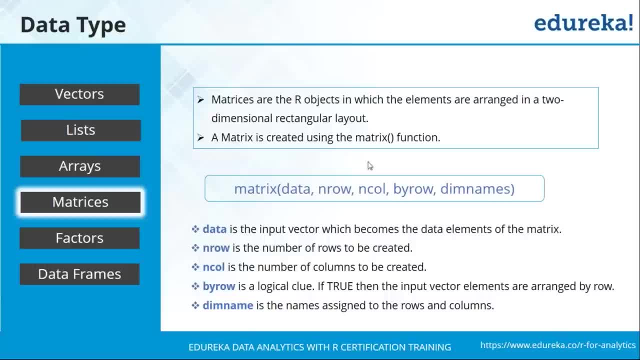 These are the next three rows for the second column. Okay, So it's a combination of multi-dimensional elements here, But when you talk about a matrix, It basically is used to store elements into a two-dimensional format. It's quite simple and is more of the basic fundamental here. 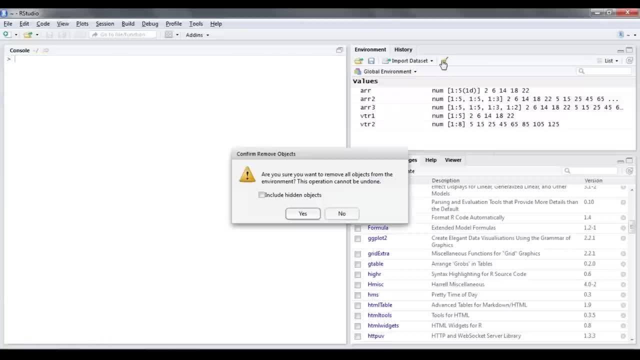 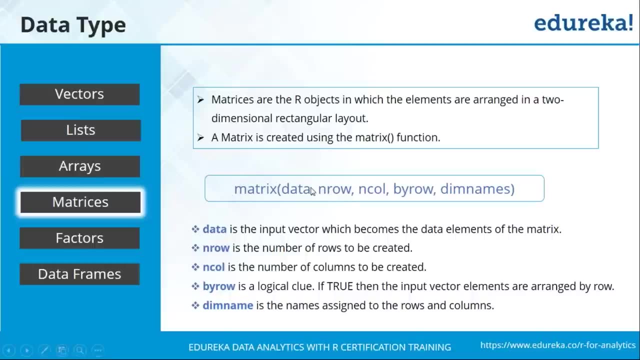 Okay, So let me just clear all this and clear the variables as well. Now the syntax for creating a matrix is quite straightforward. You specify the keyword matrix, followed by the data that you need to pass- It could be multiple vectors together- and then you specify the number of rows: number. 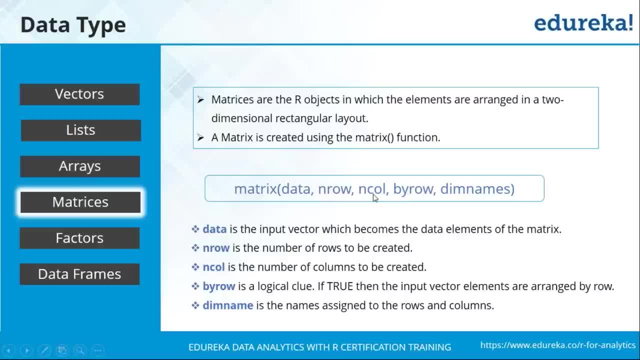 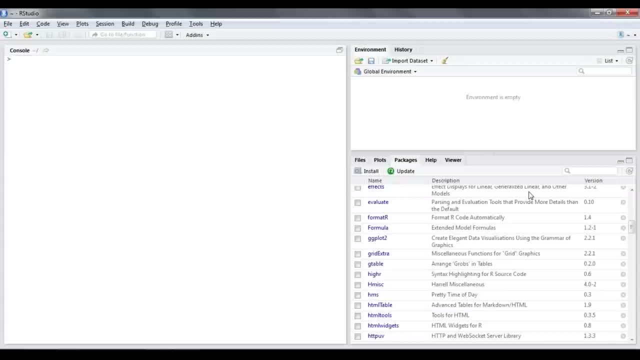 of columns By row. basically is a logic by which your row elements have to be arranged, But for now, don't worry about that- and dimension names. So let's go back to RStudio and try it out. I'm going to create two vectors again. vector okay. let me just take the previous states. 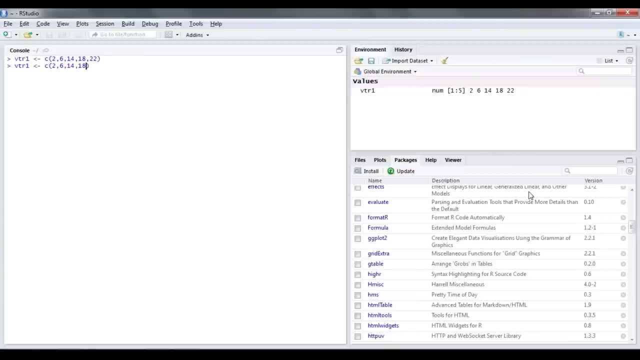 So I'm going to take the same vector and I'm going to modify this vector. Okay, so basically, I'm creating two vectors, vector one and vector two, having different values. Both have five elements presented. Now let me create a matrix- MTR- of the type matrix again. 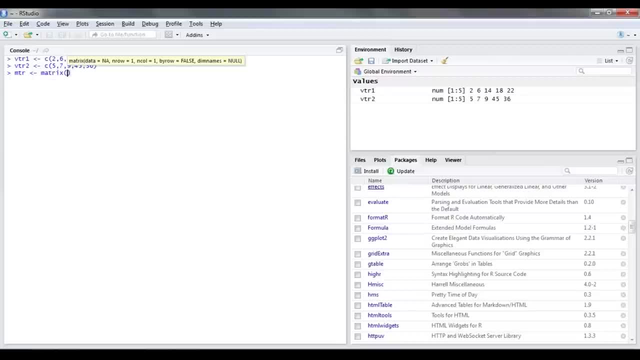 So when you type matrix- Okay, now again, there is a highlighted here- It helps you understand what should be the syntax for this function. So, as for the first part, that is, the data, I'm going to say vector, one comma, my vector. 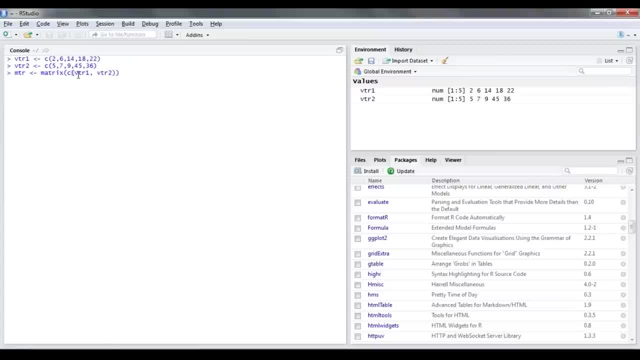 two, and then I need to specify the dimensions. Now I can either make it a five cross two or a two cross five element. Now, again, the filling of the elements starts column wise, So always the data will be filled down. So what I'm going to do is I'm going to make it a five cross five. 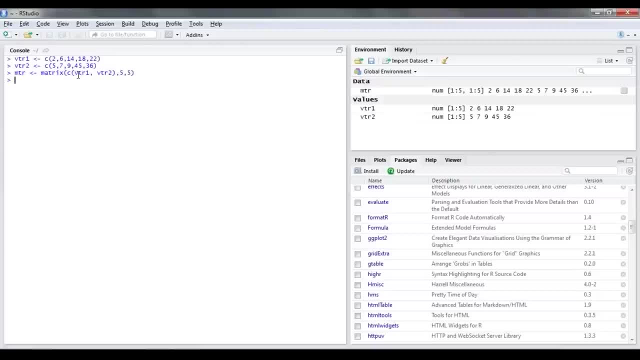 So number of rows is five, Number of columns is five. Okay, And when I hit enter a new matrix is created. But to see the data elements in the matrix, just type MTR and you can see the elements. So here, if you see, first vector is getting inserted into the first column completely. 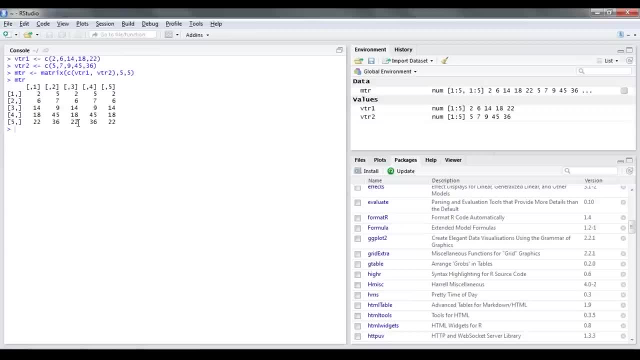 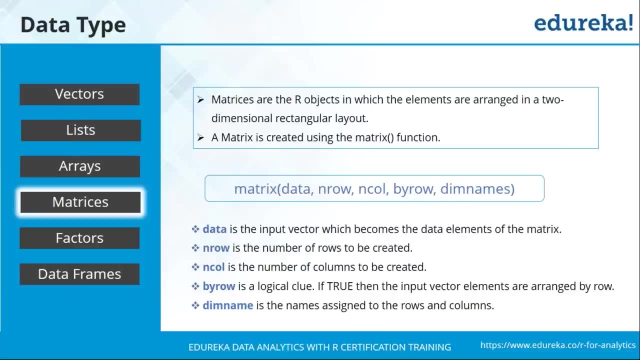 The second column is getting completely filled with the second vector, third column with the first vector, fourth column with the second vector and fifth column with the third vector. So always the data filling happens in a column, wise sequence. So any doubts with respect to vectors? 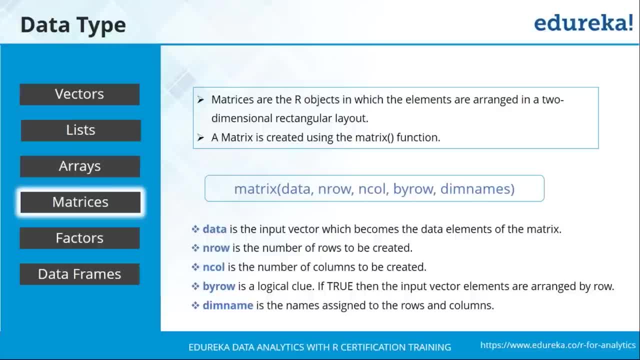 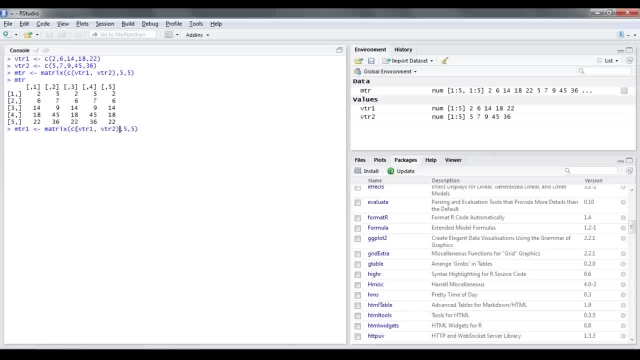 Okay. so Reshma is asking me: what happens if I give different values, Different dimension? Okay, definitely, Let me just show you that as well, Reshma. I'll just make it MTR one, Okay. And here what I'll do is I'll change it to, let's say, eight cross five, or let me just 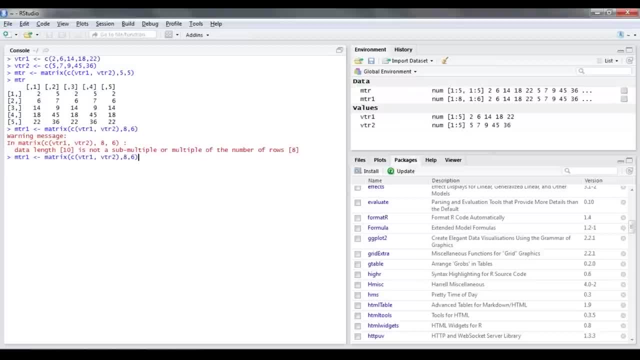 make it eight cross six, Okay, Okay. The problem with this, when I try with this, is that it goes beyond the range. Now I'll just change it to three cross four Again. that case it does not get created. So not all values come into the picture because it's not a sub multiple. 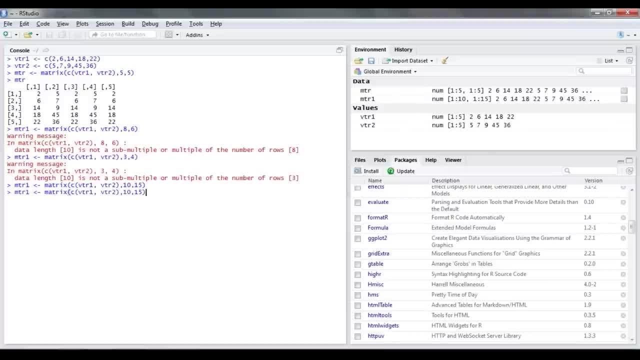 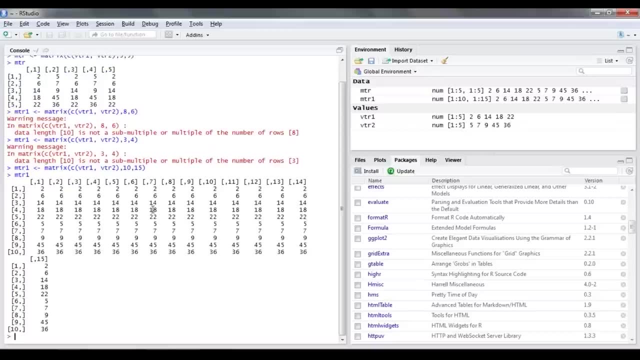 But let's say I'm going to make it 10 comma 15.. And it gets created because it's a complete multiple. Okay, so I'll just print my matrix one, So you can see here a 10 cross 15 matrix being created. 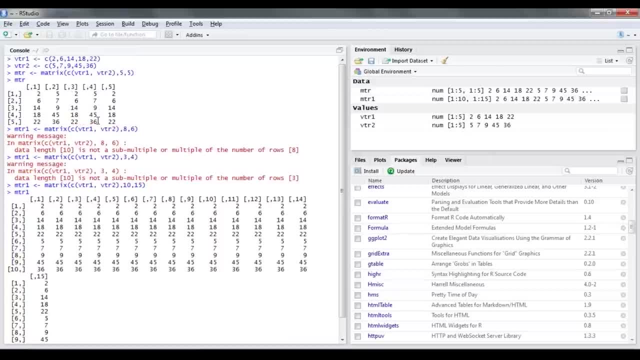 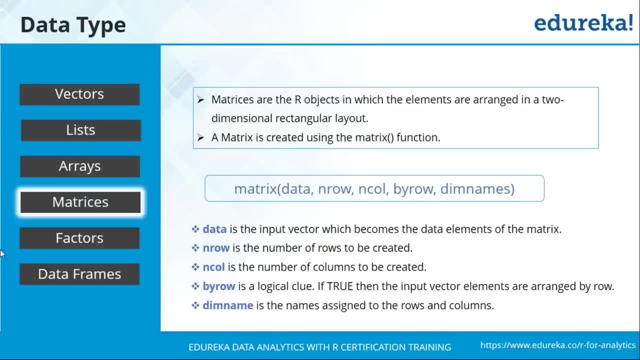 Okay, so it needs to be a multiple with respect to the original number of values present in that matrix. Is that clear, Reshma? what you need to do is, if you are creating a different dimension from the vectors that you have, then make sure your number of rows and columns are a multiple or a sub. 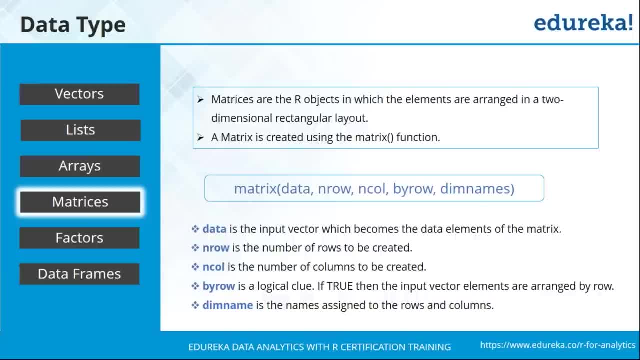 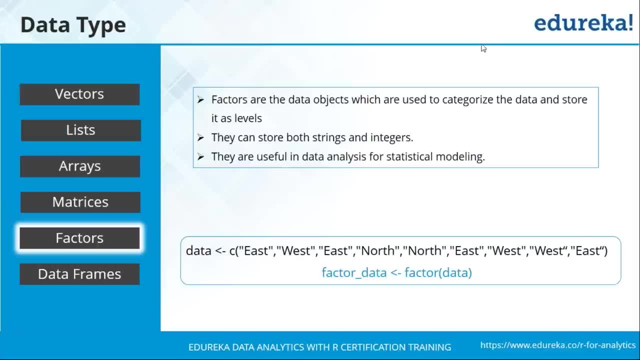 multiple of the number of elements present in that vector. Is that clear, Reshma? Okay, so moving forward, let's talk about the second last data type of today, That is, factors. Now, factors, basically, are something that are used to categorize the data into levels. 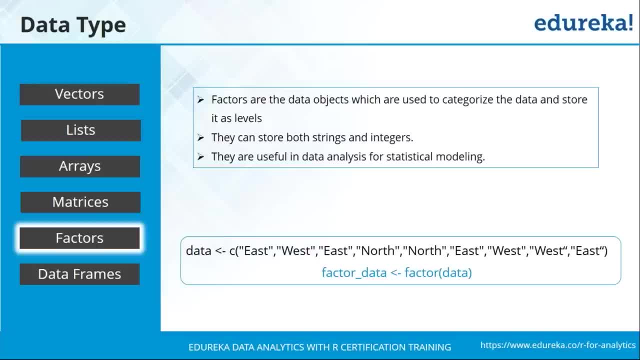 as such. Okay, now here you can use it to categorize both strings and characters, And, apart from that, this is something that you'll extensively be using when you're working with different statistical models. Now it's quite straightforward. Let me go back here. 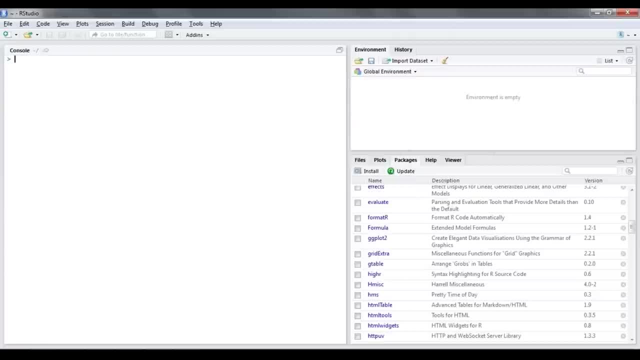 I'll just clear everything here And from here. okay, so let's begin by first creating a new vector. So I'll just say vt1.. And here let's put new values. Let's say 3, 5,, 7,, 11,, 5,, 15,, 11 again, 20,, 3.. 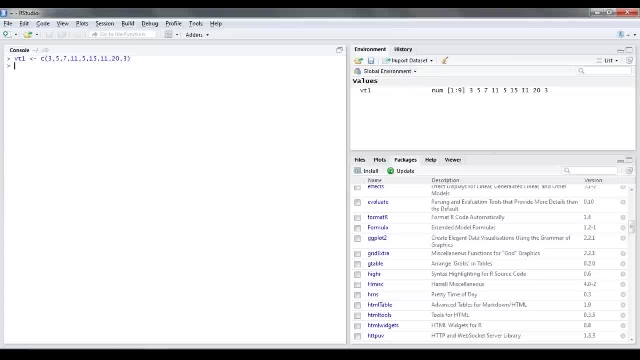 Okay, Once you hit it, a new vector is getting created. Now, what I'm going to do is: now I'm going to create a factor out of this vector. For that it's quite straightforward: I'm going to create a new factor. 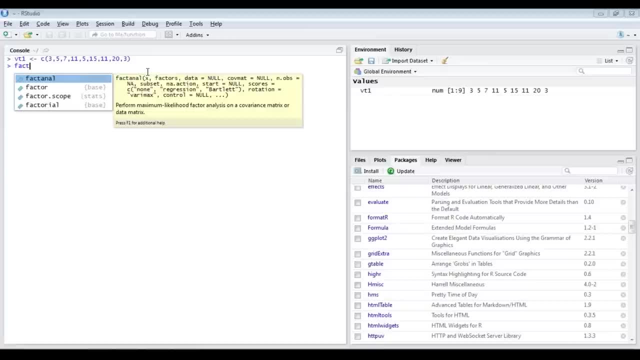 I'm going to create a new vector, So I'm going to use my factor variable, Fact VTR. Okay, On this, I'm going to convert factor And I'm going to pass the parameter of vector. Once I have created this, a new factor vector is created. 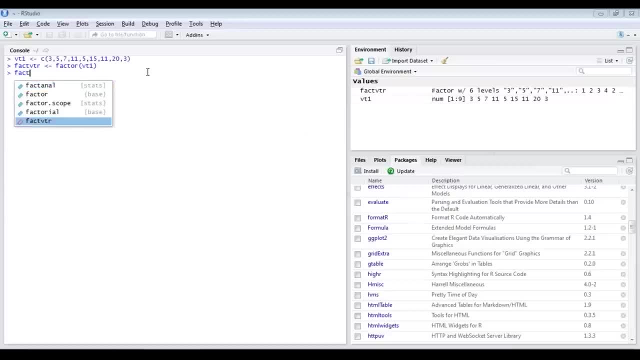 Okay, so to see what is the value inside factor vector, you can just print the variable So you can see here the different values that are present here, But their unique values are denoted by the levels. So this is something that will definitely come into use. 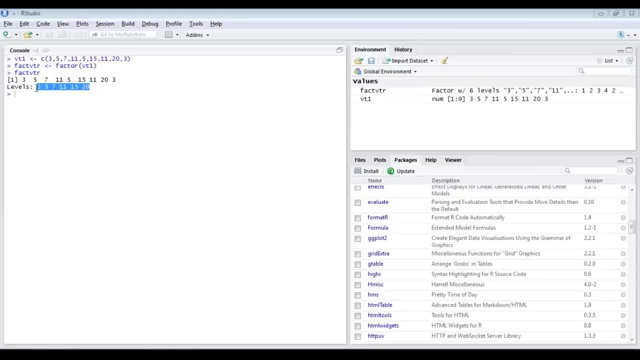 while you're working with statistical modeling, So there may be situations where you'll be seeing different values, but to understand the unique values, you can always convert those values into factors and check their corresponding levels. So it's a quite straightforward process. So let's say you're working with a data. 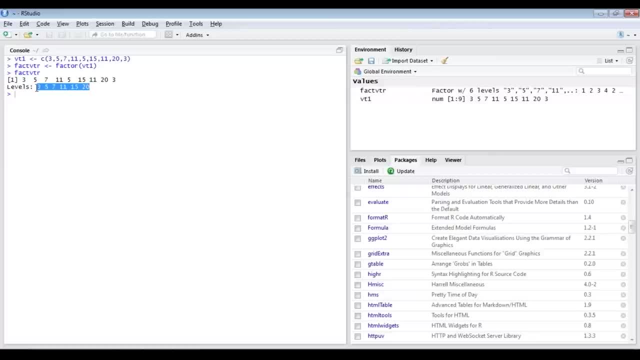 that has different probabilities. To understand the unique probabilities, you can always take that data and convert it to factors wherein you can identify the levels to identify what are the various possible probabilities that are present in that data. So are you guys clear with factors? 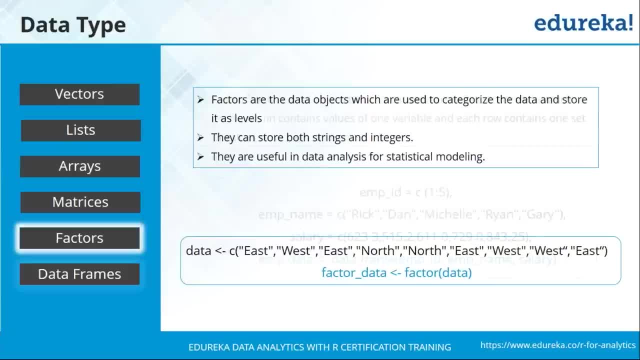 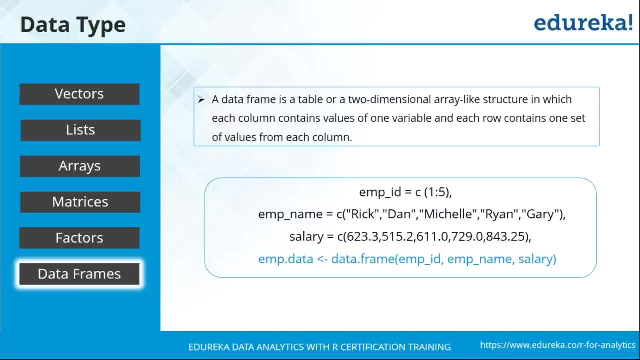 All right, that's great to hear. So, moving forward, let's talk about data frames. So data frames is something quite interesting that you'll be working with R and is one of the most widely used data types after vectors in R. Okay now, with respect to what exactly is a data frame? 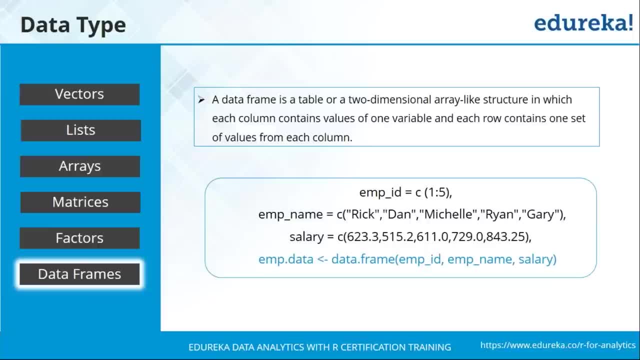 it could be a table, or it could even be a two-dimensional array-like structure. Okay now, in a data frame, each column actually contains a value from one variable and each row actually contains from one set of values from each of the columns. 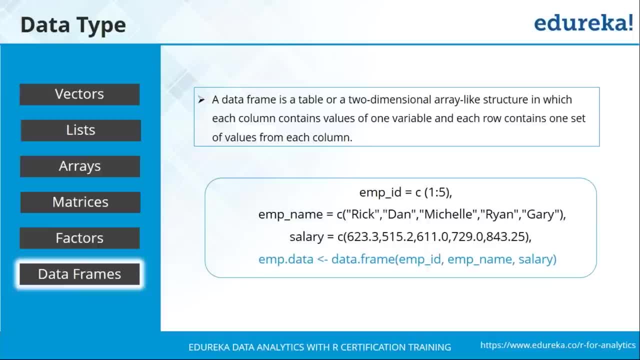 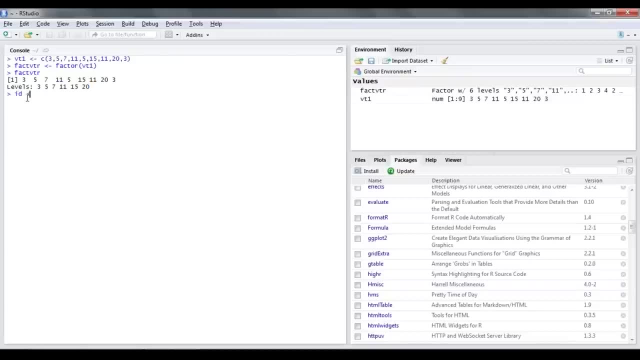 Now, rather than explaining this, let me just go ahead and show you how it works out. Okay, what I'm gonna create is: I'll create a new vector, let's say ID, and this is gonna store a range value from, let's say, 100 to 150. 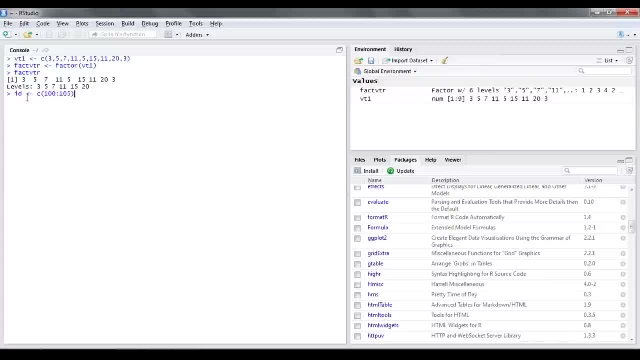 Or let's say I'll just take a smaller number, let's say 105.. So five numbers are gonna be inserted into ID. Apart from that, I'll say name. okay, Name is gonna have. let it have my name. 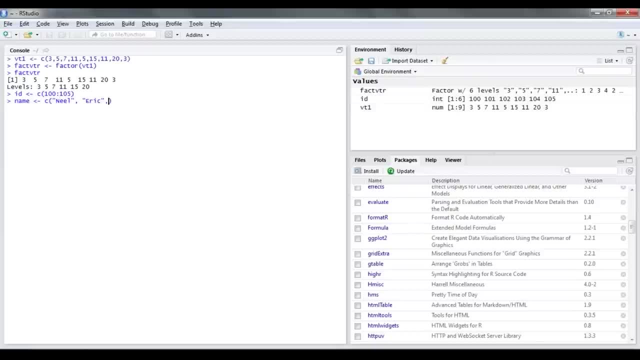 Okay, so I'll add in Eric's name as well. Then we have Dave as well. Okay, Dave, I hope you don't mind, you guys? Okay, not a problem. Then let me add Roshni as well, And let me bring in Pankaj. 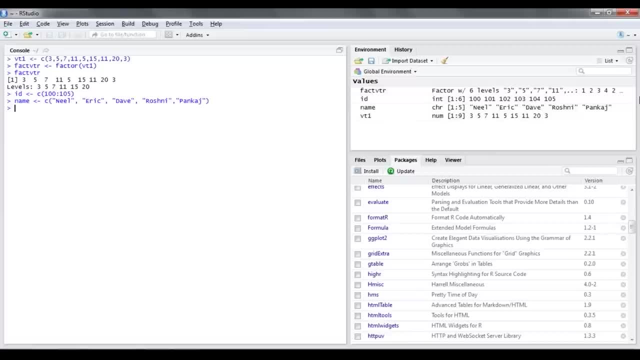 Okay, so these are the five names. Now, what I'm gonna do is I'm gonna create a data frame that combines these two vectors. Now how do I do that? Let's say I'm gonna call it class std. okay, That means it's just a single name, okay. 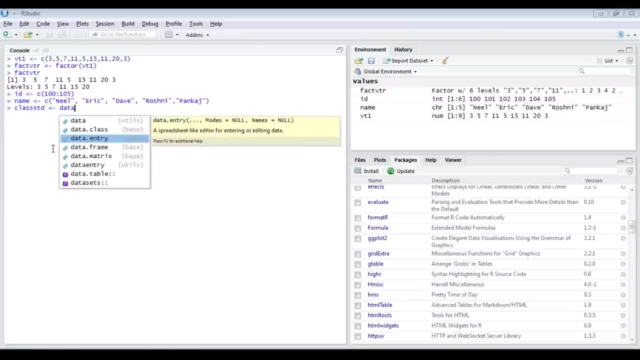 Now this is gonna take a data frame- dataframe- and here I need to pass the values, So ID name. Once I do this, it gets created and let's see. Okay, so this is problem because there's a difference. 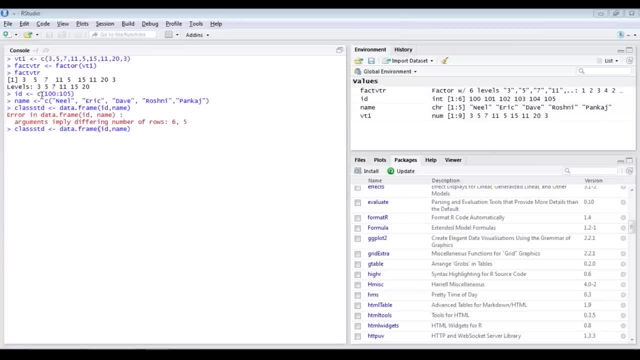 with respect to the number of elements between both. Now, here, if you see, ID has six elements, whereas name, okay, ID has only five elements. So in that case, what I'll do is I'll just go back to my name. I'll just clear all this. 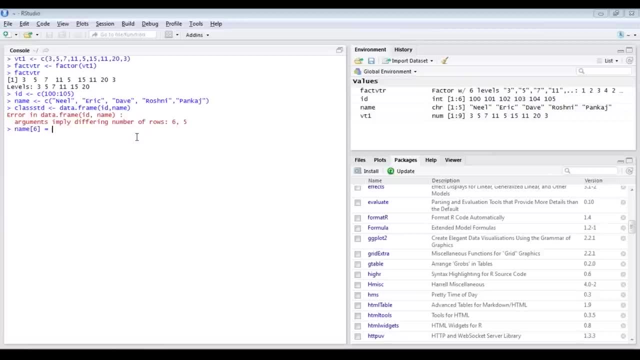 So I'll say: name of six is equal to Reshma. okay, So now I have six elements. Now if I try the same, it gets created. And if I print this, let's see how the output looks like. So here you can see they are getting linked together. 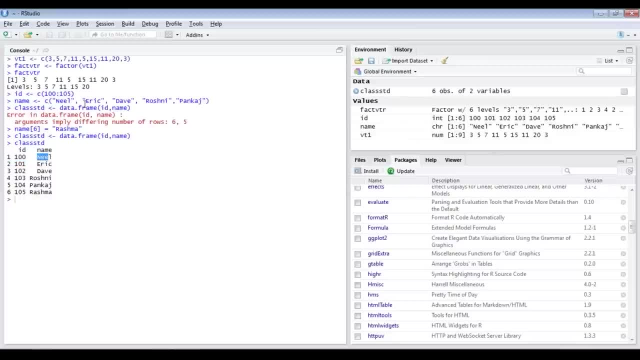 Each ID is getting a corresponding value from the name. Okay. Now similarly, let's say: you have another field, let's say marks. okay, Please don't mind this, And I'll say 80,, 85,, 87,, 95,, 92, and 89. 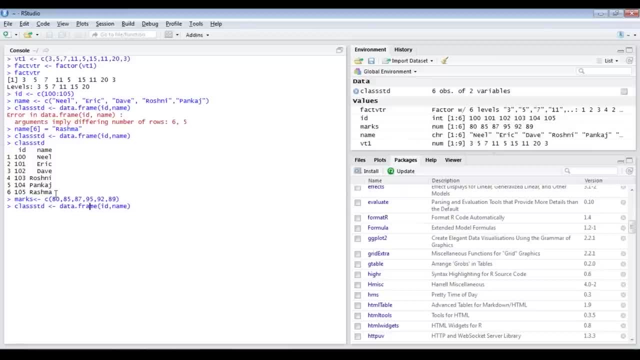 Okay, so six values. Now I'm gonna create another new data frame, std1,, and here, similarly, I'll pass the third vector, that is, marks. Now, if I print the class std1 data frame, then you can see correspondingly each row. 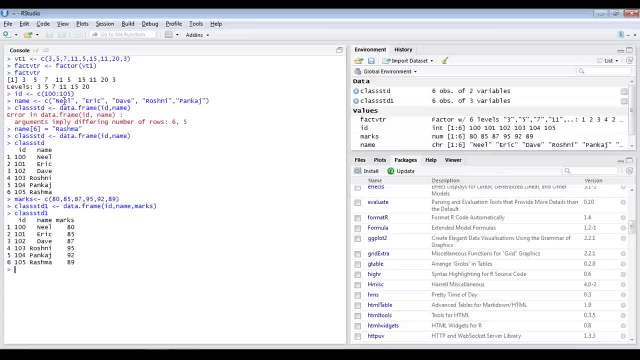 has a value from each of the vectors. That is, one element is getting picked from each of the vectors and, correspondingly, they are being linked and put in a row. So any doubts with respect to how a data frame looks like and how a data frame works. 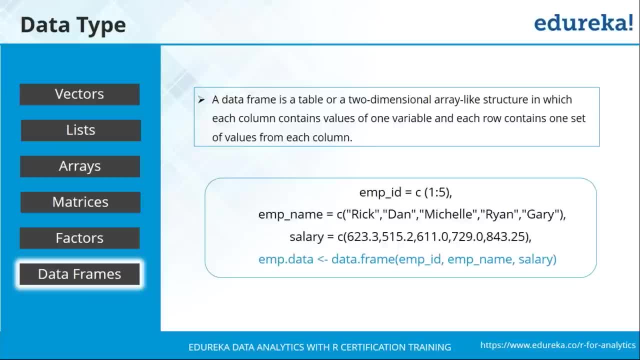 So a data frame is something that you can definitely use while you're working with different tables. So let's say, you're extracting a table from a CSV file or an Excel file. In those situations, you'll have a data frame. your data frame will be something that will definitely come into hand, okay, So 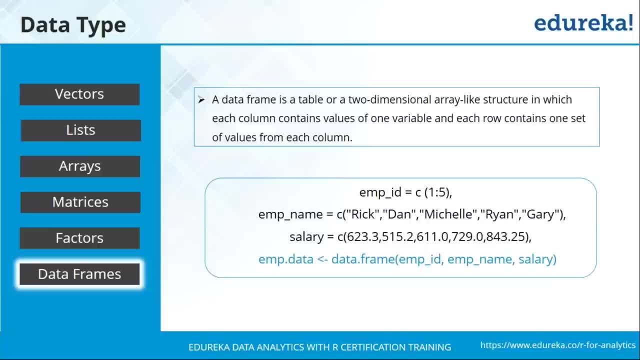 for now. don't worry too much about it. We'll be extensively talking about importing and working with different data sets in the next session, But I hope you guys are clear with respect to the different data types. Okay, so I've got a. 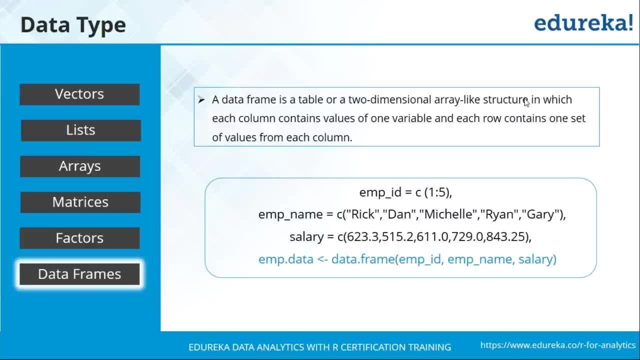 confirmation from Eric Shubham: Reshma Pankaj Gayathri. that's great to see, Adam. okay, that's nice to see that all of you are following. So with this we come to a conclusion. of data types. So I'm quite sure some of you are familiar with 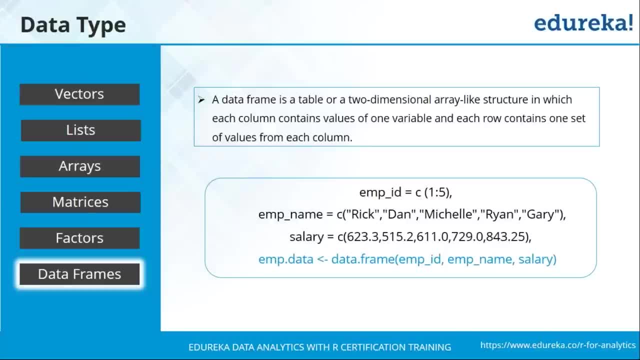 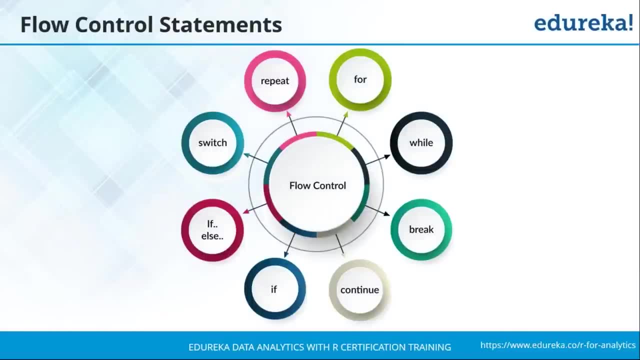 programming languages, and in programming language there's a very important concept known as flow control statements. Now, what these control statements actually do is they divert and control the flow of every program, as in the sequence of execution of these programs. So in today's session, we'll 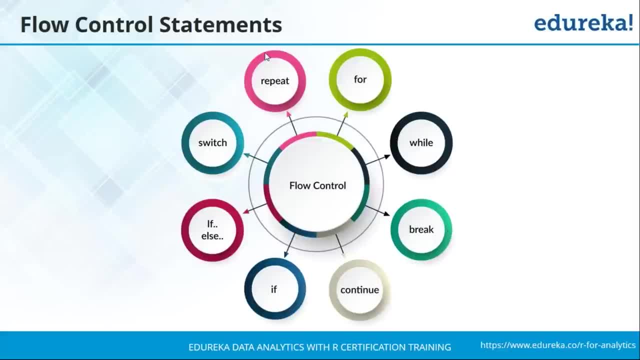 mainly be discussing across eight of these different flow control statements. You have, if you have, if else, switch. repeat for while break and continue: Now, if, if else, and switch. Now if, if else, and switch. 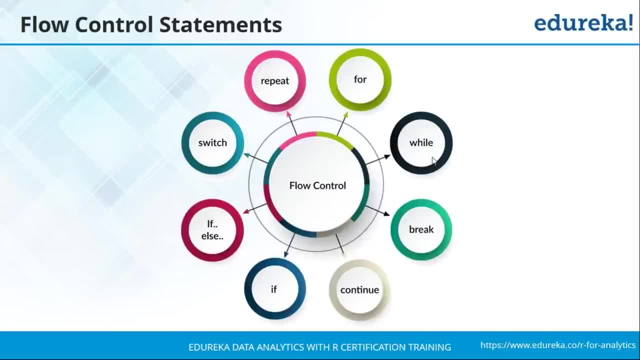 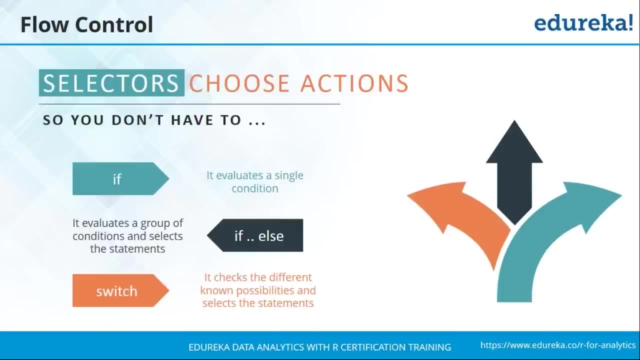 switch are your selector statements, whereas your repeat for while are your loop statements, Break and continue are jump statements, because they help you jump from the sequence of the operations. Okay, so we'll start off by talking about the selector statements. Now talking about selector statements. 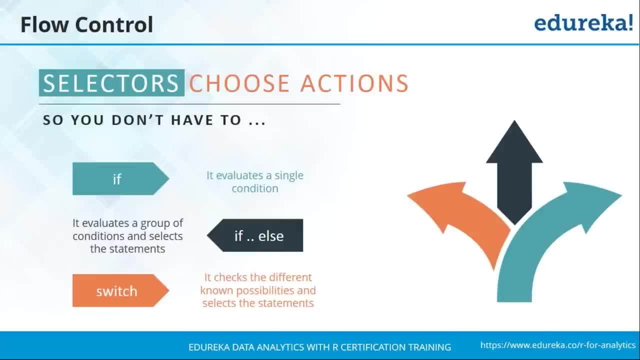 they have just a simple aim, that is, they choose certain set of operations after evaluating a condition, so that you don't have to bother to the exact detail. Now, there are mainly three selector statements You have: if, if-else and switch. 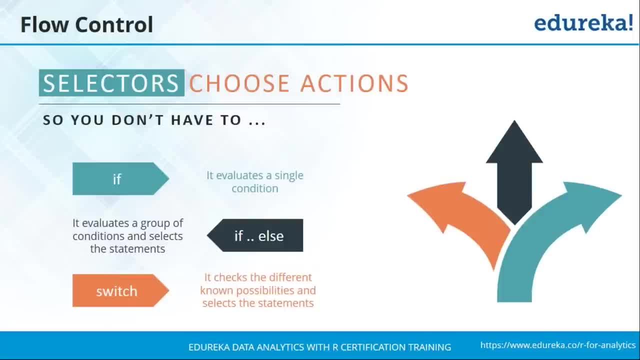 Okay, if actually evaluates just a single condition and decides what has to be done in case the condition is true. If it's false, it just ignores it. Now, if-else is a group of statements that can help you check multiple conditions. 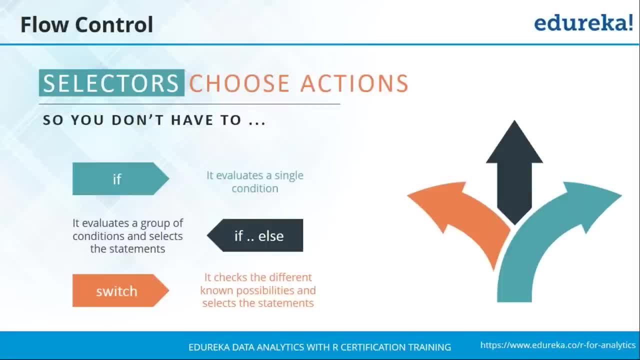 It's similar to the if, but it helps you achieve a bigger branch. Switch basically helps you check the different possibilities which are already known to you. That is, if a certain variable can take a specific value, then you can go with switch. 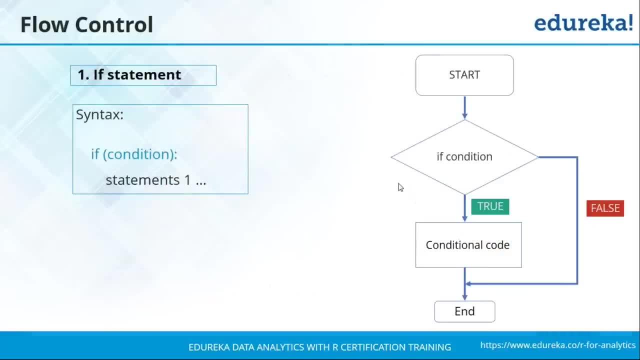 So the first topic that we'll be discussing is the if statement. Now, if statement is quite straightforward: It just has a single keyword, if, followed by the condition, and then a certain set of statement that needs to get executed in case it is true. 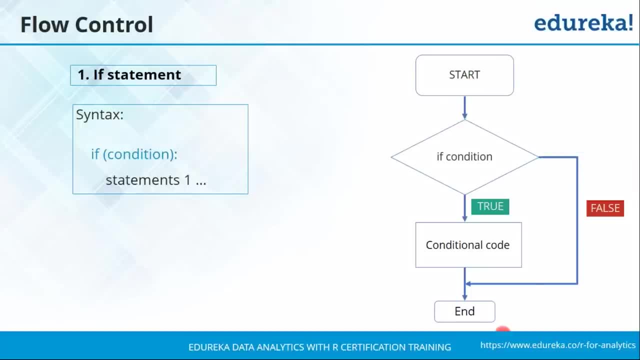 Now, if you look at the image to the right, this is basically the flow of if control. So you start off your code, you check the if condition. If it is true, the conditional code or the statement written inside the if will get executed. 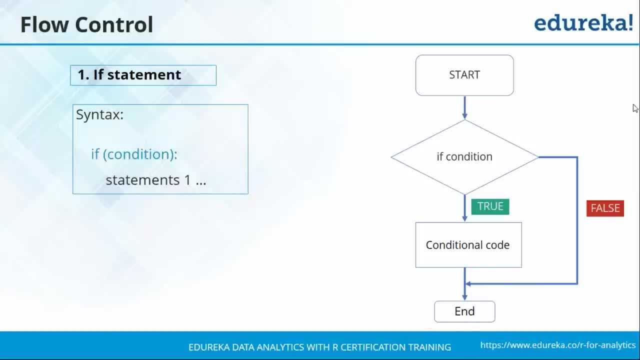 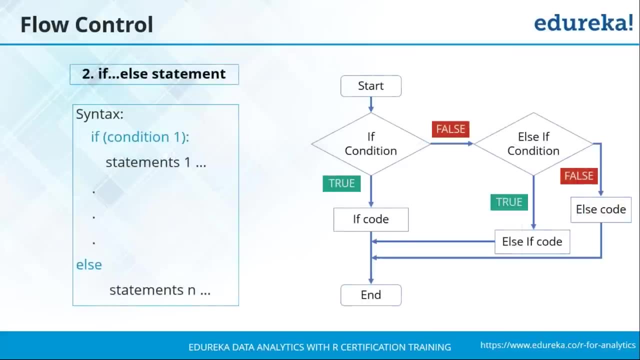 If it is false, the statement gets ignored and you will move forward. Now, before we go ahead and create an example of if, I'd like to discuss about if-else as well, because these two statements are completely related. Now you can use if and if-else or an else-if ladder. 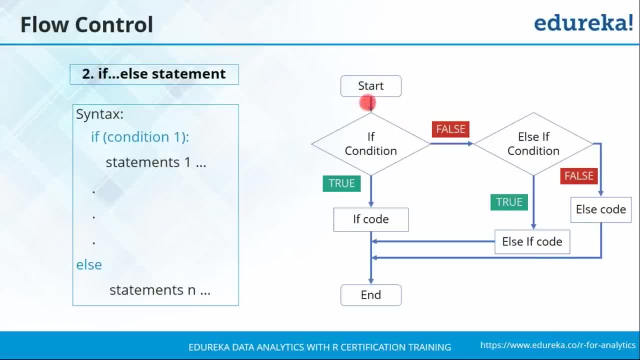 that'll help you achieve the following order. So what you do is you first check the code. If it is true, that means the first if code gets executed. If it is false, then it goes on to check the else-if condition and if it is found true, the else-if gets executed. 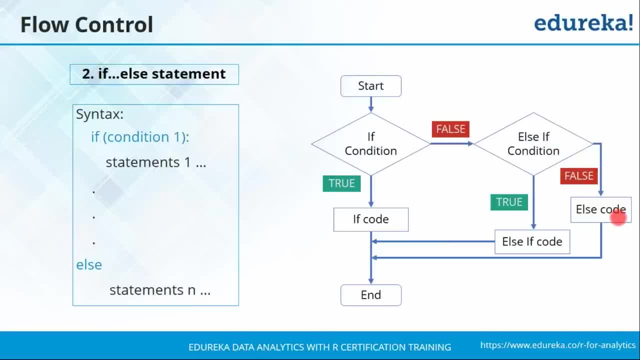 Finally, even if the else-if code is found to be false, then you go ahead finally to the else code and it gets executed. That is in case. if none of these conditions are true, then you execute the else statement, But you can have a multiple chain with respect to if-else. 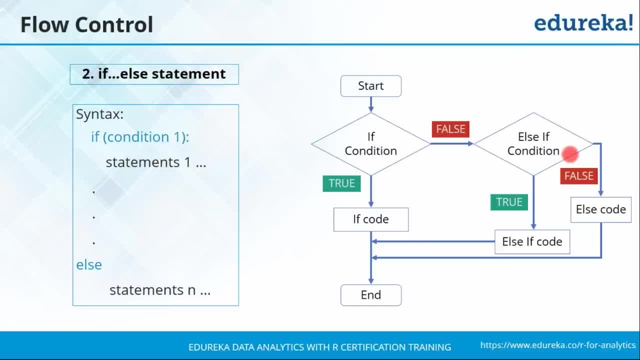 You can have any number of if-else conditions that you want, But it's suggested that you do not write too many, because it becomes confusion for the user as well. Now to see the practical example of the if-else statement, let's go back to our RStudio. 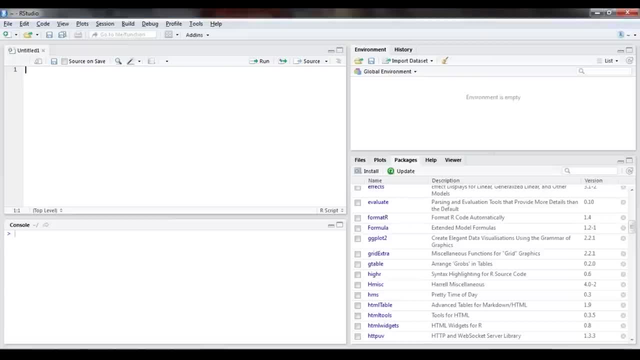 So let's begin by creating a new script file in which we'll write our code and directly execute it, rather than writing it on a console. So first let me begin by creating a new variable called x, and this is going to have a value of five. 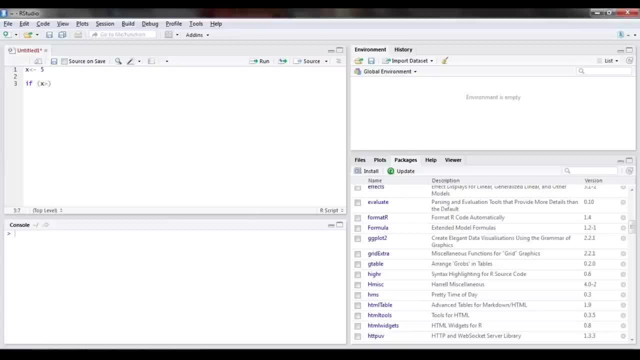 Now comes my if statement. if x greater than three, Then print x is greater than three. Now to run this, just click on the source option here and directly it will convert it and execute it on the code. So you can see x is greater than three. 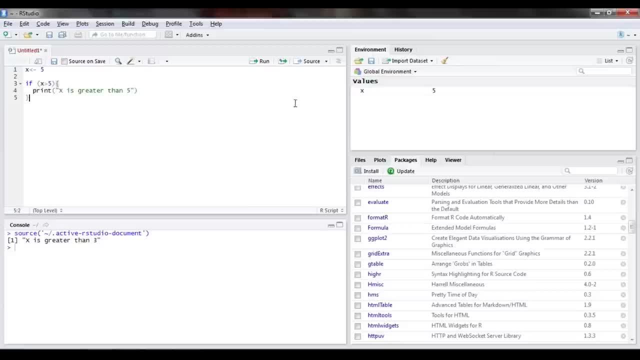 But let's say, I'm changing this value to five, Then I'm re-running this code, but there's no output here. Can you see that here? There's no output here because the statement written inside the if does not get executed. Now, in such cases, what you can do is 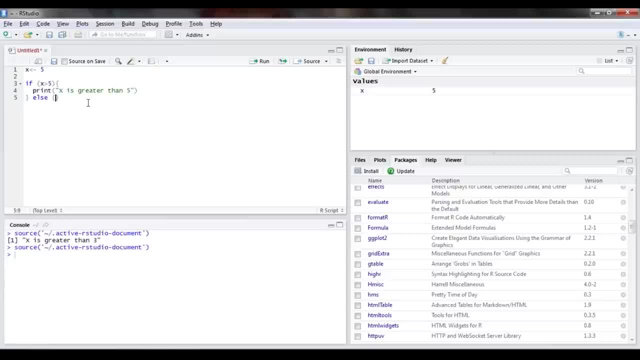 you can write an else condition where the if condition ends Else: print x is not greater than five. Okay, now you can run it and you can see printing x is not greater than five. But let's say you want to add another condition here. 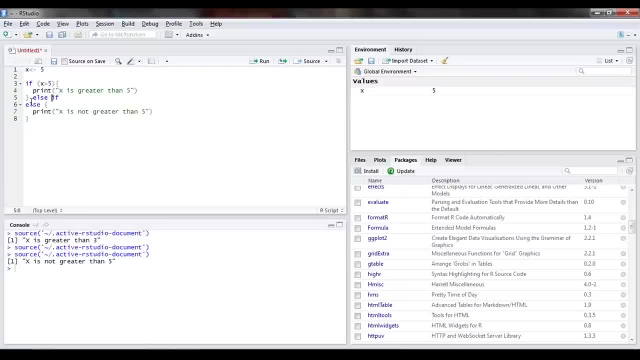 So you can write an else. if x is equal to five, Then print x is equal to five. Okay, let's run this and see: Sorry, double equals two. Always remember that for comparison. it's all double equal to. You can see it's: printing x is equal to five. 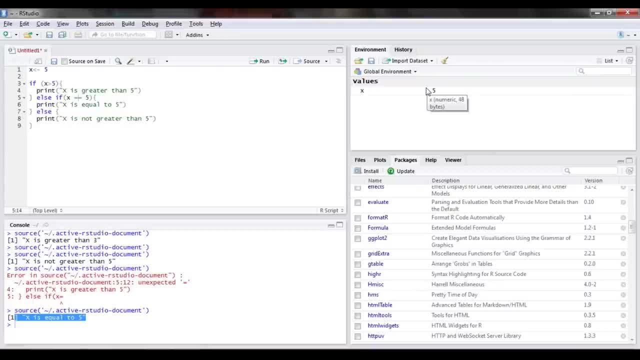 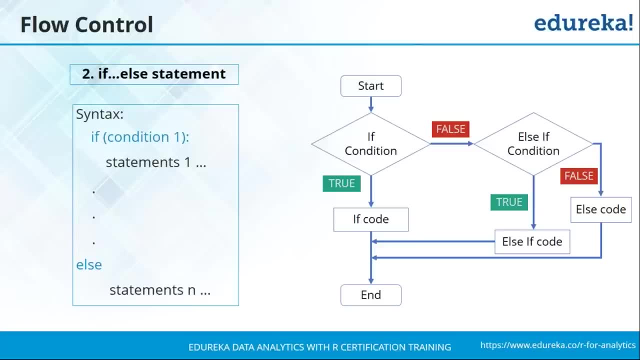 So the output's still here, How the if else ladder works. Okay, so I've got a confirmation from everyone. Guy three's asking me: is there a limitation on if else? No, Guy three, definitely You can use a continuous nest of if else. if, 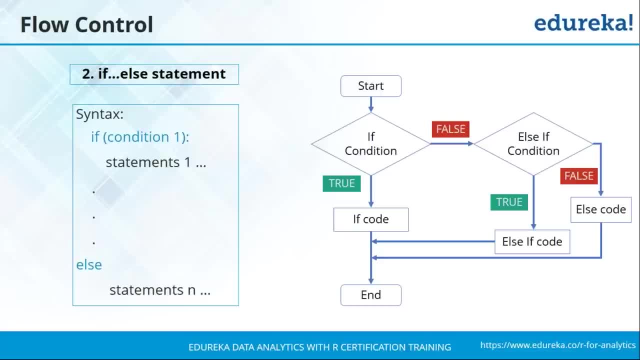 and else statement any number of times that you want. So it's all up to you. But again, the more you put conditions, the slower your code becomes, because it needs to check every condition with respect to that same. Okay, so make better decisions when you're doing that. 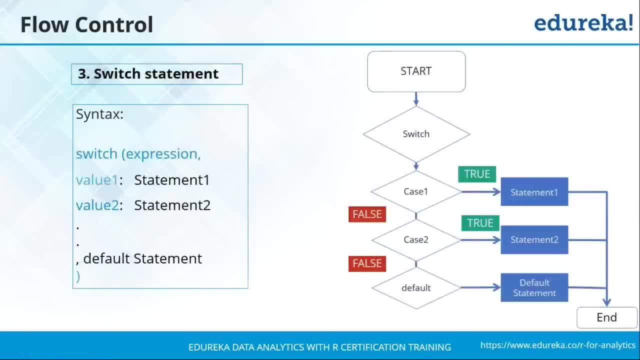 All right. Now the third kind of flow control statement is the switch case statement. So switch case is basically used to compare a certain expression to a known value, That is, you're already aware what value that variable can take and, based on that, what has to be done. 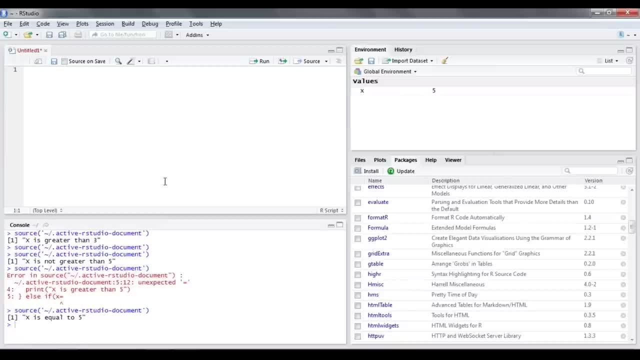 So let me go back to my R studio. I'll clear all this, For in case of switch, let's take a new vector here. Let's say VTR is my new vector And to this I'm gonna add certain values. 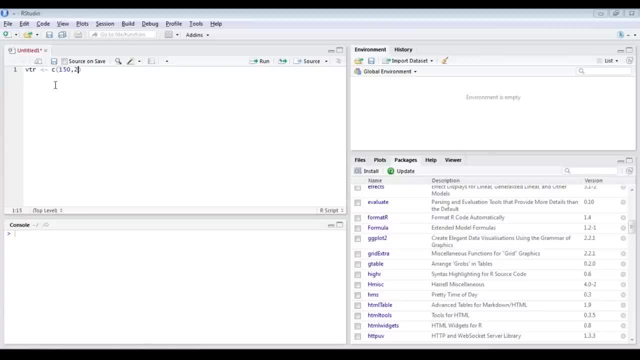 Let's say 150, 200,, 250,, 300,, 350, and finally 400.. Now what I need is I'm gonna write a new variable that says option. Now, option, basically, is gonna be the expression to be evaluated. 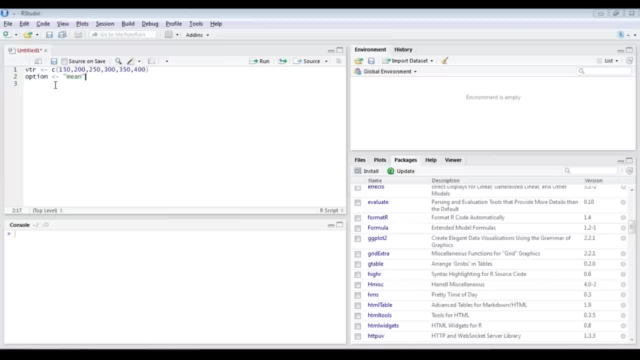 Now, in this case I'm just assuming it to be equivalent to mean and then I need to identify mean of this operation. But in general cases it can take any values and that's exactly why we take switch case. So here, if I write switch, 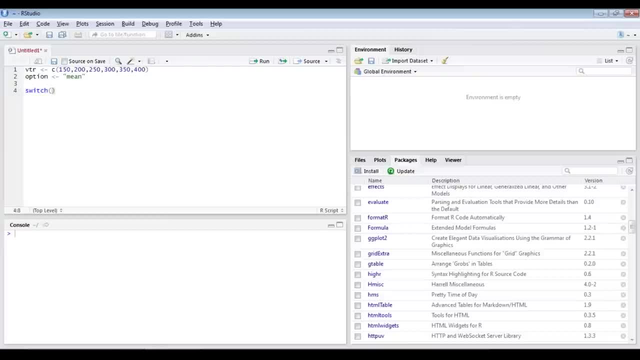 I need to specify first the expression. So my expression is with respect to option. After that put a comma, Then it can take. it can be mean which is equal to now to compute mean you already have an inbuilt function. 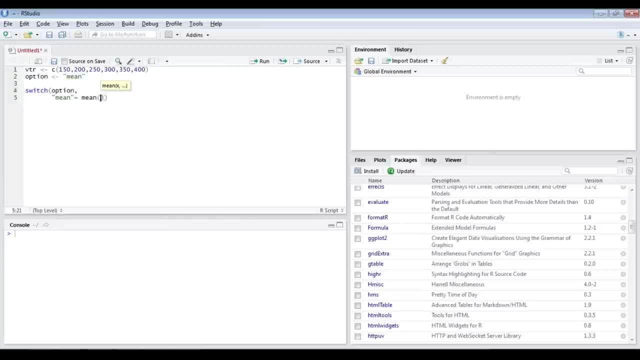 so which? you just need to pass the parameter. So in this case, it's my vector. Now to move to the next case, just put a comma, Let's say mode. Again, mode has an inbuilt function. And finally, let's say median. 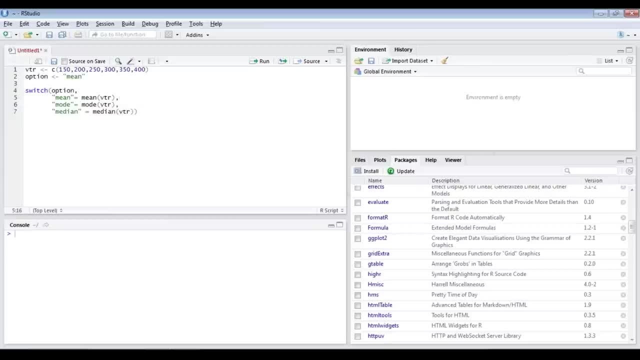 Now all these results have to be printed, so add a print before it And then you can directly close the switch case statement. So with this we've completed the switch case and let me just print run this code: 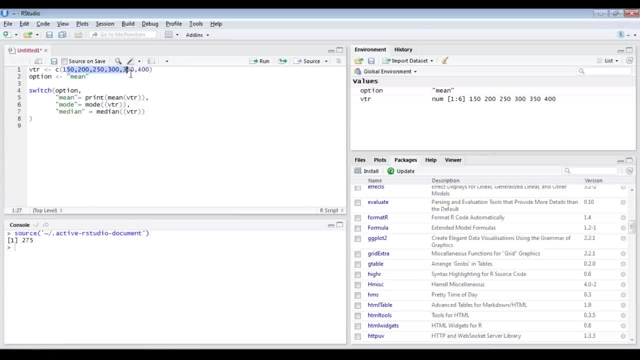 And you can see here, 275 is the mean of this vector, which has different values ranging from 150 to 400.. So from this range value, the mean is found out to be 275.. And if I say median, 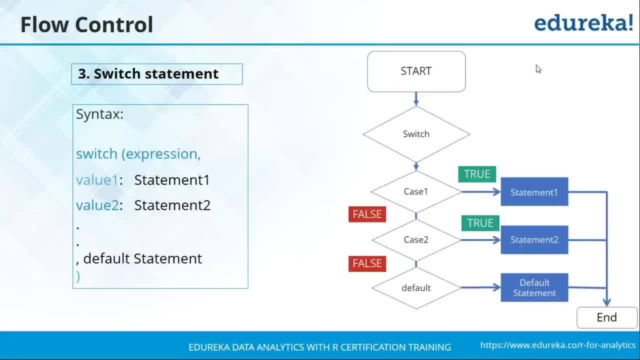 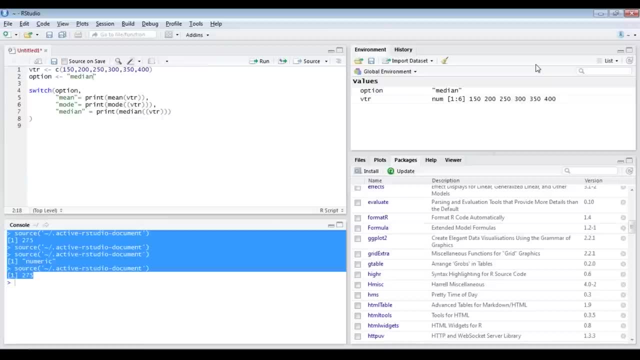 then the median is also calculated. So I hope you guys are clear with respect to switch case statement and how they work. Any doubts? Okay, how do you write default statement? Okay, default statement's quite interesting here. Just put a comma and then you can write. 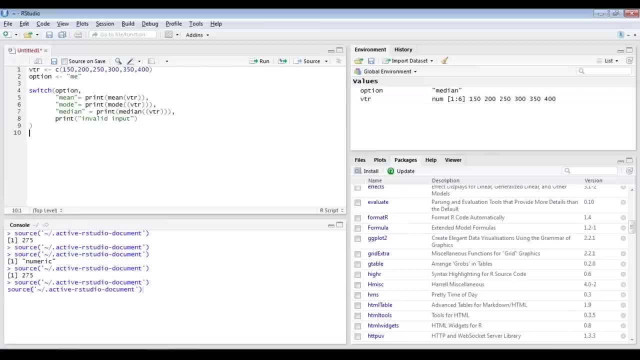 and just change it to ME, and then, if you try to run this, the default case is considered. So, as long as you don't specify the case, and the last option is considered to be a default state. Is this clear, Varun? 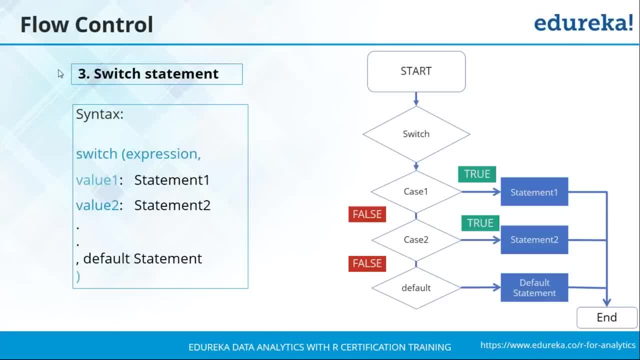 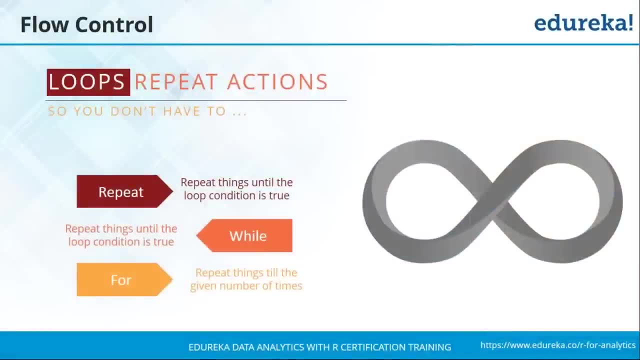 Okay, that's good. So with this we actually come to a conclusion of our flow control statements. The next kind of statements that we're gonna be talking are loops. Now, what do loops do? Loops basically help you repeat a certain set of actions. 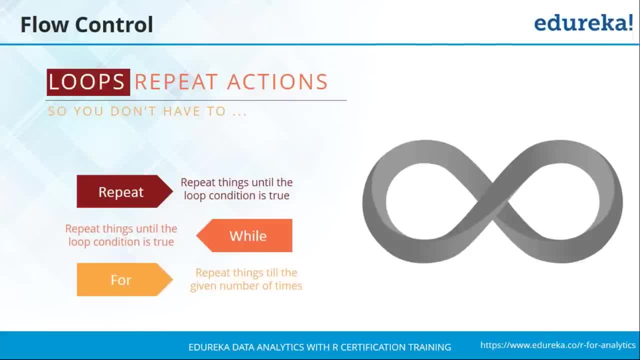 so that you don't have to perform them repeatedly. Now, the main objective of a loop is quite simple. It basically helps you repeat a certain set of actions n number of times so that you don't have to manually write. Now imagine I need to perform an operation 10 times. 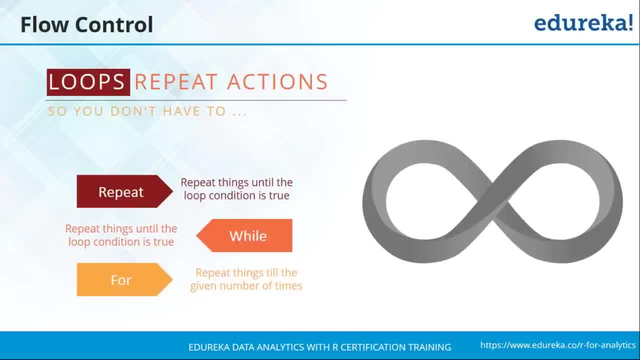 So if I start writing the code for it 10 times, then what happens is the code length increases and it becomes a problem also for the user to understand. At the same time, by using a loop, if I write the statement I wanna execute 10 times, 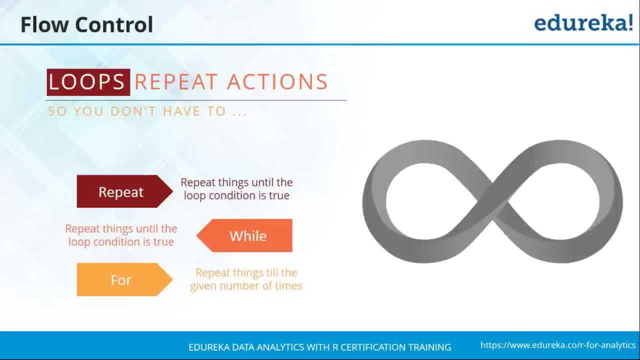 inside a loop, then it saves me the code length as well as it makes easier for code readability. It also optimizes with respect to code efficiency. Now repeat statement and while. statement helps you execute a certain set of codes until the condition is true. 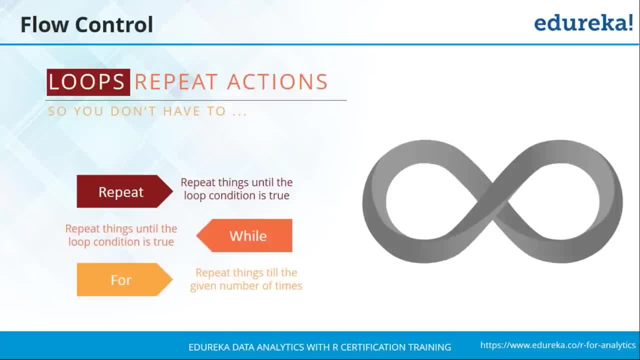 But for is a kind of loop statement that you use when you know how many times you need to repeat that statement. Now let's say you wanna repeat a set of statements 10 times, Then you'll go with the for loop. 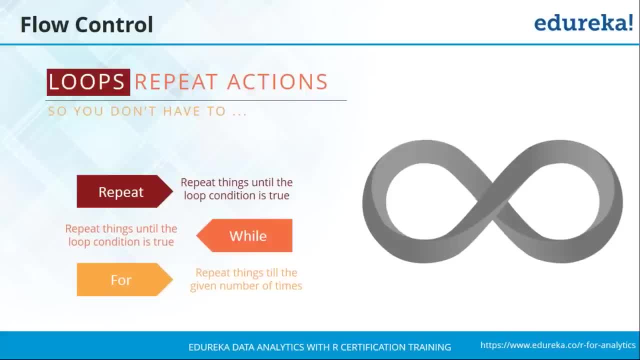 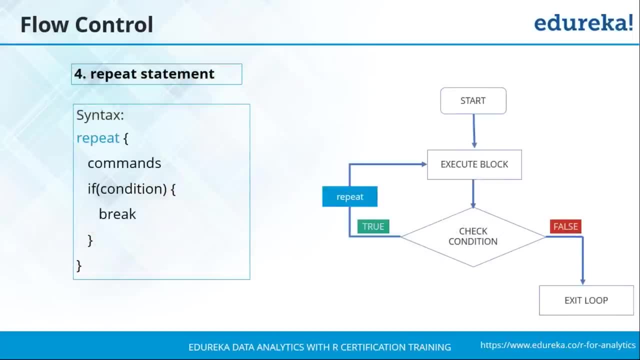 But let's say you're not quite sure on how many times you wanna repeat it, then you go with the repeat or while loop. So let's move forward and start talking with respect to the repeat statement. Now this is the basic syntax of the repeat loop. 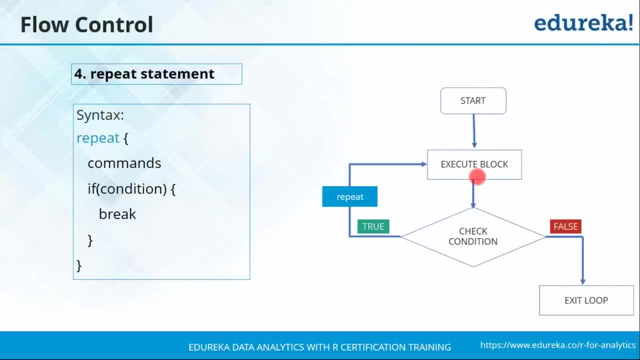 So first you start and then you execute your code. Once you've executed it, you check if the condition is true and if it's true, you go back and execute the block until the condition is meant to be false. Once it's found out to be false, 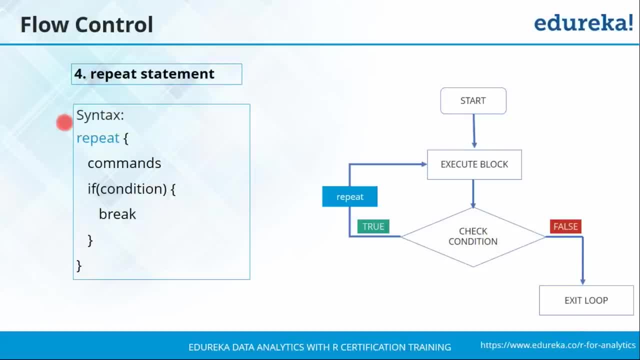 then you break from the loop and you exit. So this is the general syntax. You have your repeat keyword, then you have the commands that need to be executed. Once the command has been executed, you need to write a condition based on which the loop statement will exit or not. 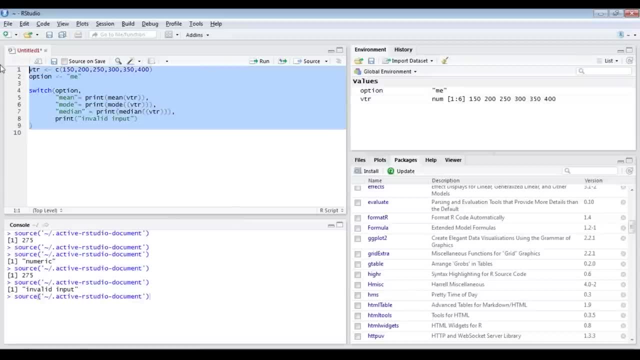 So let me show you how it's done. So let me just clear all this. So let's say: repeat Now here. let's say: before this, I'll just declare a variable. say x is equal to one. 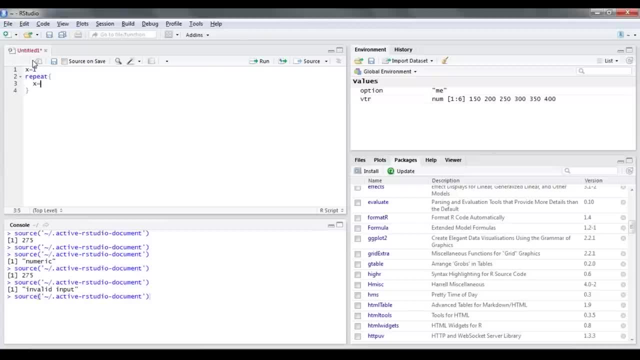 and I'll say: x is equal to x squared. Now I'm gonna write if I'll change the value of x to two. If x is greater than 100, then break Okay. before this, I'll just print x. 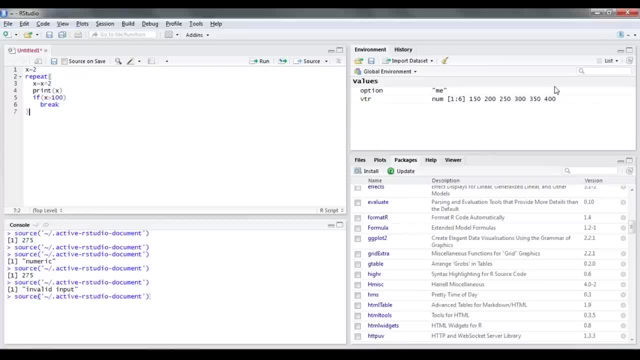 so that you can follow it. and then it's time we execute this code. So you just run this and you can see the value of x first reaches four, then it becomes 16, and then once it becomes 256,. 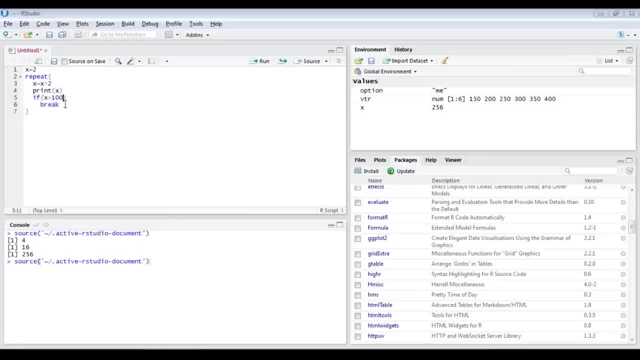 we realize it's greater than 100, so we break from that loop Again. if I add another zero and rerun this, then you can see from 256, it's again getting squared and it's getting and the number is becoming 65536,. 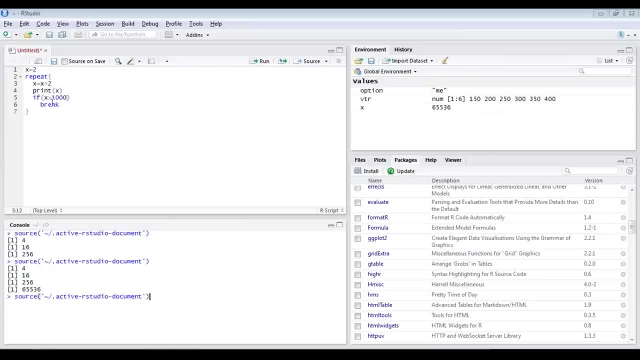 which is greater than 1,000, and you're breaking from that loop. So, basically, in situations where you're not quite out, you're breaking from that loop. So, basically, in situations where you're not quite out, you're unaware of how the value is changing. 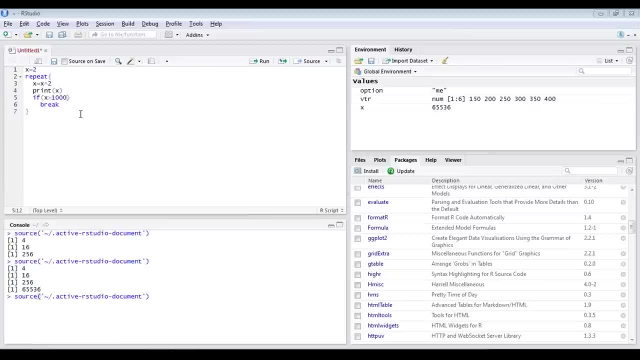 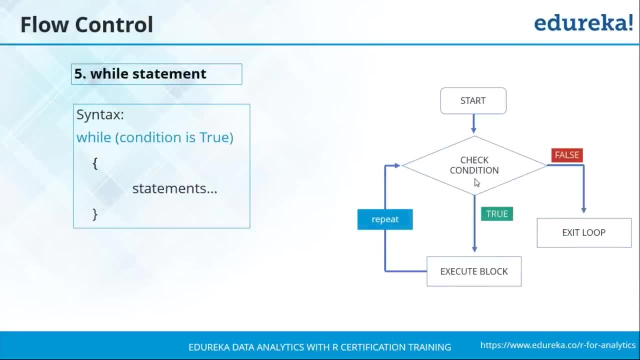 but you know at one point where it has to stop. then you use a repeat loop. Similarly, a while loop is also quite the same. If you go back to your presentation, while loop actually starts by checking the condition and then it executes the code block. 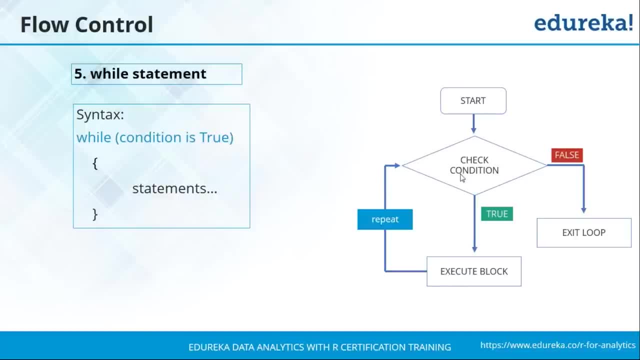 Okay, and once you've completed execution of the code block, then it goes back and checks the condition. As long as your condition is found to be true, it'll keep executing the code block, but the moment the value is found to be false. 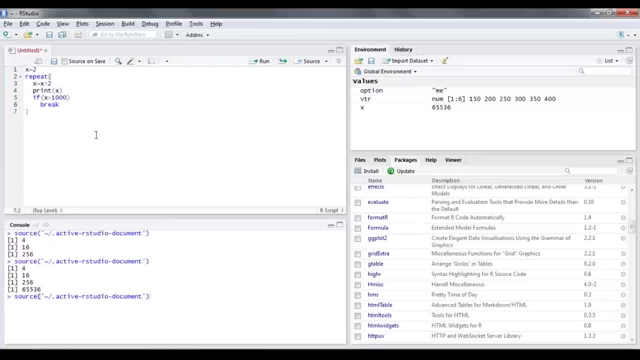 then you exit from that loop. So let's go back here and I'll modify the same code for while loop. So here what I'll do is I'll change it to while, I'll bring in this condition and I'll remove the condition from here. 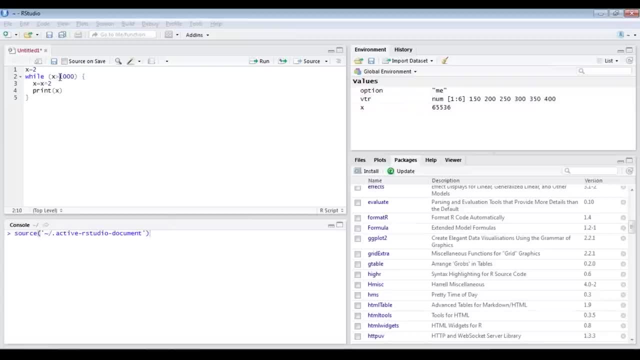 So how your repeat and while loop changes is earlier. with respect to your repeat, you had actually changed this condition to be greater than 1,000.. But in case of while loop, you're basically gonna change it to less than 1,000.. 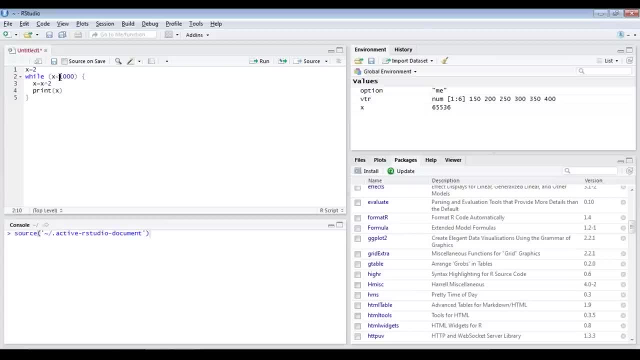 That is, if the value of x is less than 1,000, then only enter that loop. Now, if you re-run this code, then you can see the output present here, which is same as our repeat loop, but the major difference here. 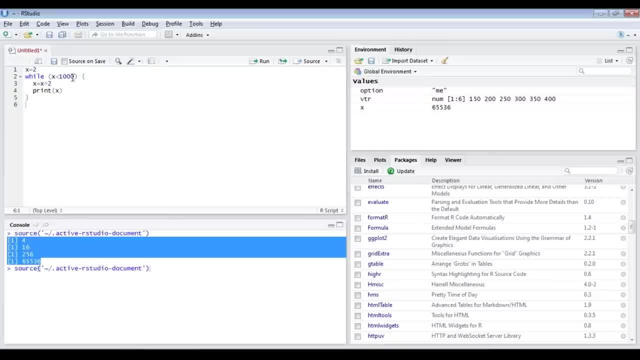 is change with respect to the condition. Now your while loop basically defined when you're going to enter the loop, whereas your repeat loop defined when you're gonna exit from that loop. So these two statements are better known as entry control loop and exit control loop. 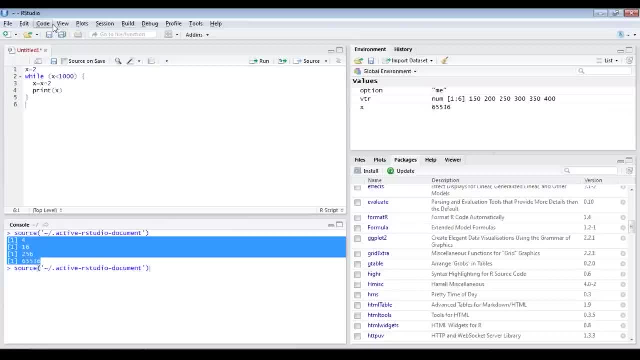 Your repeat loop basically defines your repeat loop. loop is something that defines when you leave from that loop after you've completed execution of the statement, But as your while basically controls when you're going to enter into that loop to execute the statements. Okay, that's how. 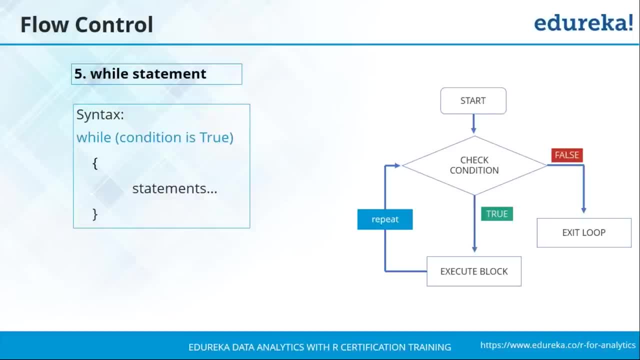 your repeat and while loop are different, So I hope you guys are clear with respect to both these loops. Okay, Reshma says yes. so does Gayathri Adam, That's great to see. Okay, so the last kind of loop that we'll be discussing is a for. 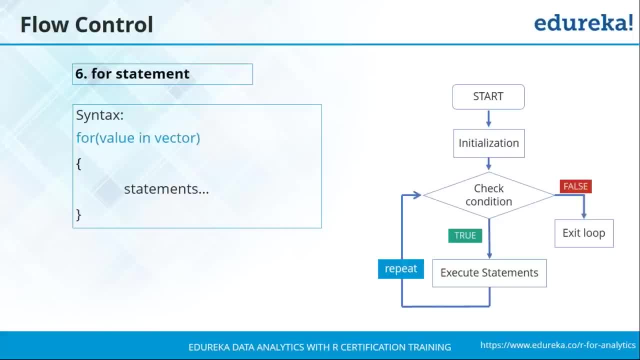 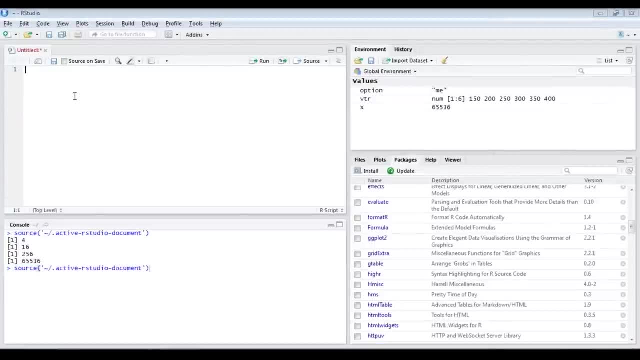 statement. Now your for loop is quite straightforward. Okay, when you know how many times a loop has to be executed, then you can directly go ahead and execute. So let's say I'm going to define a new vector, VTR. Now in my vector, what? 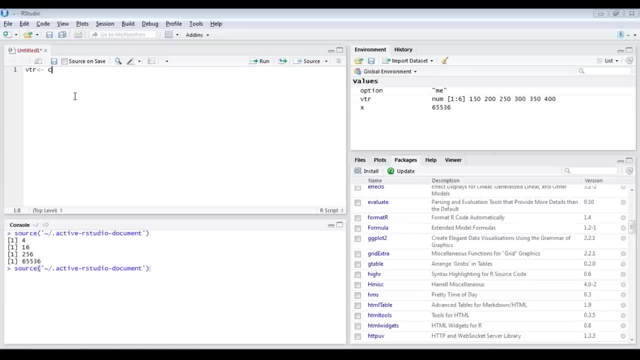 I'm going to do is I'm going to add five elements: 7, 19,, 25, 65, 45. Okay, now I want to print them one by one instead of individually printing all of them at one go. 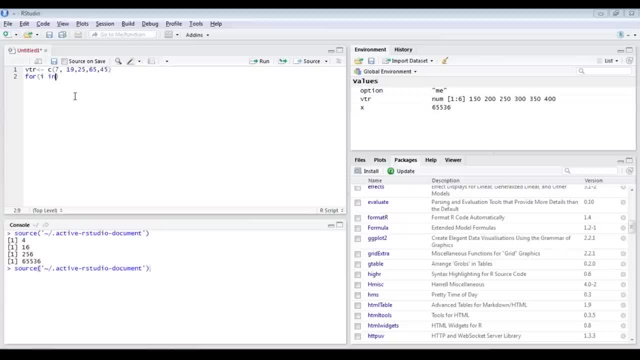 So in that case what I'll do is I'll use a for i in my vector VTR. Okay, so for every value in my vector VTR, I'm going to print that value. So basically, you just need to write print of i. Okay, so if you run this, you can see all the 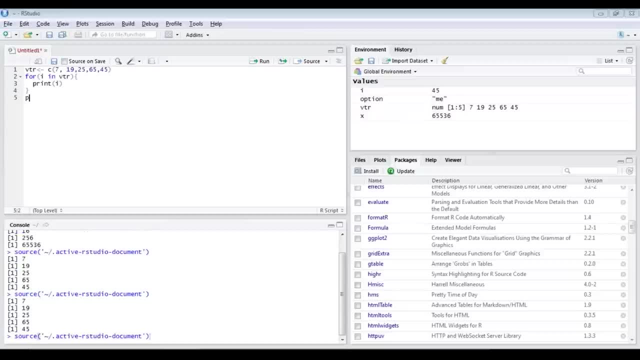 values are individually being printed here. Okay, but if you just directly print VTR, you can see the difference between both. So where one is printing each value in new line, when you print the whole vector, all the numerical values are present in the same line and are considered to be one entity as part of. 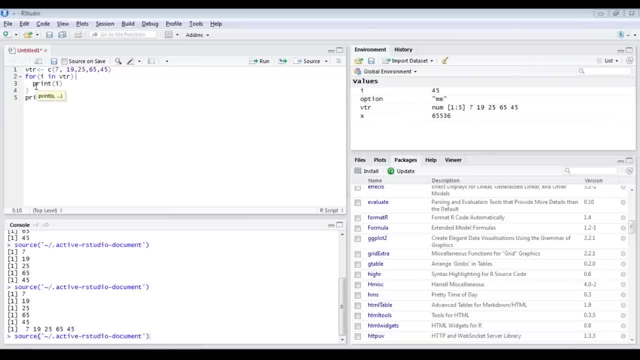 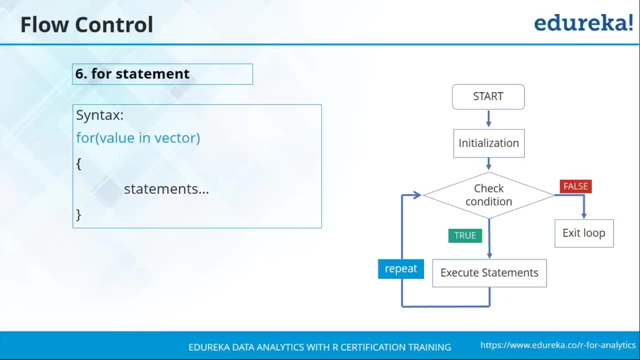 the whole vectors, But here you can access each of the values one by one. So I hope you guys are clear with respect to how to work with the for loop. Okay, so your for loop is something that you'll definitely be using while you're working. 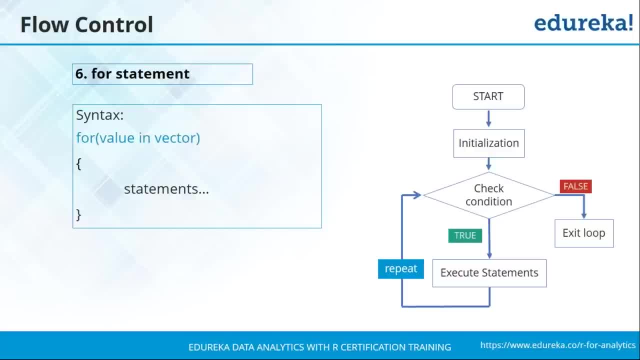 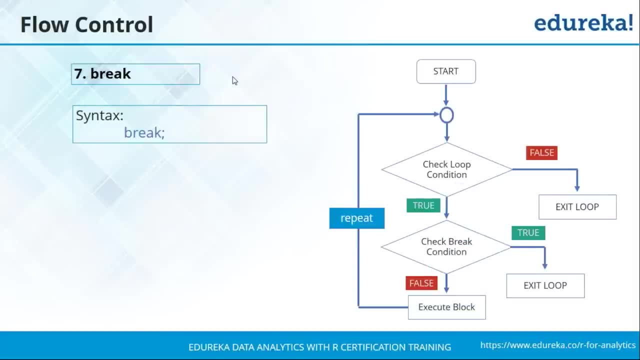 with matrices, as well as arrays and some amount of data frames as well. Okay, so keep this in mind, because this is an important concept. Now comes your break Again. so you've seen break, how break statement works, while we had seen our repeat loop, but none of you actually put across the question: what a break? 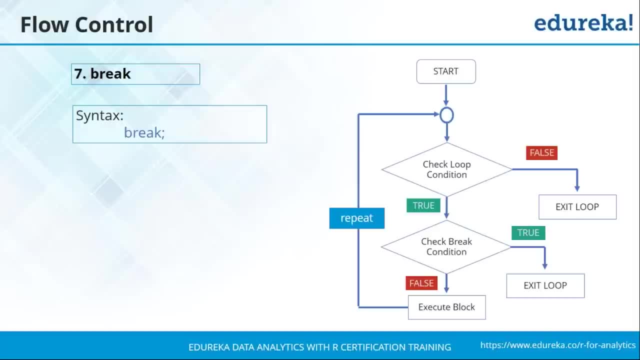 statement was. So. a break statement basically helps you come out from the loop whenever it is being caught. Now, if you look at the image here, first, what you do is you check the loop condition. If the loop condition is found to be false, then you exit from that loop. After that you come in and you check if the 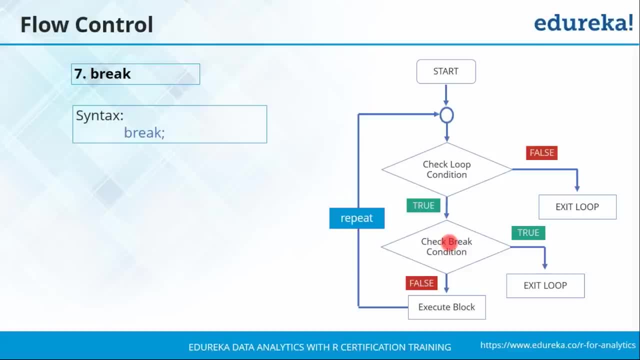 break condition is true. That is inside a condition. when you have written break that condition, is it true or not? If it is true, then it will encounter a break and it will exit from that loop. but if it is not true, then what happens is the code written after break gets executed. 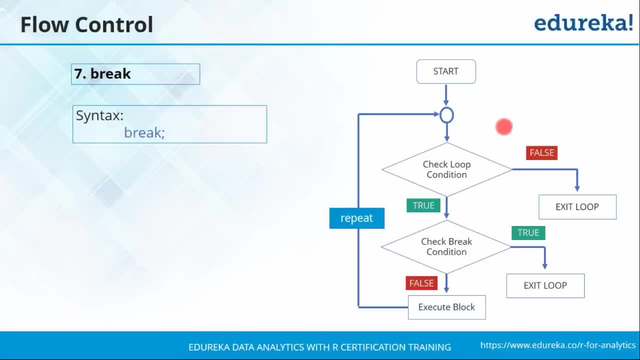 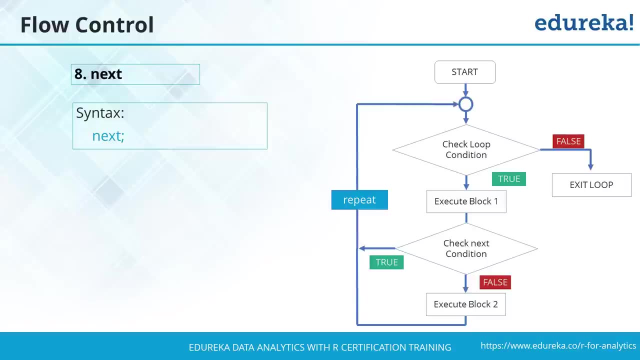 and then you go back and repeat the whole loop once again. So after your break comes the next statement. Your next statement is quite similar to the continue statement that you have seen in other programming languages. Now what actually happens is your next is slightly opposite to your break statement Here. 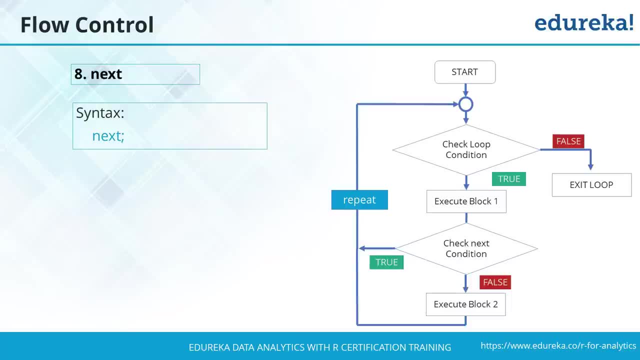 instead of leaving from that loop. what happens is if you encounter the next statement, Every code that is written after that does not get executed and you go to the next iteration. Ok, so if you look at the flow diagram here, you check first the loop condition. 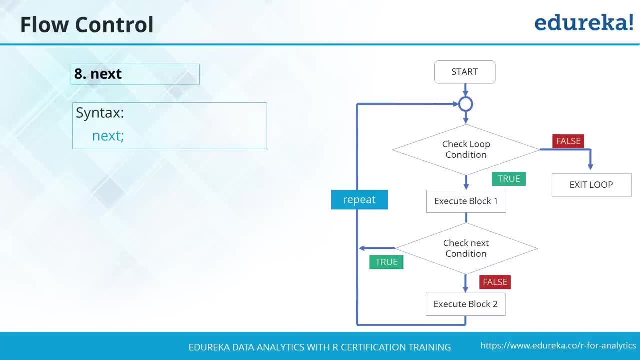 and then let's say you have certain codes written before the next condition, Then you check if the next condition is found to be true or false. If it is false, then you'll execute the remaining code written in that block and then you'll go to the next iteration. But let's say the condition is found to be true, then you 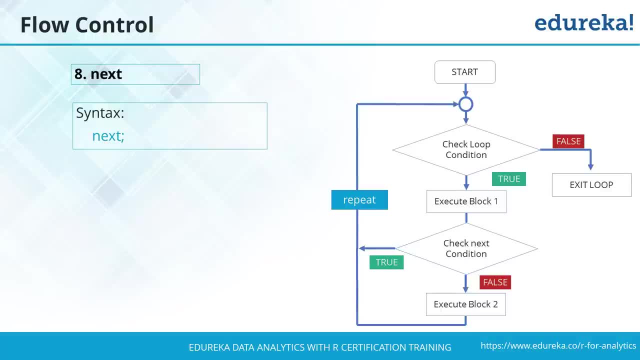 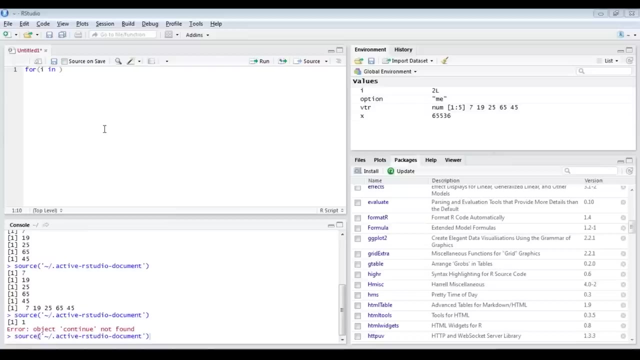 do not execute the code written below it, and then you iterate to the next loop. Ok, now let's go back to our RStudio and show you how it works. So here, what I'll be doing is I'll say, for i in, let's say, I'm going to give a 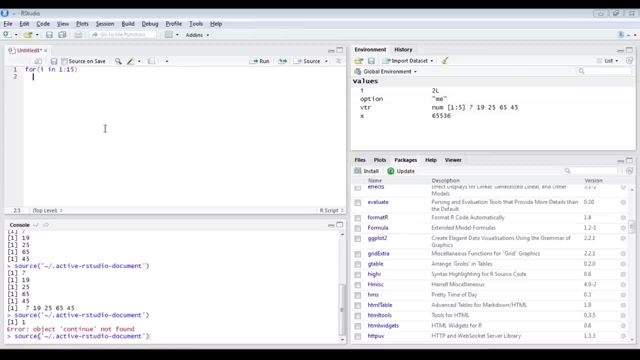 specific range, so 1 to 15.. Now, in this range I don't want to print even numbers, so for that, if i modulo 2, that is when I divide i by 2, the remainder is equal to 0. then go to next. Go to next. If not print i, Ok, so let's try executing this code. 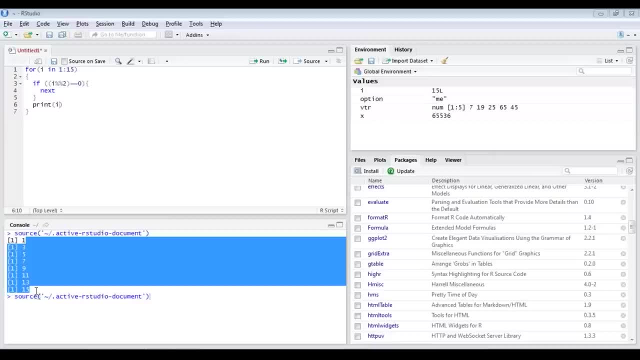 So just run this and you can see only odd numbers are being printed and even numbers are not getting printed. So basically, every time the statement is found to be true, the next keyword is being encountered and then the print command is not executed, So it goes to the next iteration without checking the 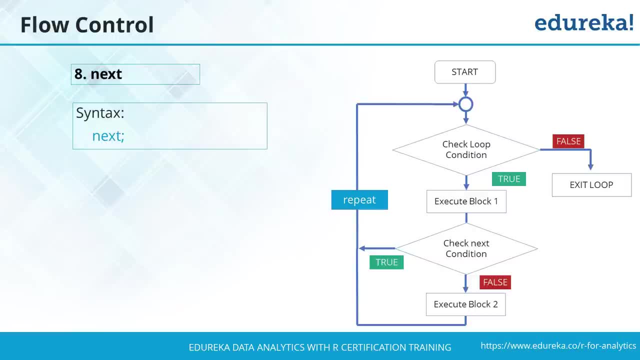 code written after this. So I hope you guys are clear with respect to these flow control statements. Ok, that's great to see. I've got a confirmation from Reshma Gayathri Roshni Adam Shubham Pankaj. That's great. Until now you've seen the analytical aspect of R. 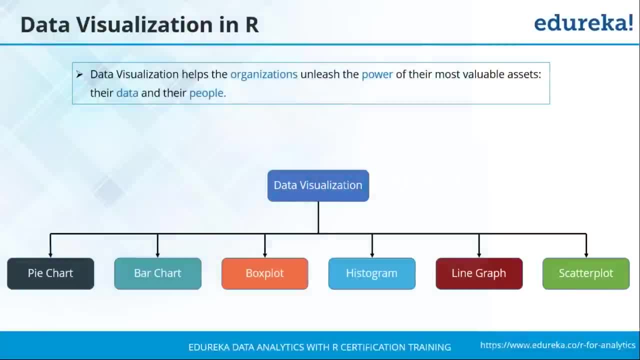 So now let's move forward and look at the visualisation aspect of R. So, with respect to visualisation aspect in R, you can create the six different kinds of plot using a data that you have. Now I'll be showing you an example of. 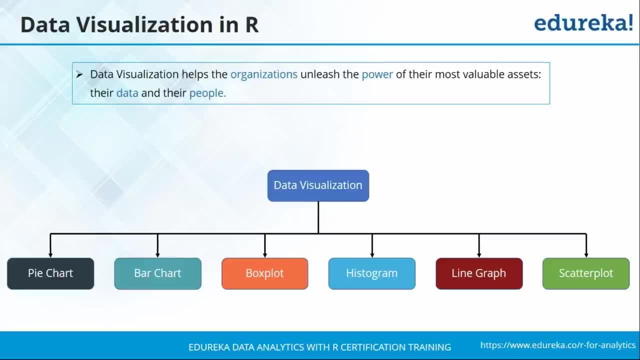 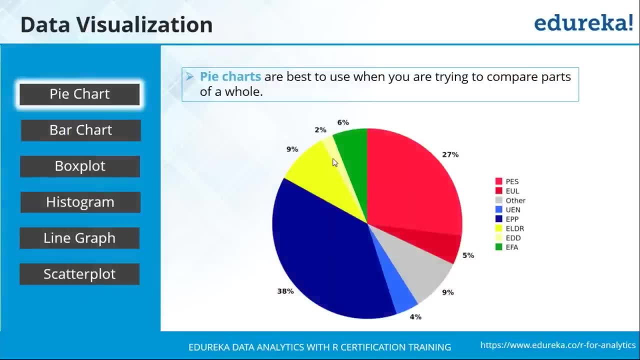 how to create each one of these plots at one by one. So we begin by first talking about pie charts. Now again, when you talk about pie charts, pie charts are best used to compare different parts of a whole. So again, let's say: you have. 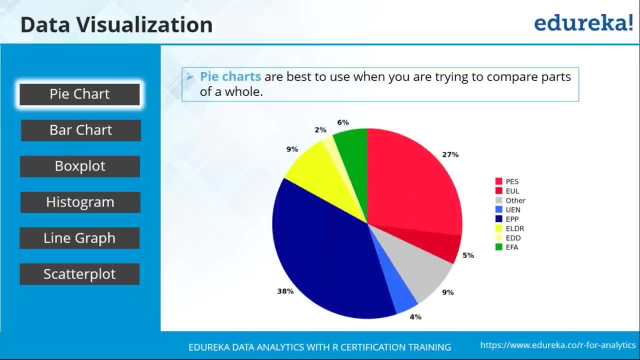 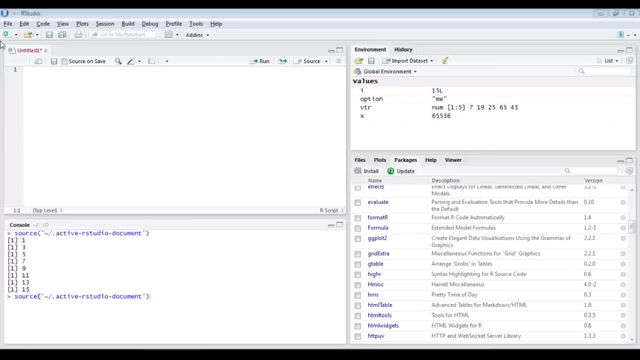 different branches to identify which branch is getting you more sale. it would make more sense to plot a pie chart with respect to all the branches of details. Okay, so create a pie chart. it's quite easy. let's go back to an R studio and I'll show you how to do that, So I'll just clear all this. Now I clear the. 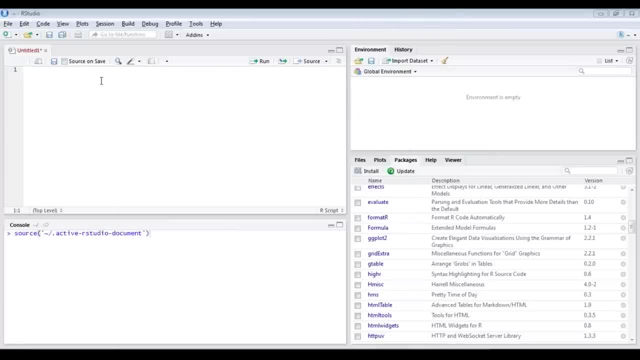 memory here as well. I have a vector, VTR, in which I'm going to have percentage of my five departments. Okay, so see, let's say one department is contributing to 14 percentage of my sales, the other is contributing with respect to 28. 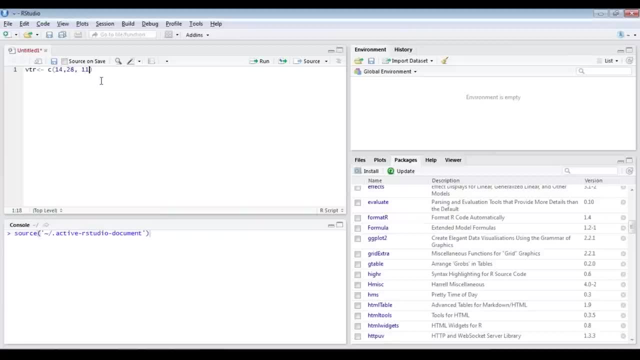 percentage. then there's a department that contributes 11 percentage, and then there's one which contributes to 30 percentage of mine, and finally I have another one which contributes 17 percentage. Okay, so these are the different percentage with respect to each department, But to understand better which department is contributing, 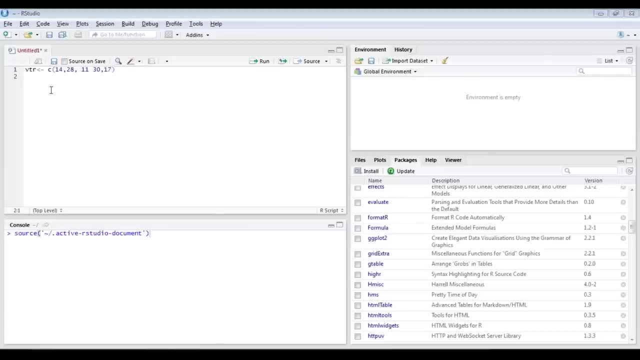 to each value. I'm going to create a new vector as well. that's called names. So here I'll just give some of the departments. I'll say R&D, then let's say I have marketing, I have corporate, then there's sales and finally I have support. 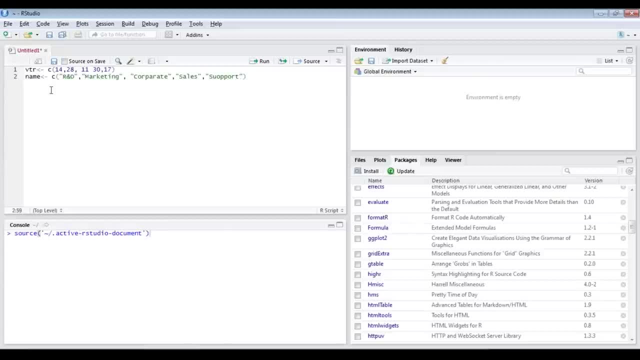 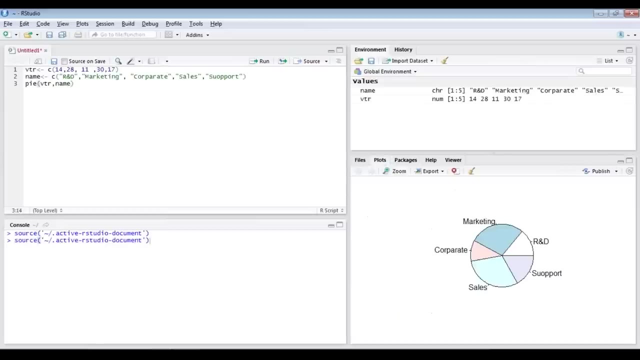 Okay, now, with these two values, I'll just show you how to plot a very simple pie chart. now, if I just say pi of vtr comma name. so you just need to run this code and you can see the plot has been provided to your left. so here you can see the contribution of the different. 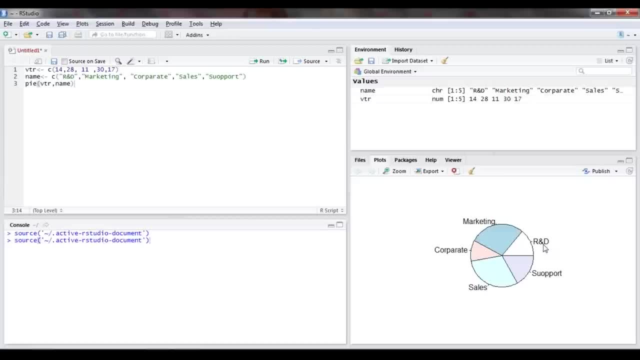 departments. you have marketing, you have corporate sales support and R&D, and a pie chart has been created from the corresponding values that you have taken from vector. so this color seems a bit dull for me. so I'm going to say: col equal to rainbow, so rainbow. 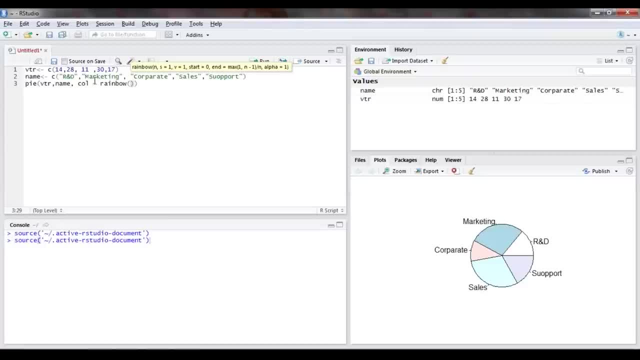 basically gives me different values. now how many different values do I need? I need length of vector. that means with respect to the total number of values present in vector. please give me different colors. now if I run the same code again so you can see the change with respect to the colors. so this looks: 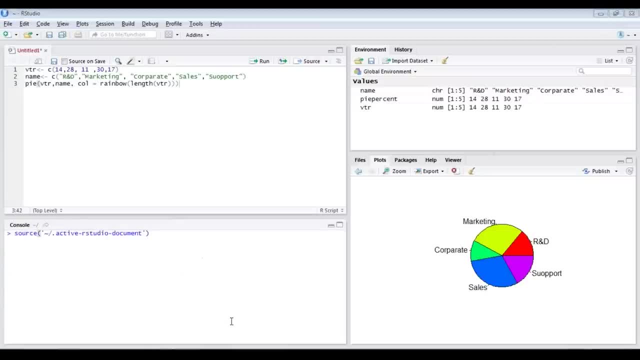 a little more better. so this is not the end of capabilities with respect to pie chart. there is a lot more that you can play around, but this is just to give you a simple idea that you can plot a pie chart like this. it's basically with respect to three simple steps that you're writing in R. okay now. 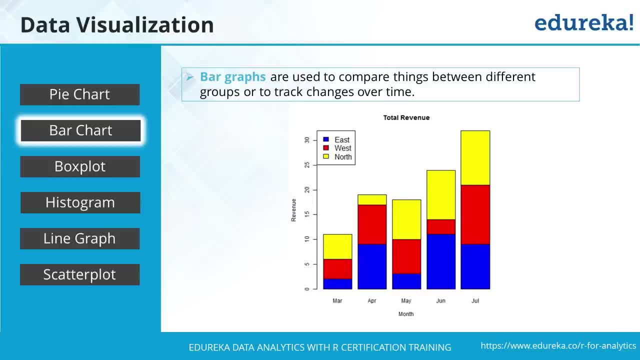 apart from this, the next type of graph that we'll be looking at is bar chart. now, your bar chart are basically used to compare things between two different groups or track the progress of certain things with respect to different times as well, so let me show you how to. 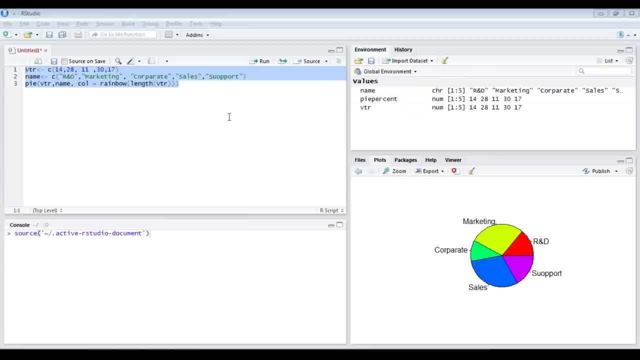 simply, it is to plot a bar chart as well. now for a bar plot, I'll just modify the same content, I'll just remove this line and say bar plot, and I'll just pass VTR. so this is all the value that I need for plotting a simple bar chart. and if you 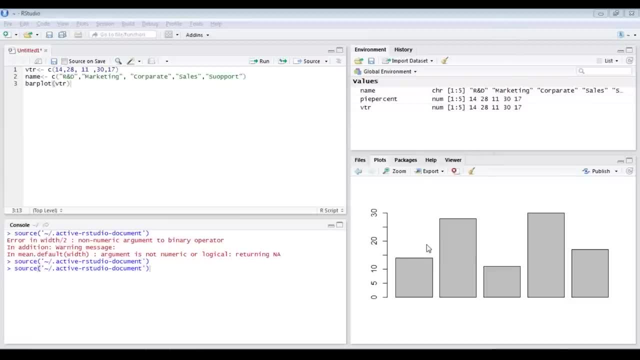 run this, you can see a bar chart with respect to the different values present here, so you can always zoom and see a complete bar chart. apart from that, let's say, if you want to even export this image, then you have the option to save that to R. okay. 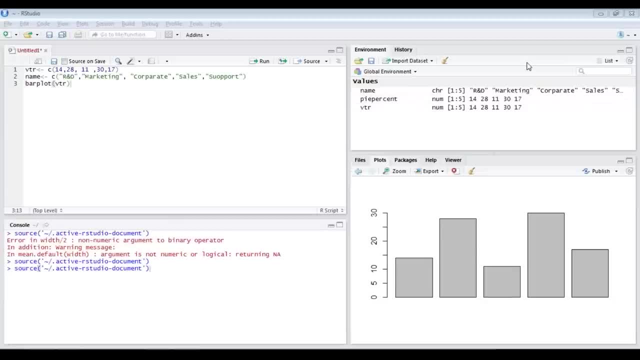 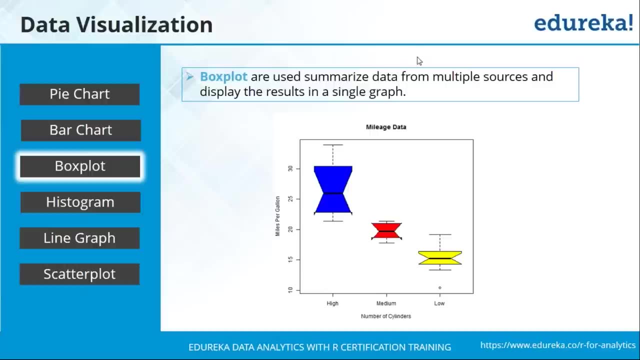 so this is how you plot a simple bar chart. now, apart from bar chart, you can also plot a box plot. again, when you talk about box plot, this is mainly used to summarize the data from multiple sources and display the result basically in a single graph. so, again, when you summarize the data from different graphs, it 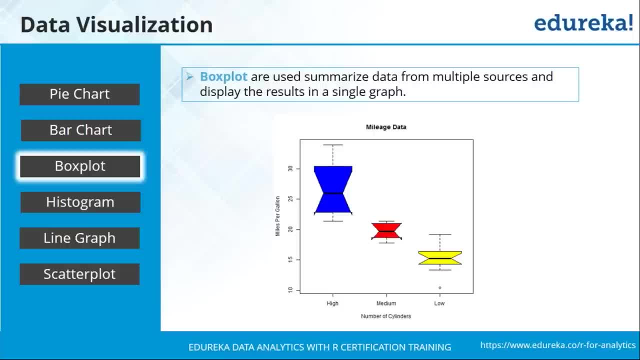 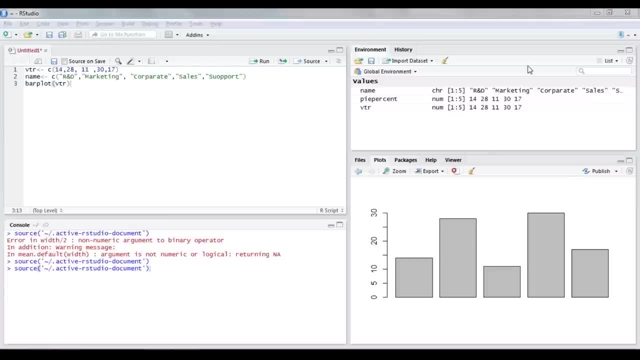 becomes a problem for you to use any other representation to understand better the difference or the change as well. so your box plot definitely helps you achieve that. so let's modify the same code to create a box plot. okay, so for bar plot, what we'll do is we'll be using a standard input data set that. 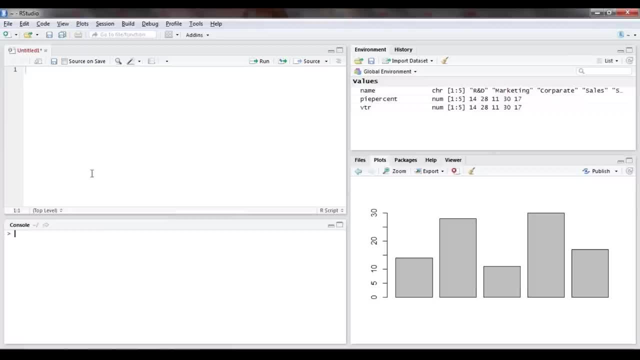 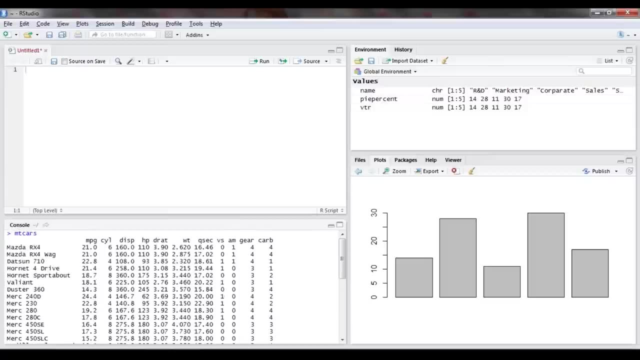 is present in our library, that is, empty cars. so to see the data set, let's say, empty cars is there. so if you just print this, you can see the complete list of empty cars. now here, what I'm going to just take is: I'm just going to take the 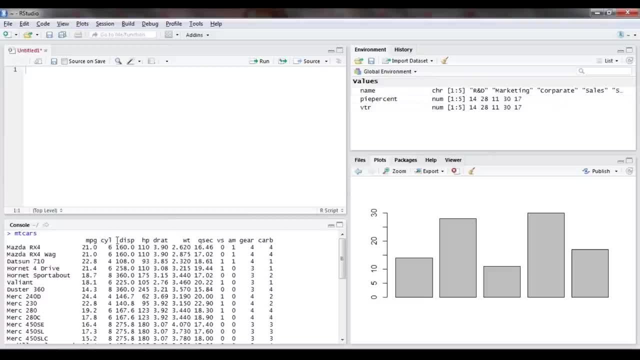 name. I'm just going to say the maximum power with respect to the cylinder, and then I'm going to create a bar plot with respect to that same. now, this is a simple command that I have written here that will help you achieve the same. okay, so these two columns have to be selected. the data is from empty cars in. 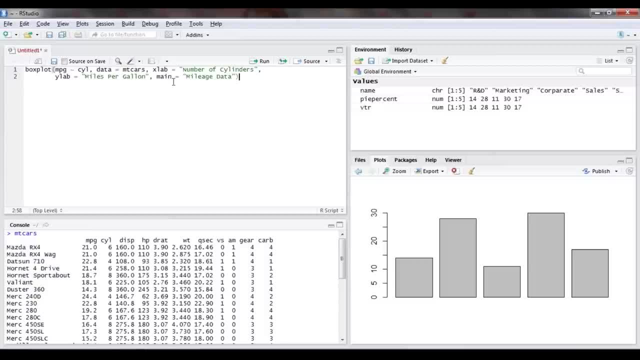 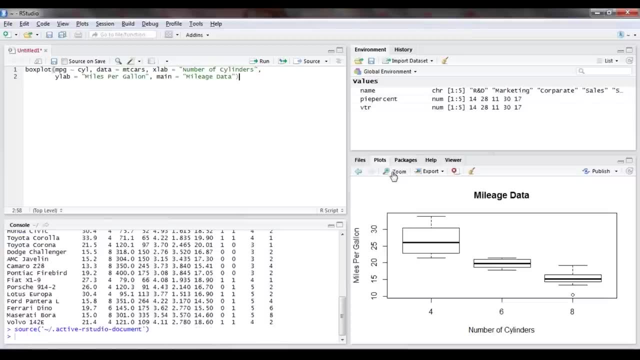 your X label it should be number of cylinders, your Y label should be miles per gallon and your main plot should be: with respect to mileage of data. if you run this, you can see the graph present here. let me just export it so you can see the data. now. let's say you want to give color here. then all you have to do 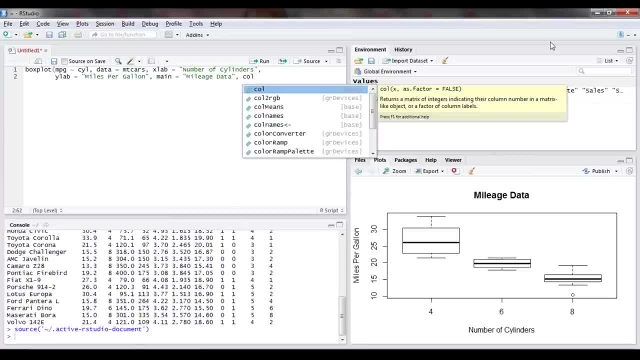 is put a comma, call, call is equal to the colors that you want to use. so you can see the colors that you want to use here. you can see the color that you want to pick. any three colors, okay, I have red. okay, yellow. something else okay, blue. okay, sure, okay. so these are the three. 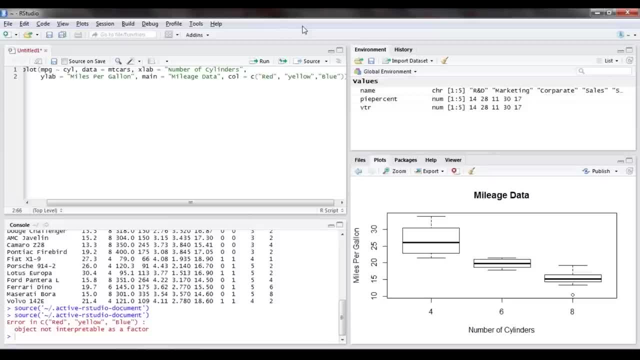 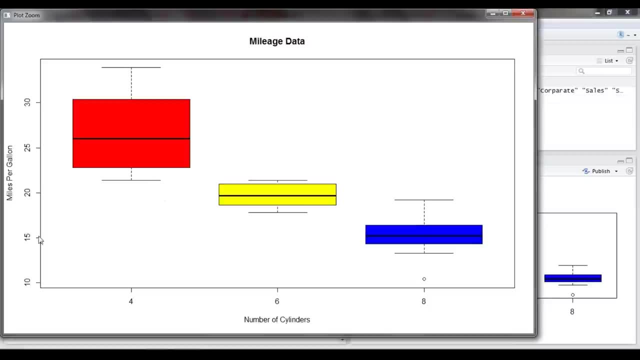 colors that I want as part of my bar plot. just close this. and now let's try rerunning this so you can see they've been colored as well. so if you just zoom on this, you can see the three different colors that they have taken up. so again, 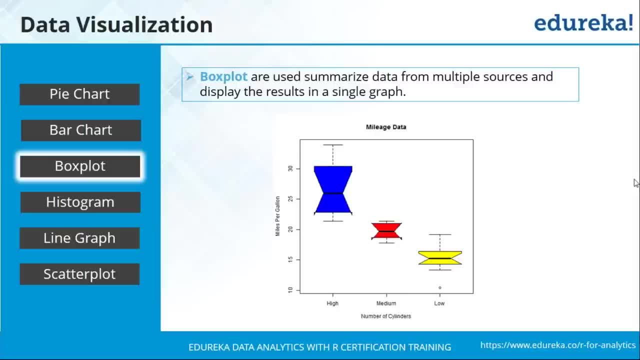 you don't need to worry how exactly it is working, because our next session is going to be on the colorization in our. okay, but I just wanted you to have an idea on what, not types, of graphs, you can plot in our, and how simple and easy it. 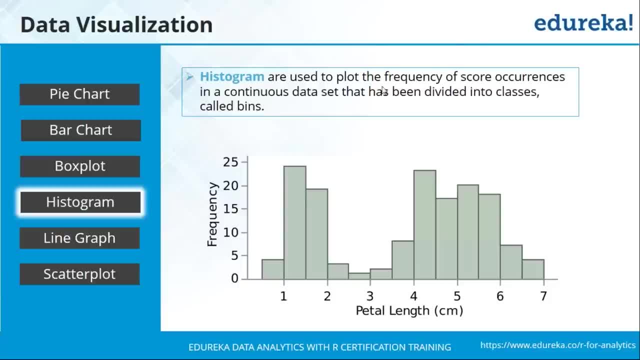 is now. the next type is histogram. now, histogram is one of the most easiest graphs that you can work with. histograms are basically used to plot frequencies of continuous data. so, again, this is one of the most common kind of graphs that you will be preparing as part of our, apart from scatter plots, so definitely. 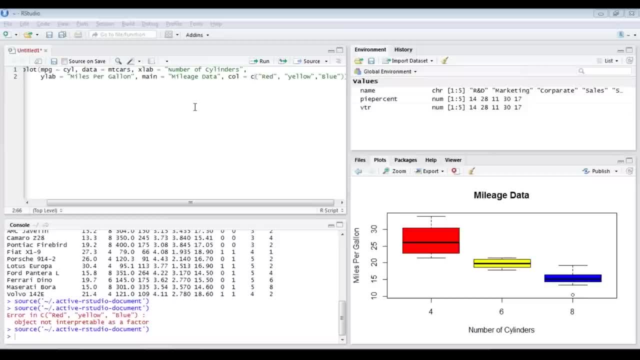 this is something that will. that is quite easy as well, so let me just show you how to do that. so in our R studio, let me just remove all this. let's say vector 1: okay, throw at me some random values, okay. so 9, 11, 25, 70, 3, 4, 5, 9, okay. 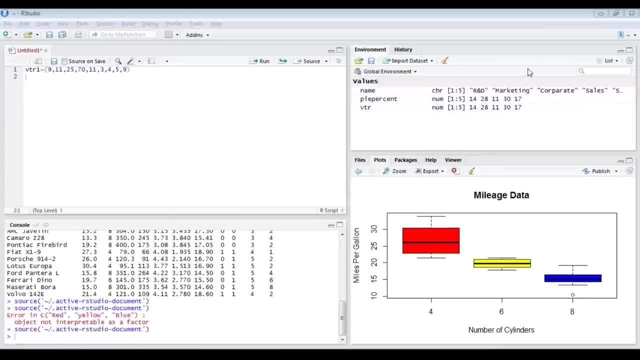 this is my source data and based on this, I'm going to create a histogram. so it's so to create a histogram, it's just hist. so I'm going to create a histogram. so I'm going to create a histogram. so it's so to create a histogram, it's just hist. 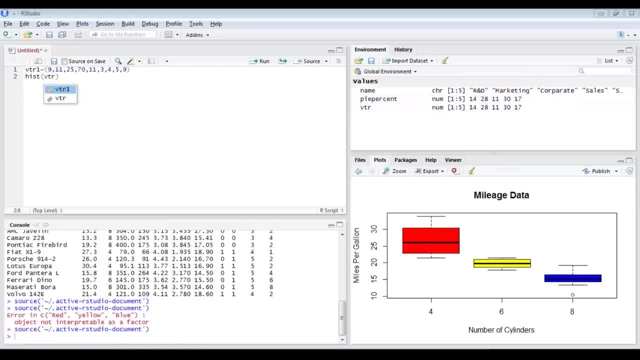 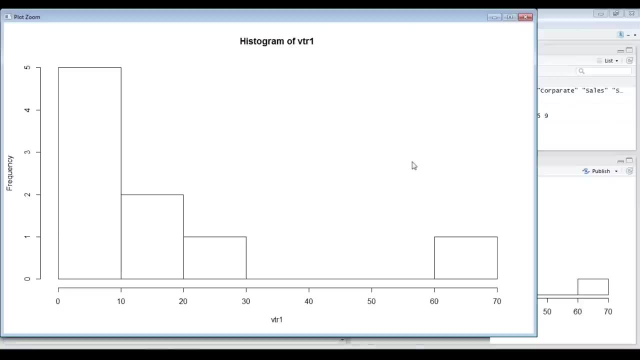 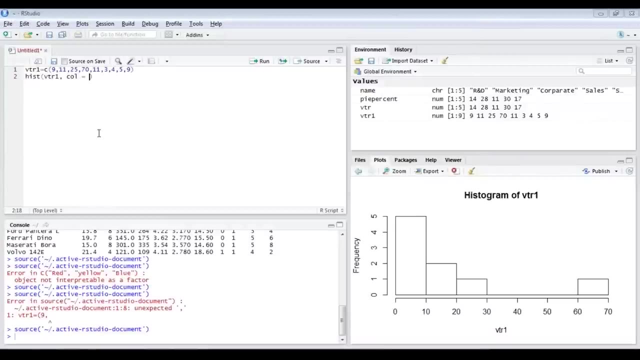 and then you just need to pass vector 1. now, if you run this code, then you can see the histogram here. now it feels a bit dull, so what I'm going to do is I'll just close this. let's say, col is equal to blue. again, it needs to be in quotes, and I'll 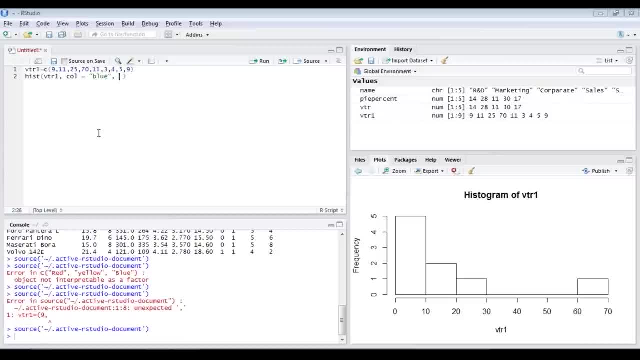 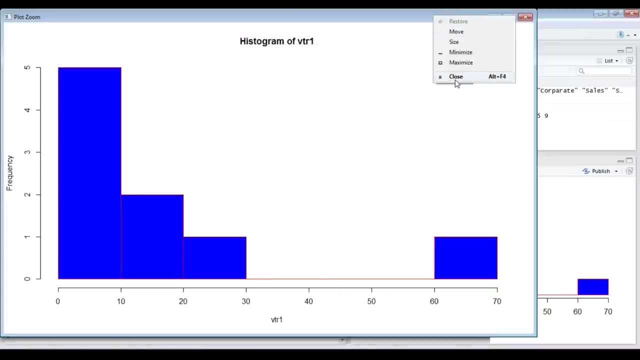 also give a border. let's say border is red. okay, if you just read on this. so your histograms got a little more color with respect to that same now, although there are certain inconsistencies, but this is because we've just taken a random data set again, so all it requires is just one. 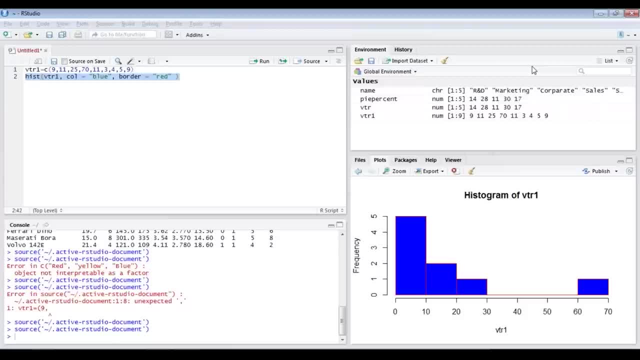 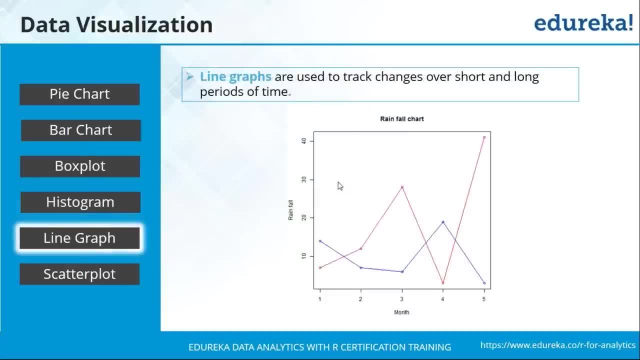 simple command for you to create a histogram, and it's quite easy with respect to that same. now, coming back to our presentation, the next and second last graph, or line graphs. now, line graphs are something that's quite interesting. you can always plot different kinds of line graphs. it could 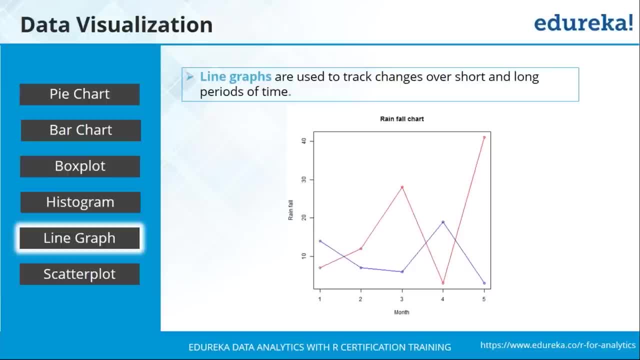 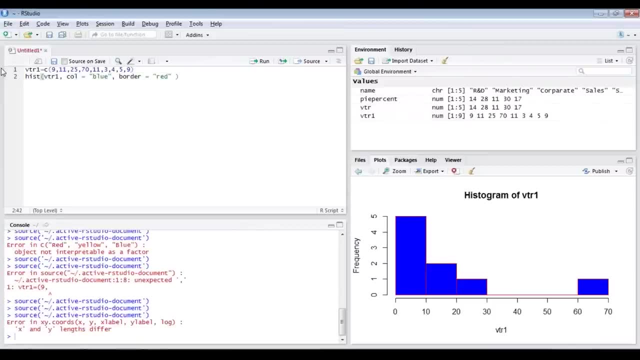 be single line, it could be multi line, it could be a single line, it could be two lines, it could be multi lines. so any number of lines, as long as you have the correct information. now let's go back here. so let's go ahead and modify the. 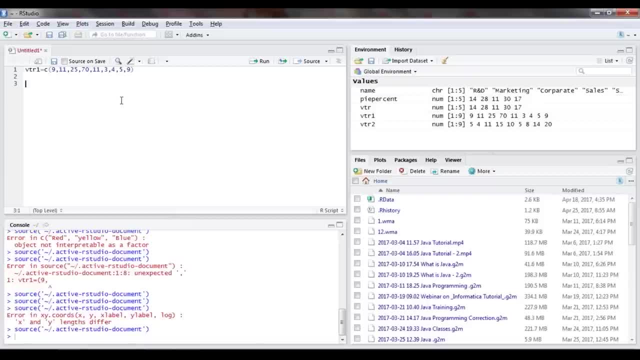 same part itself. so we'll just consider the same vector 1 and I'll just say plot. I just passed vector 1 comma. the type again. type takes a value P to either draw only points, I to draw only lines, and over to draw both points and lines. 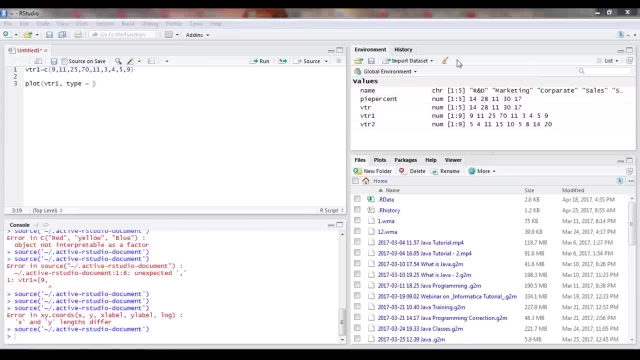 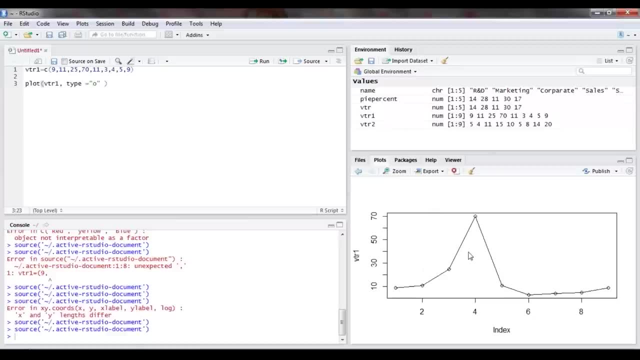 so, since want both, I'm going to pass the value of type to be O. Okay, now, if you just run this, you can see a line graph being plotted for the different values that we have passed. So it's again quite simple. and the final. 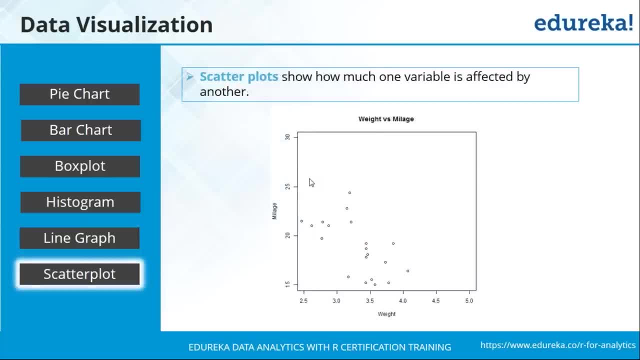 kind of graph that we'll be discussing is scatterplots. Scatterplots actually tell us how one variable is basically affected by another variable. So this could be with respect to two different criterias, itself The change in value of one, how badly does it affect the change in value for the other? So this is: 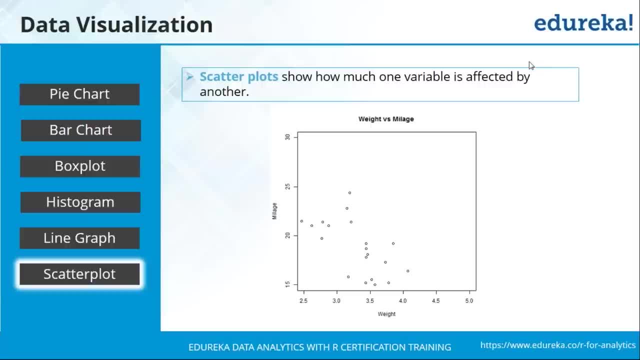 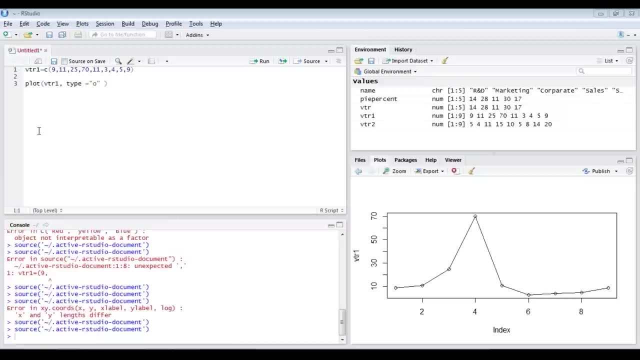 something that can definitely be understood using a scatterplot. So let's go back to our RStudio. So here all you need to do is, let's say you already have another vector, So I have vector 2 present here. So I'll say vector 1, vector 2 and instead of type O.